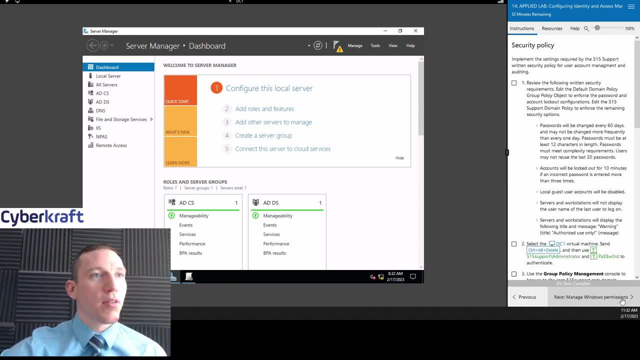 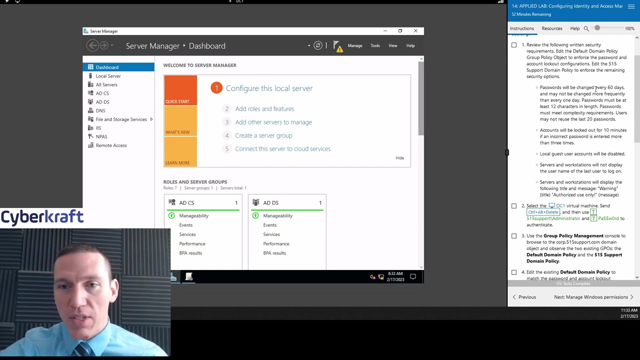 Okay, so it gives us the domain objectives where we that we're going to be looking at. All right, so let's see: implement security settings required by 515 support: written security policy for user management and auditing. So we have to review the following written security requirements: Basically, we're going to be implementing these, these changes, I think All right. passwords will be changed every 60 days and may not be changed more frequently than every one day. Passwords must be at least 12 characters in length. Passwords must be complexity required. 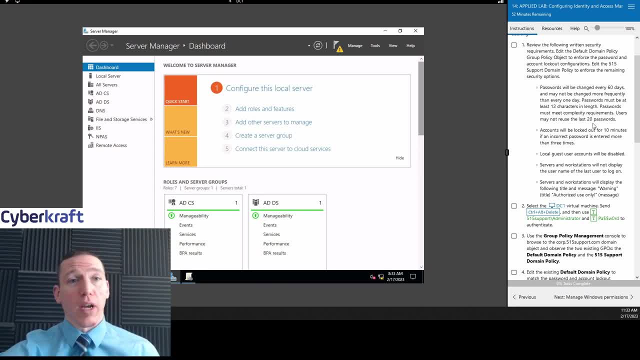 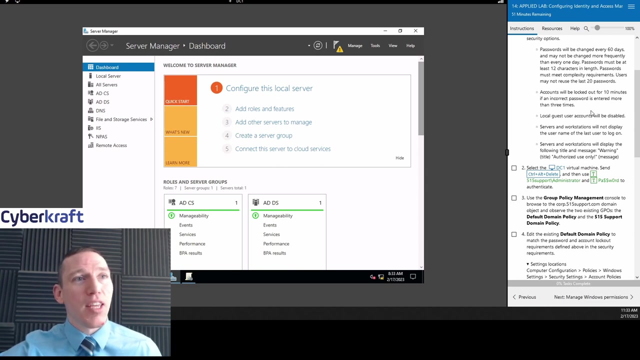 Users may not reuse the last 20 passwords. Okay, that's pretty strict. That's even stricter than what you'll see with the federal government Changing passwords 60 days. I don't think that's a good security practice, in my opinion. I think something a little more reasonable, like once a quarter, maybe once every six months, but 60 days, that's just. that's a pain in the butt. Anyway, counts will be locked out for 10 minutes if an incorrect password is entered more than three times. That's going to generate a lot of IT support tickets, especially if someone is using it. 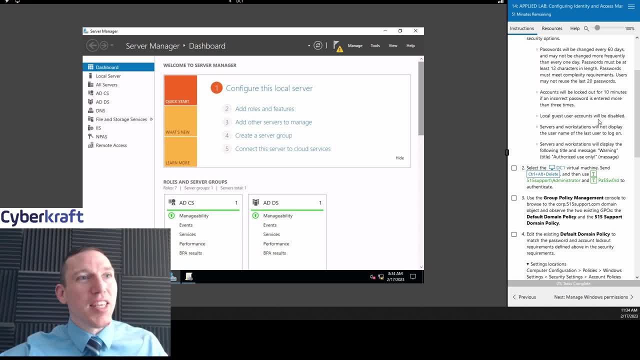 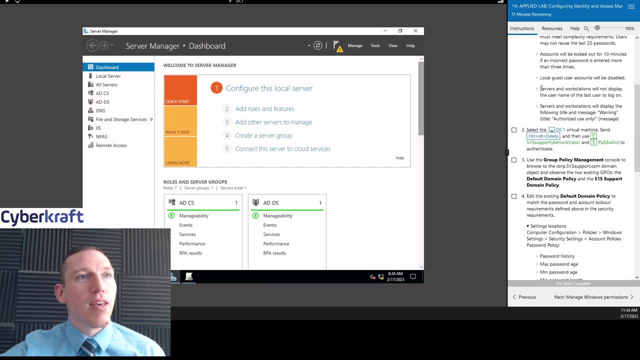 Someone's coming in early, you know fat finger in the keyboard or just you know not really paying attention. Local guest user counts will be disabled. Okay, servers and workstations will not display the username the last year to log on. That's a good security policy. Servers and workstations will display the following title message: warning- authorized use only. Okay, often you want to have some sort of security banner or message when you first log on to this to basically to cover: 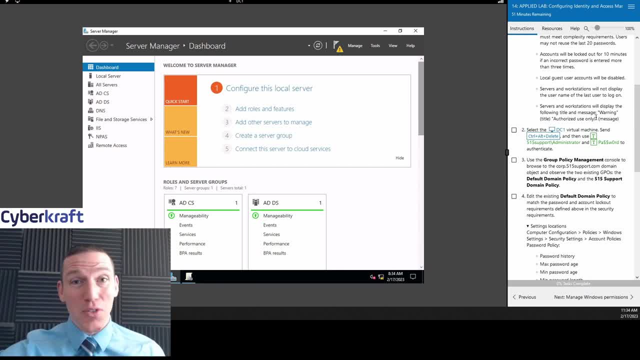 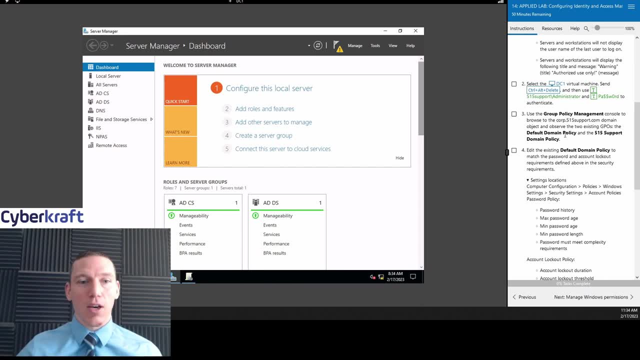 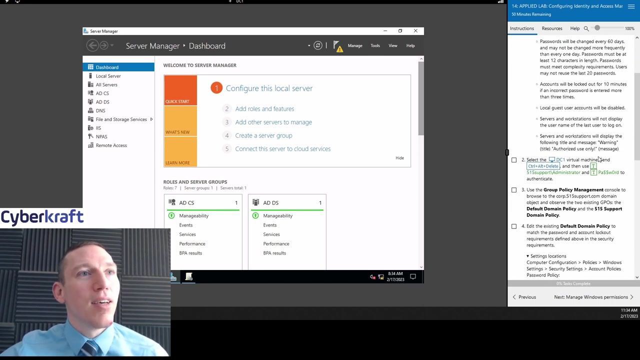 your butt to show, to show that you're telling your users that they need to follow the security policy. So users can't, you know, go do something on the computer and then later say, Oh well, I didn't know, we weren't supposed to do that, And you have a lawsuit on your hands, things like that. So this is usually the message, a little more involved, But that's. that's a pretty good setting. Everything here is pretty good, except for the 60 days nonsense. And I don't know about not reusing last 20 passwords. That's kind of annoying too. 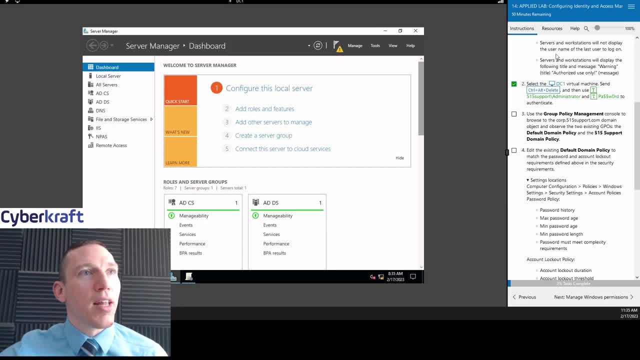 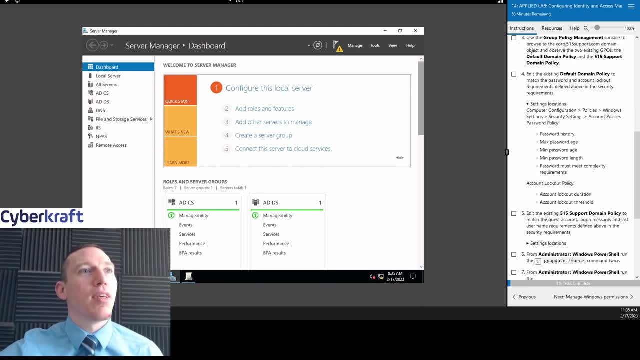 Okay, so we're gonna log on to DC one. I've already logged on to DC one. I like to log on to this stuff right away, as soon as I get into labs, because I don't like to interrupt the flow in between. Okay, now, obviously we're using okay group policy management, So you access this through your server dashboard tools, group policy management. Okay, And I have that open already. Now, here you're going to see in your domains. 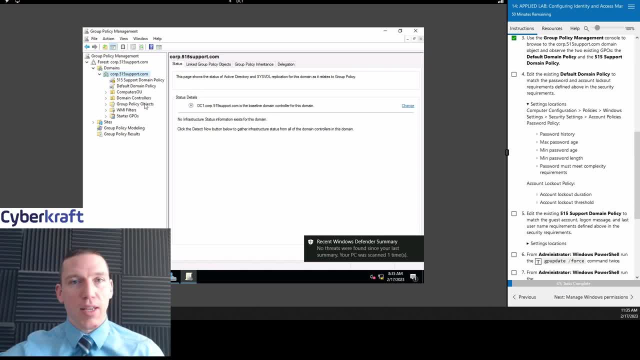 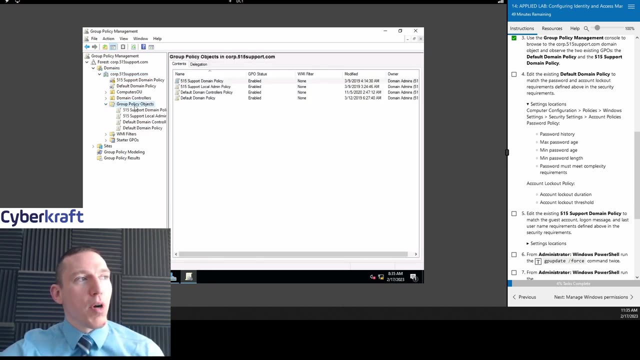 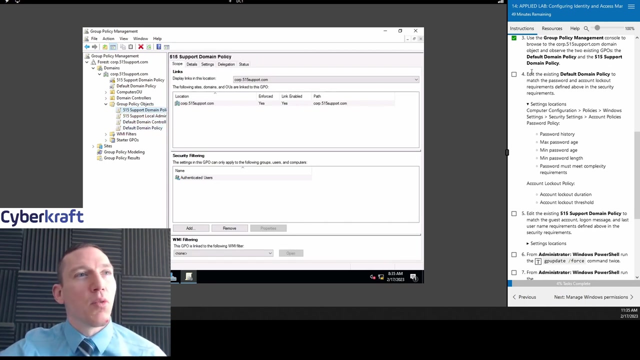 corp.515supportcom. that's the domain that we have designed for the labs. So if we're going to be doing, oh they have shortcuts here, they have shortcuts for what we need, But we can. we can look down here at group policy objects to find these, these objects that we need. So let's take a look here. Which one do they want us to configure first? Sorry, default domain policy. Okay, so we have to look at group policy. 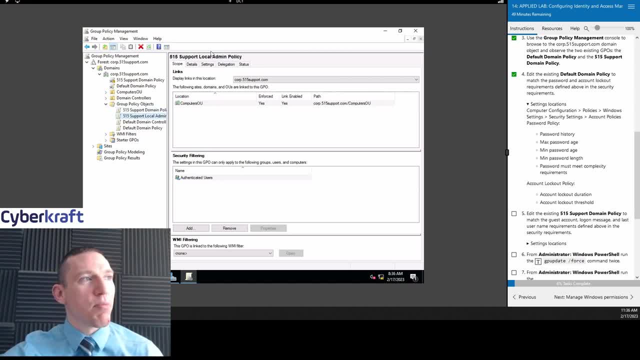 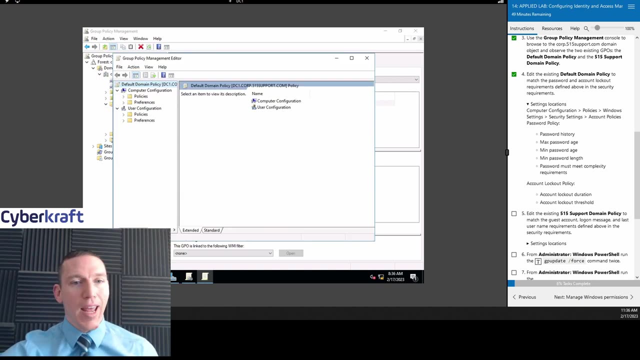 look at the default domain policy. we have this 515 support domain policy, the local admin policy, default domain controllers policy and then default domain policy. so we can just right click on this and hit edit. okay, we could also go to action- edit, those are the same things. so let's go ahead and 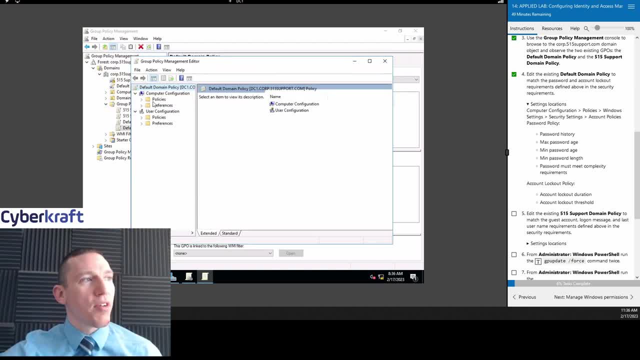 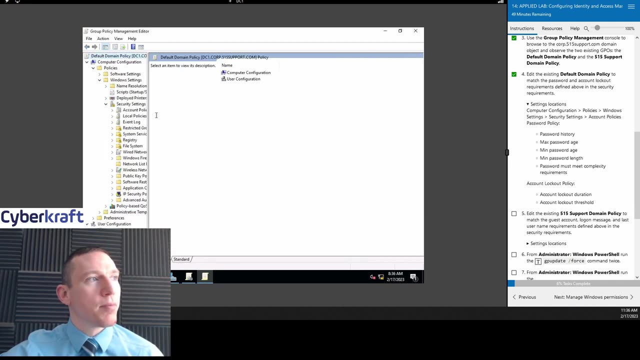 edit that one. all right, in here we're going to find uh down here under policies. this is where we're gonna go ahead and set this up. we go to policies should be windows settings and then security settings. okay, let me expand this out: security settings and then we should see. 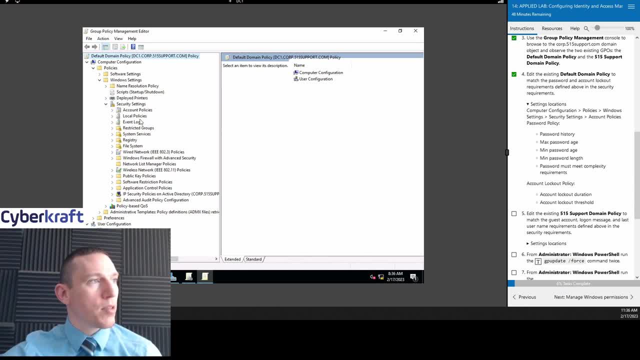 password settings here. um, i think there's one more. i have to do: account policies, right count policies and then password policy. okay, so here we go. password policy: let's take a look at what we have here. history, so we could change this. remember they wanted 20 passwords, remember so? we'll apply that. it's gonna take a moment. they want 20 passwords. can't reuse the past 20 passwords. has to be 12 characters in length, so we're just gonna go ahead and adjust these settings here. okay, minute for minimum password age or maximum password age. we're gonna change that. right-click properties change that. 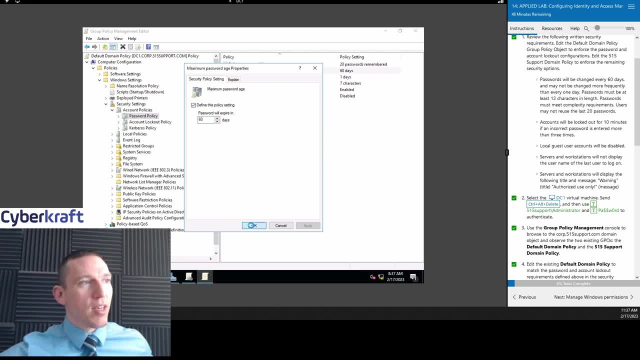 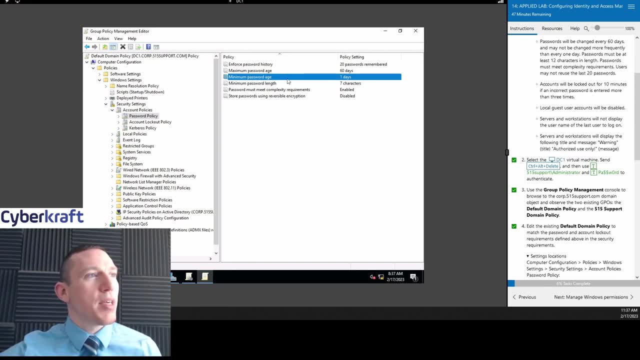 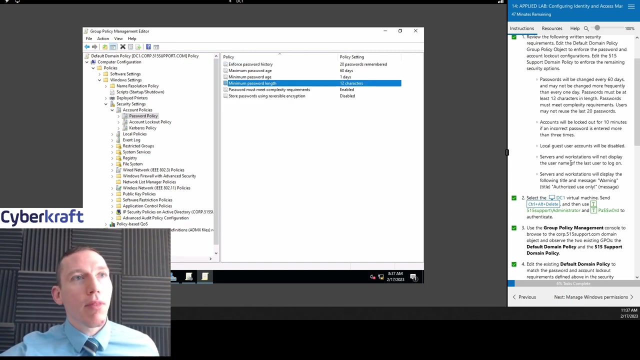 to 60 and it looks like someone clearly just went in here and adjusted these, you know, to be random values. I have to be 12 characters length. right now it's at 7. let's up that to 12, okay, and modifying these in GPO is a really easy way to do it. I think it's probably the 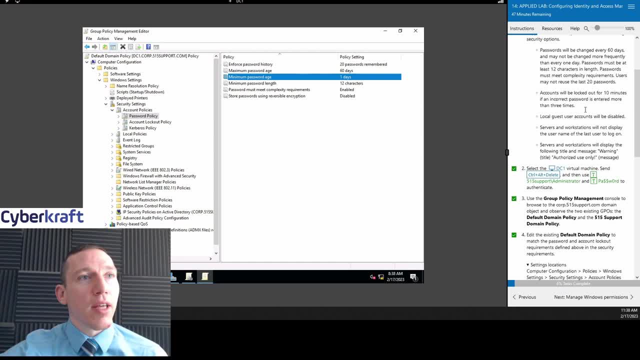 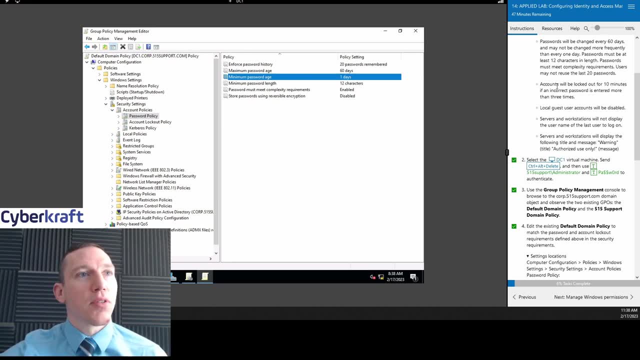 most efficient way. so I think this is a good system. minimum password age is one day. I think we that's correct. passwords where did say that may not be changed more frequently than one day? okay, that's minimum password age, right, so that's good. it prevents users from constantly changing their password. must meet. 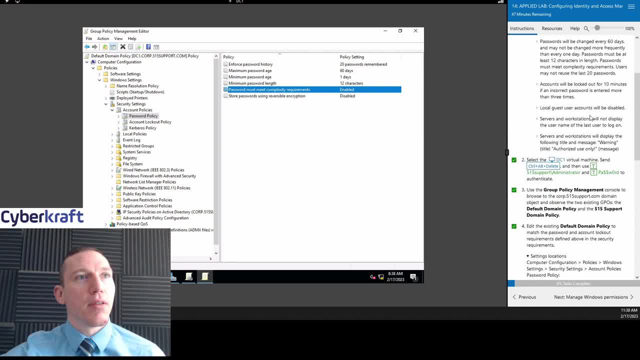 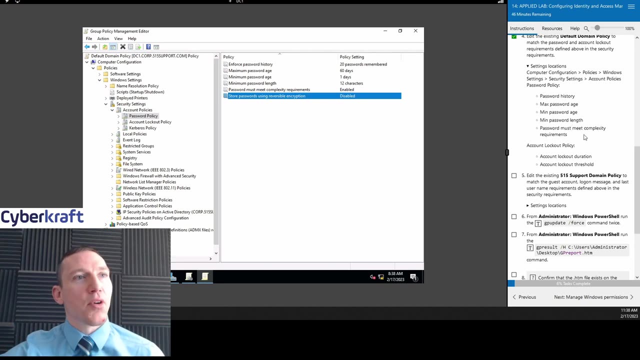 complexity requirements. it doesn't say anything about that, but that's fine. store passwords using reversible encryption. the same thing about encryption. no, okay, pretty good, let's see. it does ask us for complexity requirements here, so we've done everything there. now we want to do account lockout policy. okay, and for that. 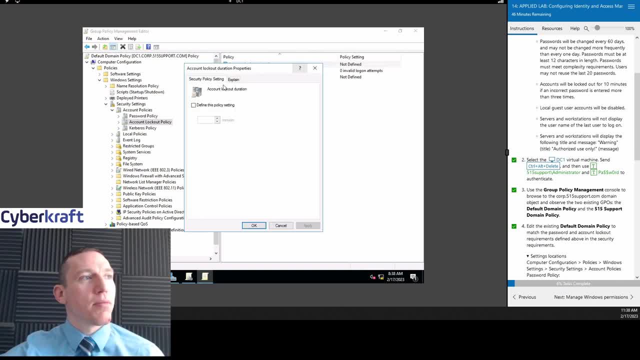 one. they have to be locked out for 10 minutes. so you know I've been right-clicking, deploying or doing properties. you can also just double click it, so we're gonna hit. you have to check the fine if something is not defined. you have to check this to be able to modify the value. just keep that. 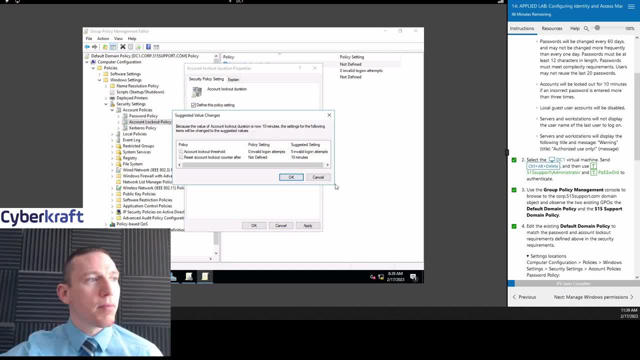 in mind. this can be a 10-minute lockout, and then we're gonna have to change those. yeah, it's. it's telling us: okay, if you're gonna put a lockout, you need to. you should adjust the conditions for when the lockout triggers. so I think it's. at three lockout attempts, which is a little strict. I think five is more reasonable. reset account lockout counter after 10 minutes. yeah, that's that should be fine. that should that can often match the duration and let's see that should be good. all right, we adjusted those, so all those are pretty good. 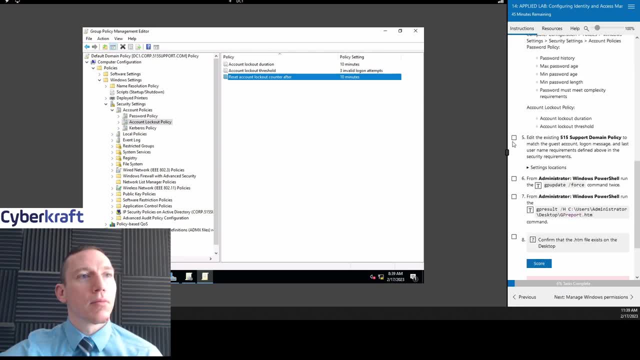 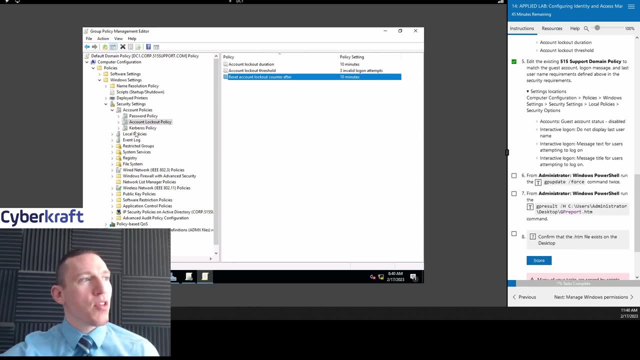 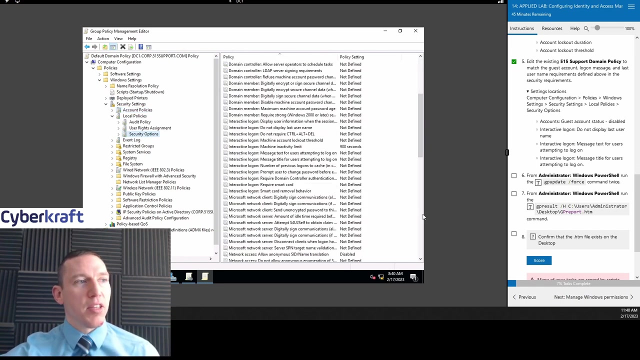 okay, now for the rest of these, we're gonna have to go to a different setting. or if you go to window settings, security settings, and we have to go to security options, right, local policies, local policies and security options. okay, now here's where you'll find a lot of these miscellaneous settings that we're gonna 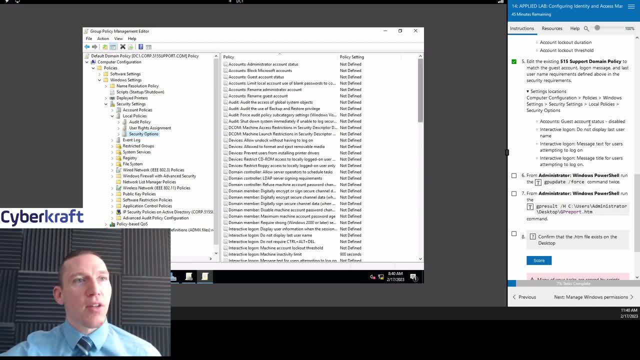 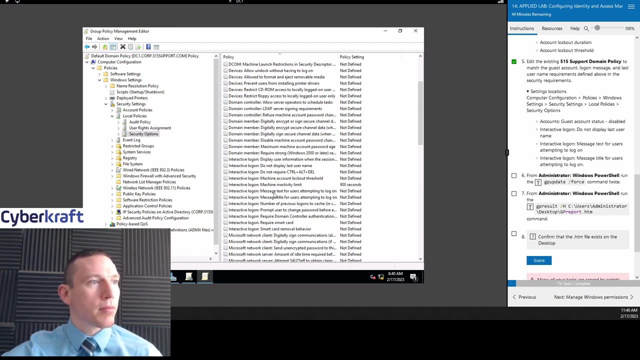 be looking for. so a lot of these are gonna be in counts accounts. guest account status: disabled interactive logon. that's gonna help us display that message. it's also going to help us not display the last name. display user information. no, no, do not display last username. 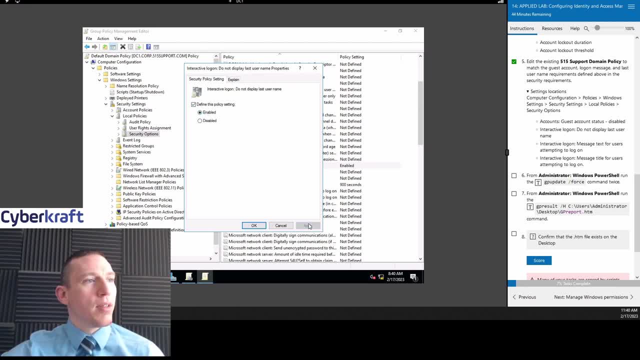 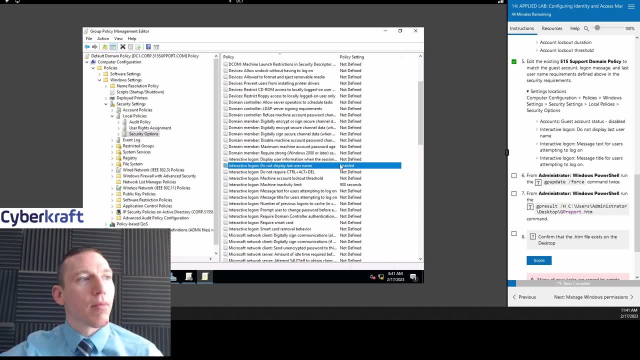 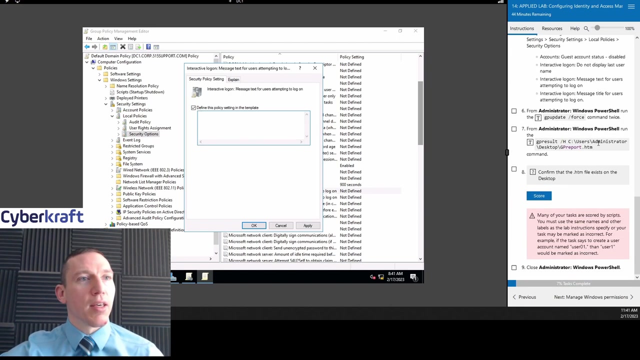 enabled. this one's a little tricky because it's it can be a double negative. do not display last username. let's see interactive message text for users attempting long on yep. and this is where we can. we'll just copy and paste. oh yeah, I don't think I can. 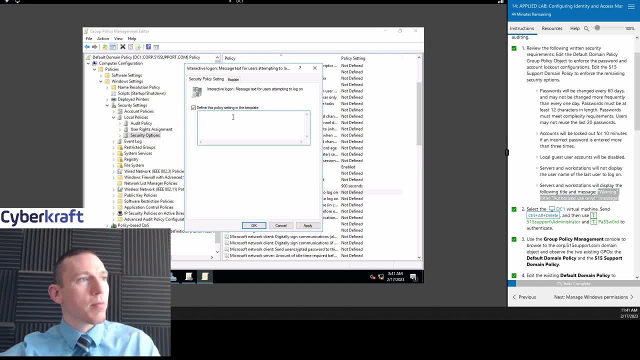 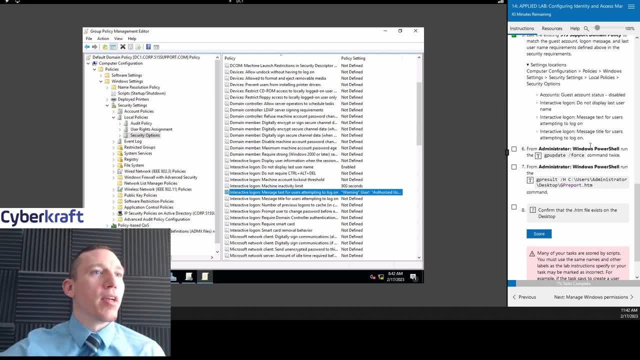 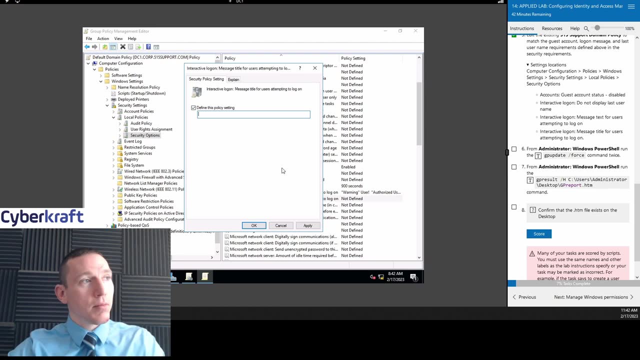 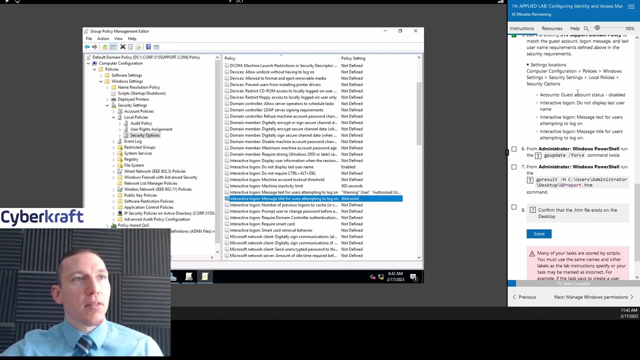 Did that. that's pretty good. And what else are we doing here? Message title for users attempting to log on. All right, so that's where we're finding all those settings. Should be good to go there. Now we're going to be. 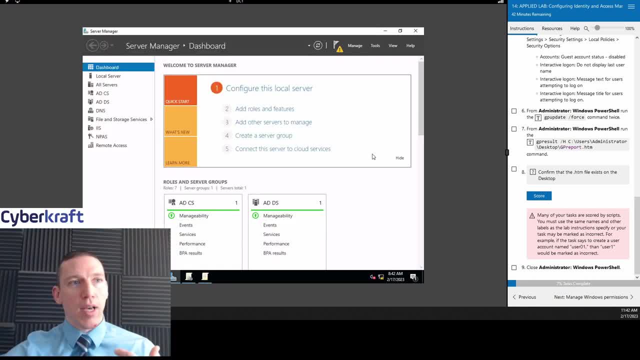 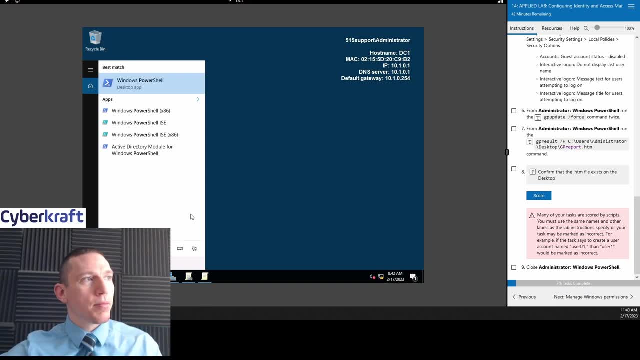 Once we've done that, we've applied all those. Now we have to update our group policy settings, Okay. so an easy way to do that is to open up PowerShell. Just search for PowerShell, Right click on PowerShell, run as administrator. 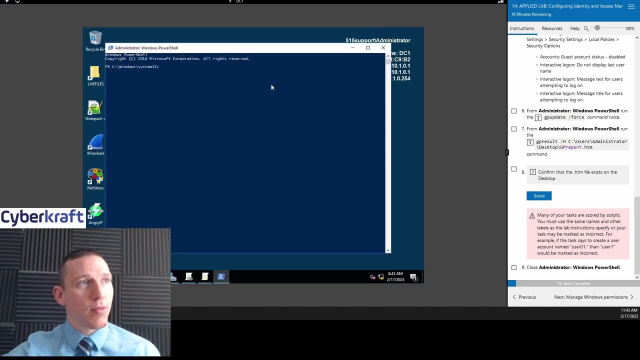 You always want to run it as administrator, Just as a good rule of thumb if you're making administrative changes, because it's going to help you bypass any permission problems. And then GP update- group policy update- This is the command that you want to use. 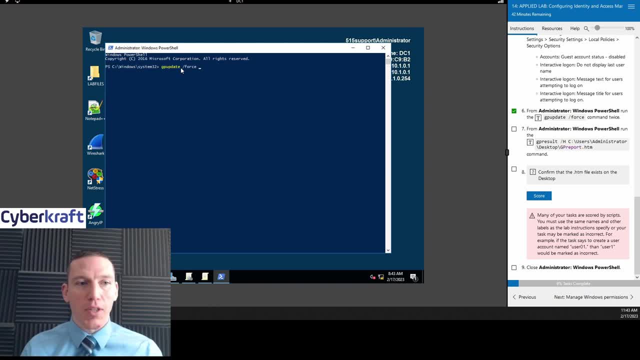 And if you're using group policy, if you're making a lot of changes with group policy editor, this is a great command to keep in your toolbox. So GP update slash force lets you update the policy. Lab tells us to run that command twice just to make sure it goes through. 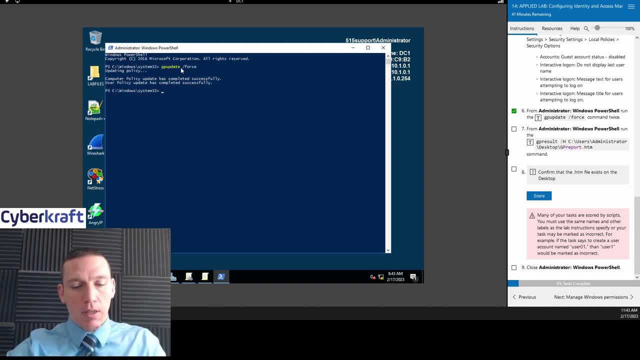 Says it's completed successfully. Let's just run it again just to be sure. Okay, Okay, Okay, Okay, Okay. Now again, I always invite you to type out the commands. gives you believe it or not? just the act of typing it gives you that extra muscle memory. 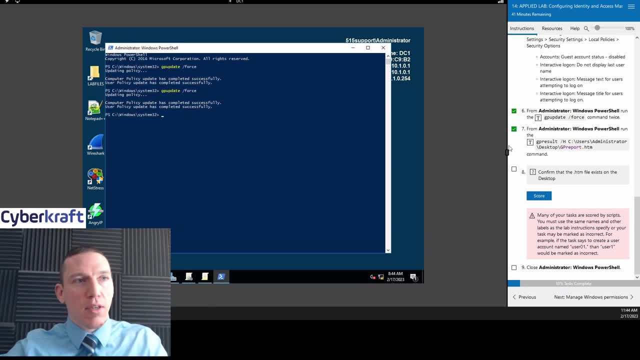 So it really does help. I know you have the quick options here, but I do invite you to type them out. Now we're going to show the results. Okay, Make sure to spell correctly: Razzults. All right, GP result as result. 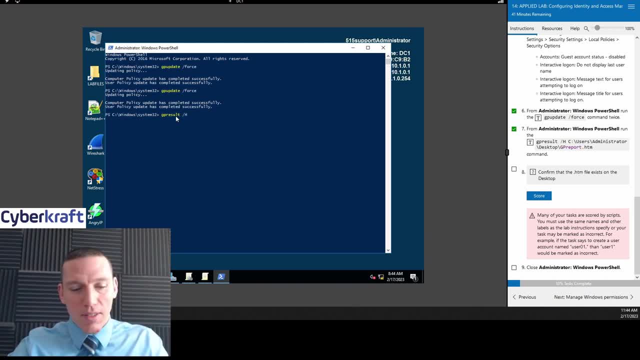 singular slash h. so we're going to designate the location and basically what we're going to be doing is we're going to be exporting our results- here you know, in a file that we can be reading, so like a reference file, instead of digging through all the group policy updates manually. 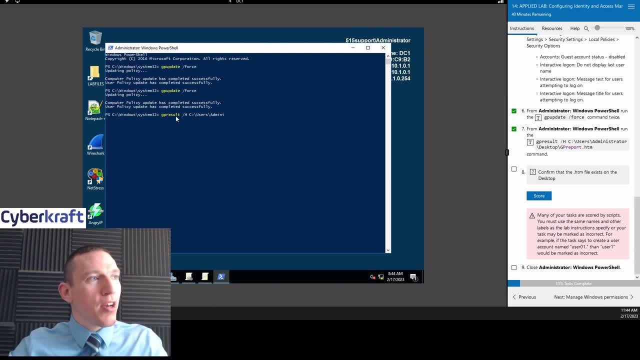 we can just output this to a file and then look at that file, understand what we talked about or what we configured. all right, see users administrator slash desktop. make sure to make this case sensitive and then we're new GP report dot HTM. okay, if it says generate report, we should see. 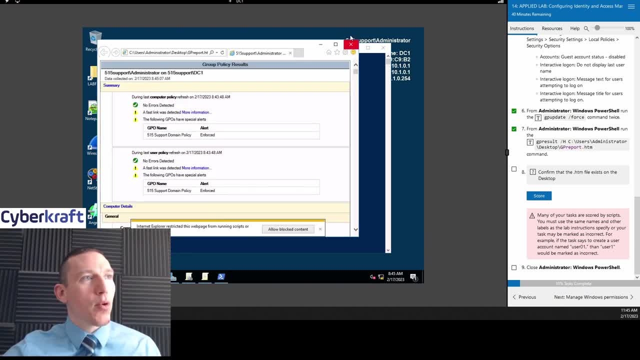 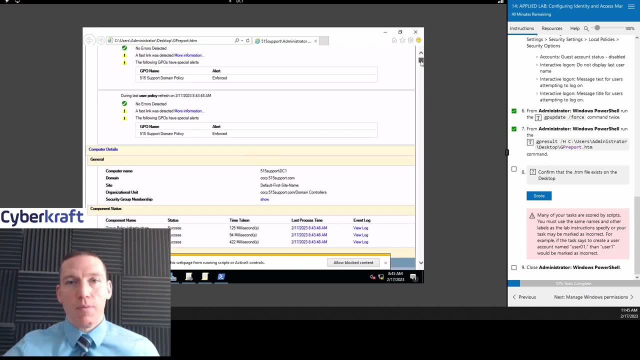 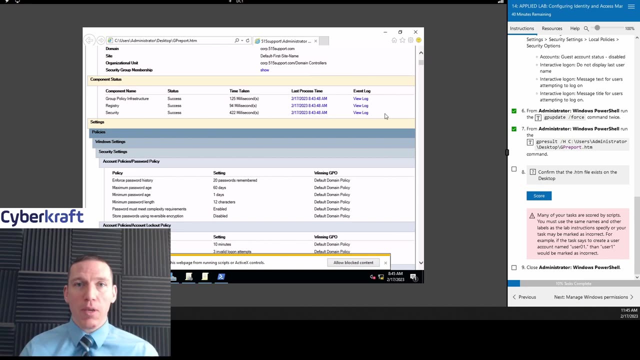 a report pop up on the desktop and we can open that report and here what we can see are all the you different changes we made to our group policy editor makes into a web viewable file. so if you want, if you you have a remote workforce, remote admins, you can, when you ever you make group policy. 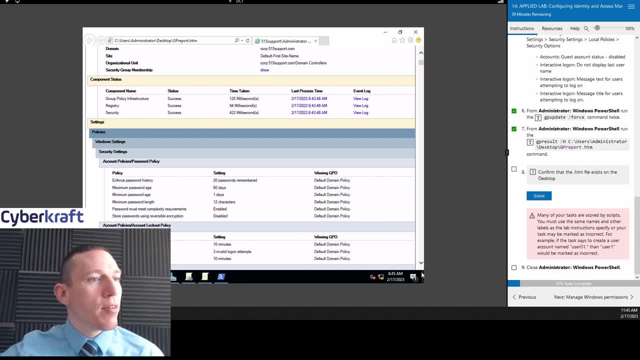 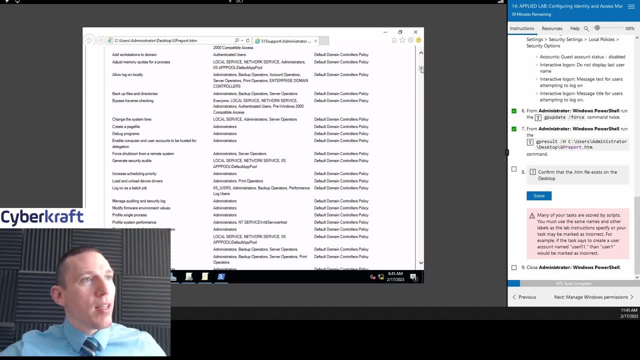 updates. you can publish this to like them your intranet and then share that with other admins- show you know what changes were made that day. it'd be pretty helpful if you have some sort of change management process. usually this will be automated. you'll have some sort of automation. 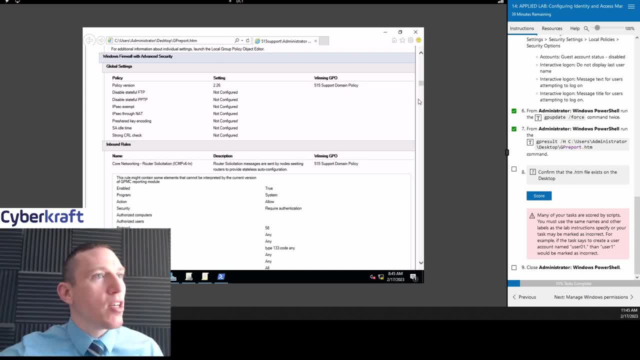 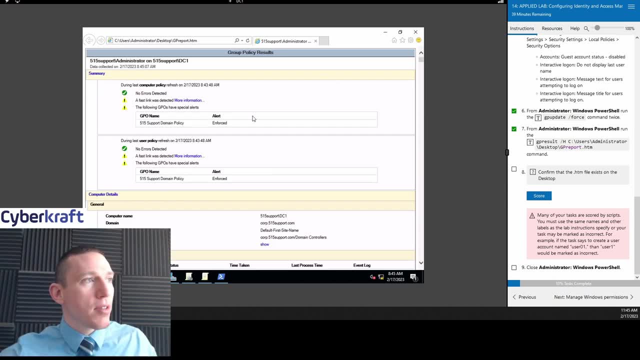 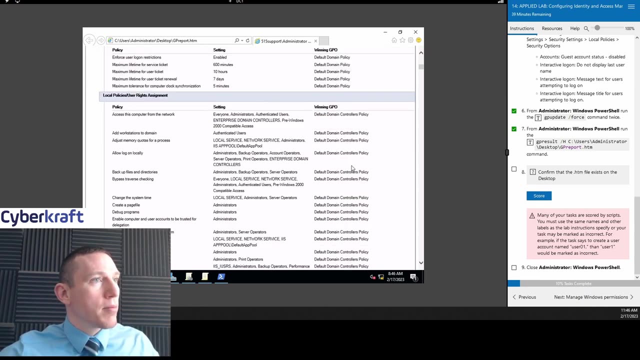 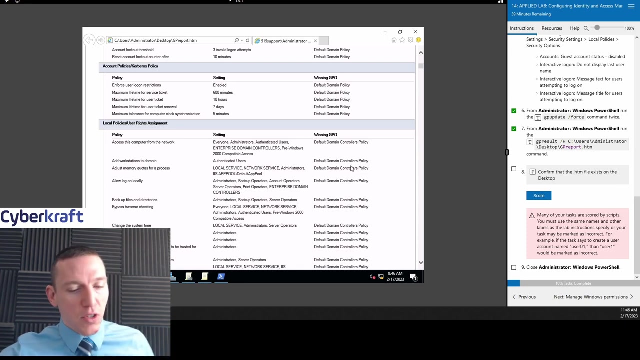 that will publish this so that everybody's on the same page and they know what changes were made. okay, so we can see some of changes if we go through this. we don't need to go through everything here, but let's see. yeah, we can just do a quick search too, and you can search the document so we can find. password related stuff. and that a little bit of information for the third of the first five pages there and let's go back to our dslr Mercantile clusters. i so we're going across two. we can just do a quick search through and you can search the document so we could find password related. security information me. there's some actual multiple zip code domain so it kind of works really well to the other side of it. so if you ever want, you're going to go over to the insert档 box, want a window where word retainer link for every configuration and together log in and and the AS Turk a link for you. so i'm just going to go over a mini search page and 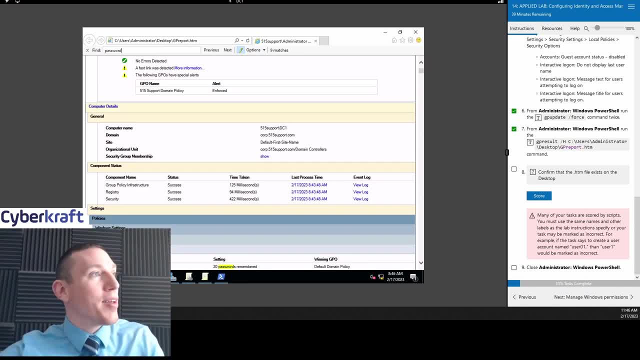 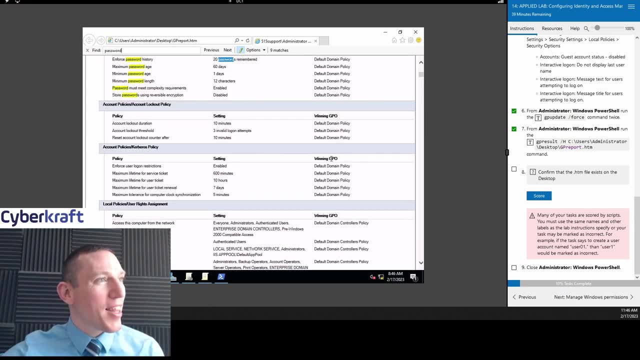 settings if i spell password correctly. i'm pretty bad at typing things so that they're spelled correctly, so if you have trouble with that, i sympathize with you. that's just. that's me too. and here's here's some of the changes we made: 20 passwords remembered, 60 day age, 12 characters. so 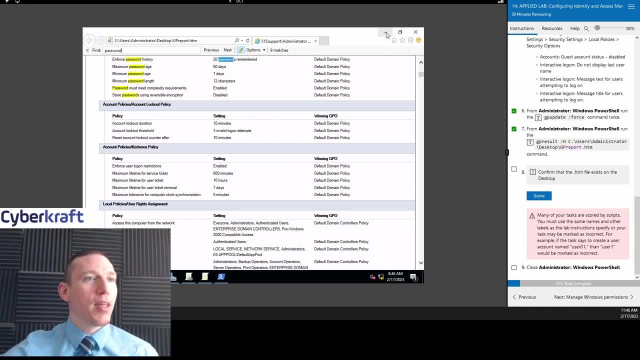 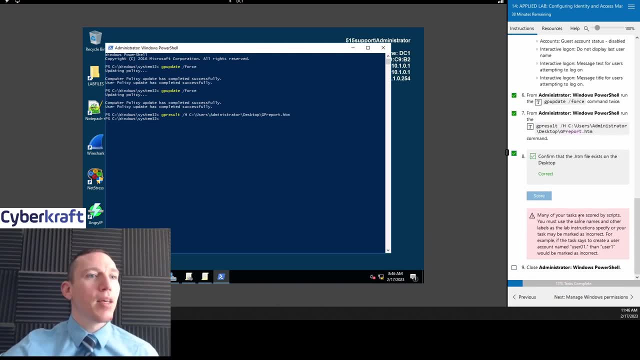 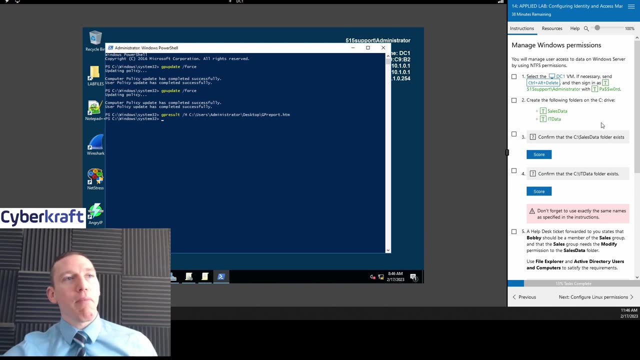 we see that those policy updates were published successfully. now the lab is just going to check that that file exists on the desktop, and clearly it does. we can see it, so that's great, all right. everything looks really good, all right. so now we're going to manage windows permissions using ntfs, new technology file system. 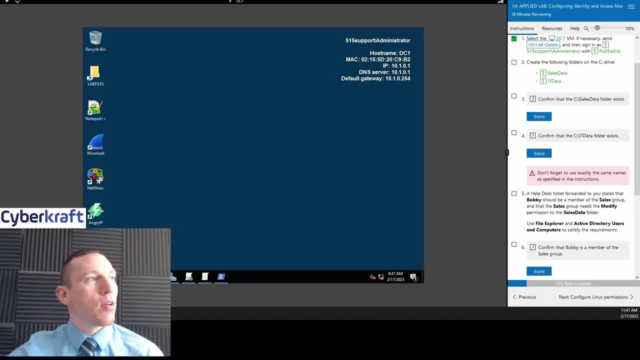 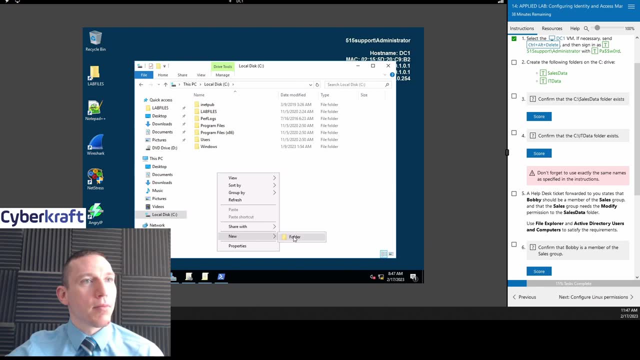 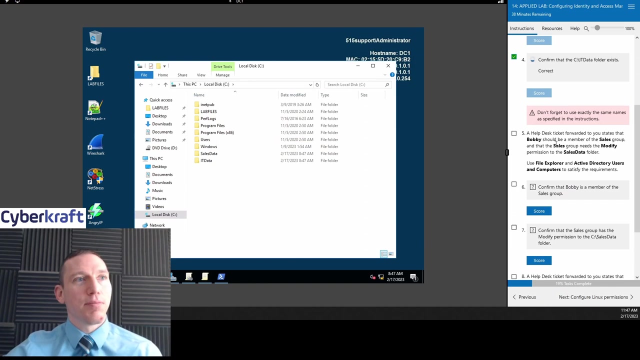 all right. so we've already logged on. we're going to create two files in the c drive. so i'm going to create one called sales data and i'm just right clicking new folder, okay, and then it data, okay. so we have two folders there. they exist, we see them. some of these are a little silly, these scripts, i gotta say. 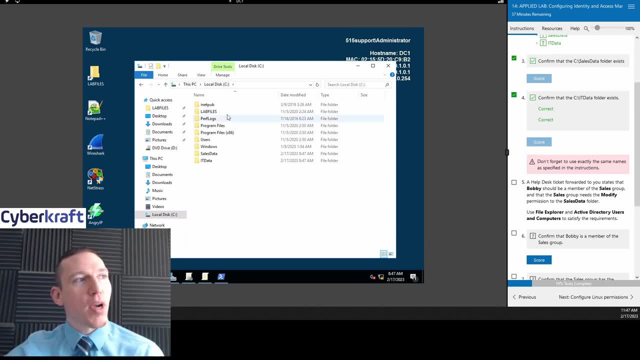 but it's designed to keep you on the right track, because if you don't put in the right spot, maybe you put in lab files. the other scripts aren't going to work, so they all build on the same thing. so we're going to create a new folder and we're going to create a new. 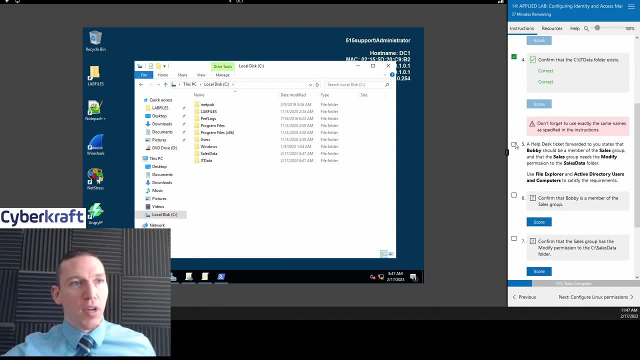 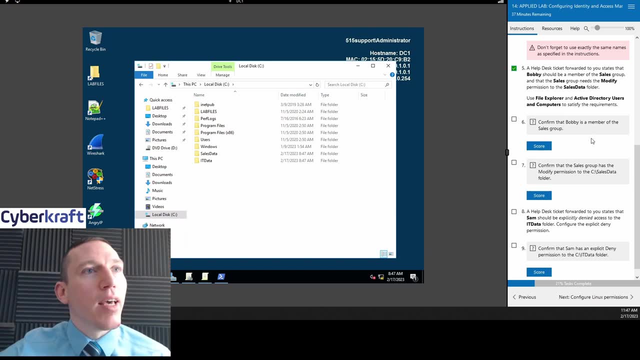 file one another. so it does pay to score them, even if they seem pretty silly, because they just help you. it's another check to make sure you're doing the right thing. so that's it helps, okay, help. desk ticket 40 to you to you states that bobby should be a member of the sales group. 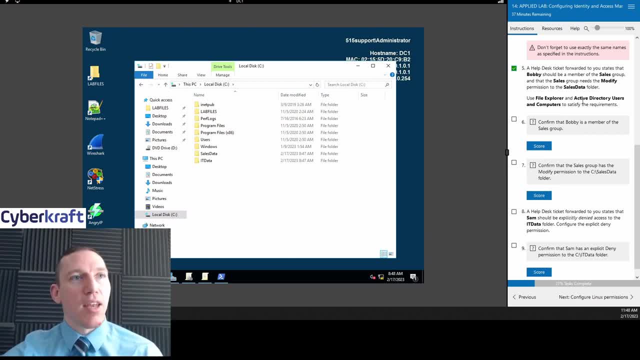 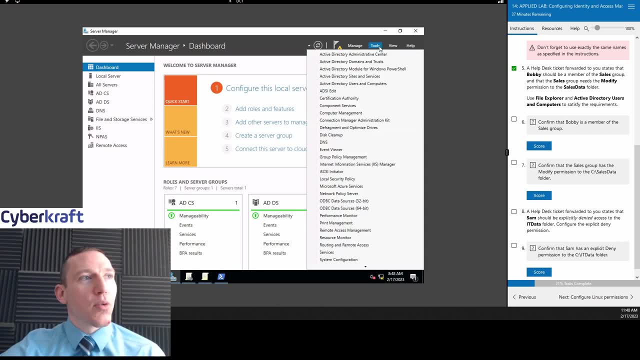 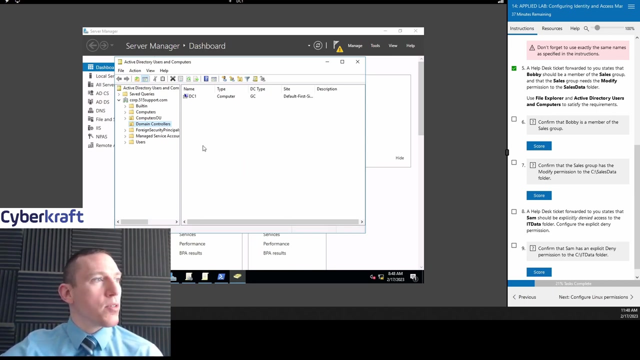 and the sales group needs to the modify permission to the sales data folder. okay, so we're going to go to server manager, active directory tools, active directory users and computers- okay, and then let's see, we're going to go to see users. let's go to Bobby Bobby. 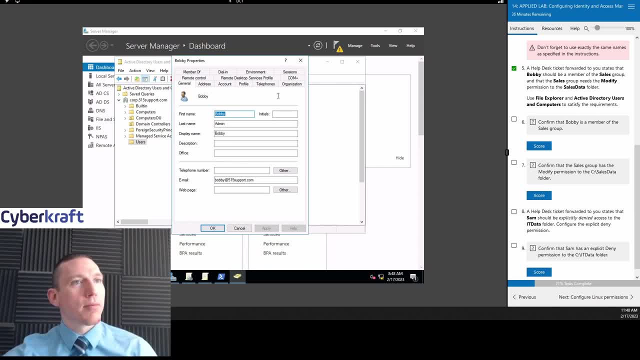 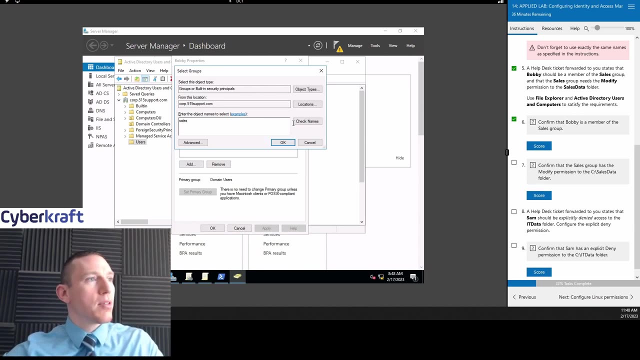 Bobby at 515 supportcom, member of 515 support users and local admin. so is he now he's not a member of the sales group, so we can add, so we can do sales check names. so basically what I'm doing here. okay, we see that Bobby's not a member of the sales group. there should be a group. 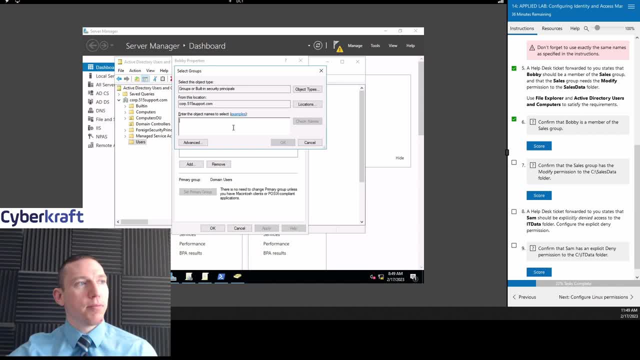 called sales. so I'm gonna hit add here under member of you go to sales. okay, I'm clicking sales and then I click check names. when I click check names, that sales group pops up. you can tell it pops up because it's under sales group. underline now, okay, so we've searched for a group called sales. I could search. 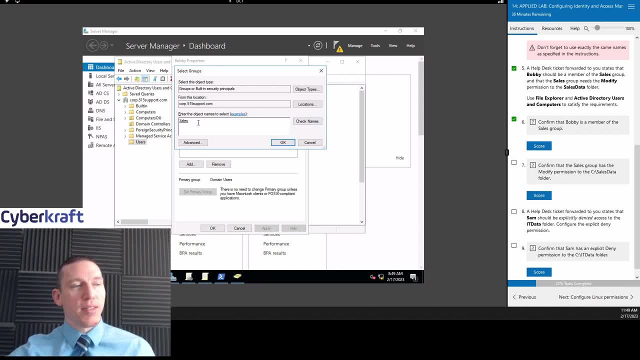 for something like sal okay, and I could check names and sales group would pop up, so it's recognizing the character string that put in there to identify an existing group and then, once it recognizes that that's the group I'm looking for, it'll put it in to the object. so I'm gonna hit OK, now and now. 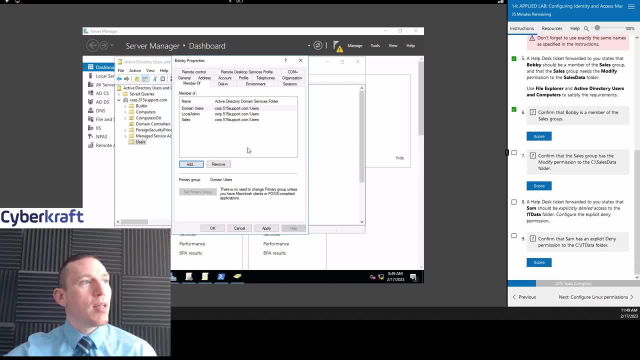 Bobby's a member of the sales group. okay, now we could do this a different way. we can modify the sales group and we're going to do next. I just want to show you how to do it from the user side, so we can do that from the user side. okay, so now we got to go to the sales group. here the groups. 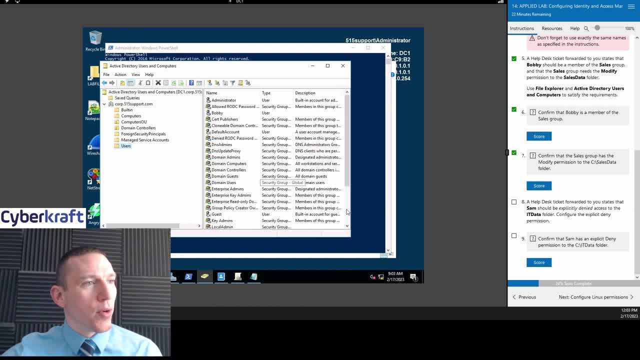 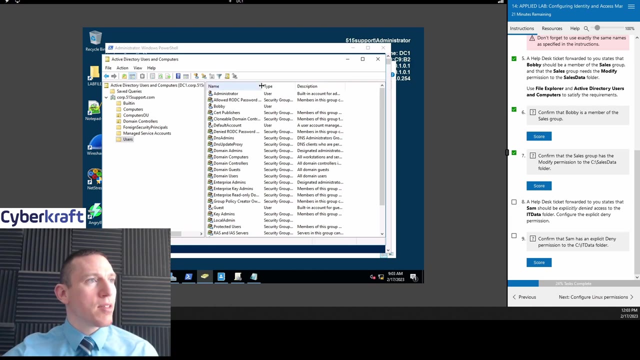 here are all listed in our users folder. okay, a lot of times you'll find the security groups just right off the domain corpse of 515, support calm. so I just made a test group. it appears here, but here there in the users folder it's. it's up to you how you want to organize these, but this is. you know I could see. 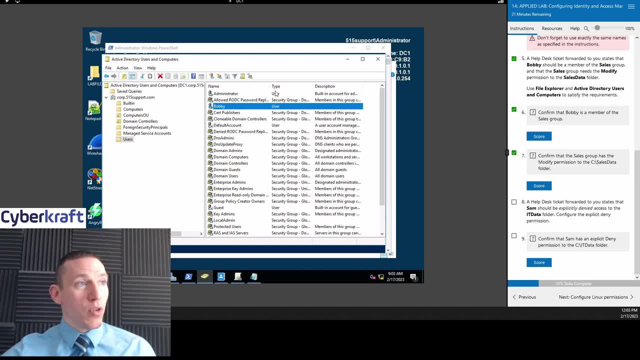 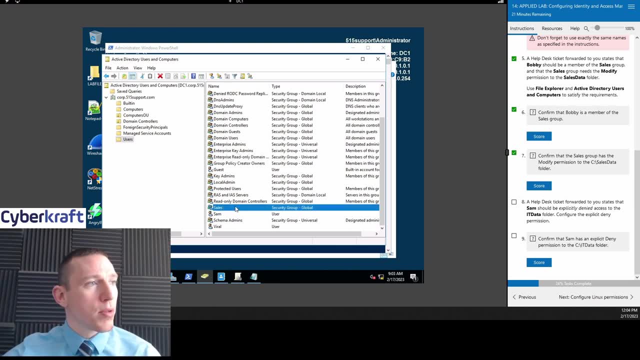 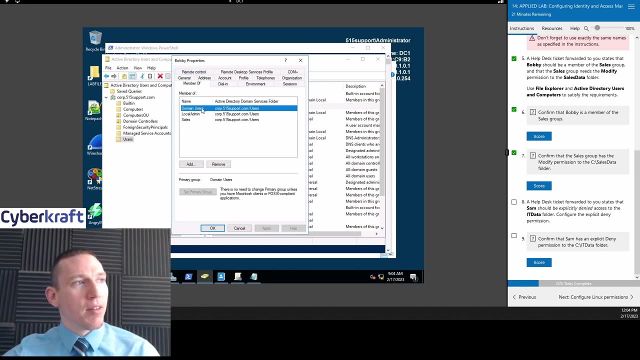 this, given some people some trouble. so here we have users. normally you see users here, but here we see security groups also. so this is where we see our sales group, and we saw that Bobby was a member of the sales, the local admin, admin and the- the main users. okay, so what we're gonna do here is we're going to double click. 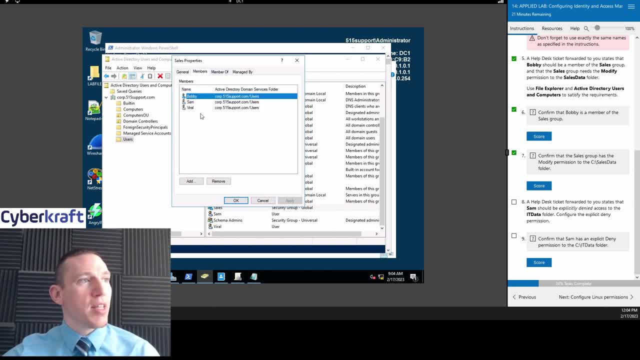 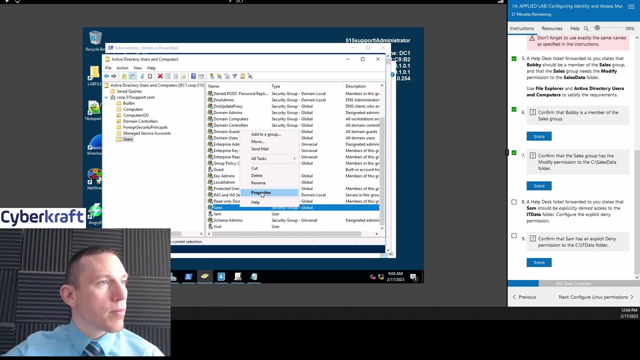 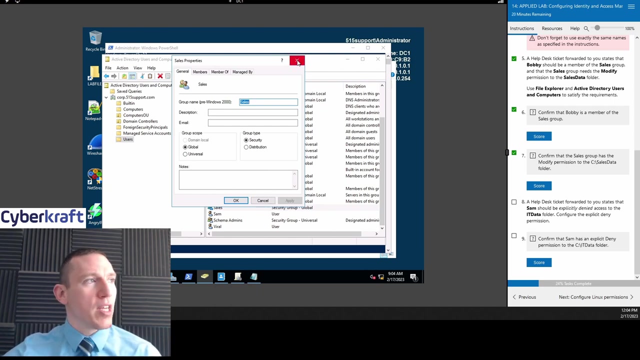 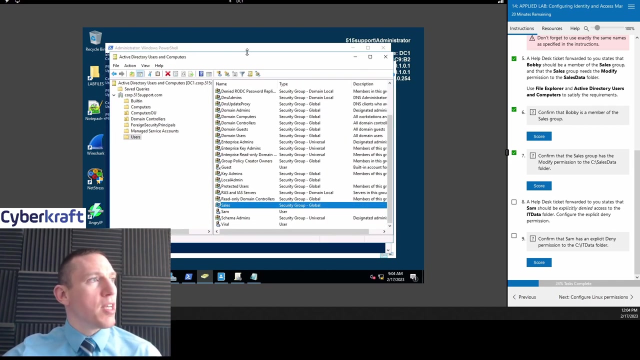 this sales group or to modify this. we see these members, okay, and then we have that managed by. we set this to a one click and we need to make the sales group have modifyee permissions of sales data folder. we can do that- the folder level. so let's go ahead and do that. but if 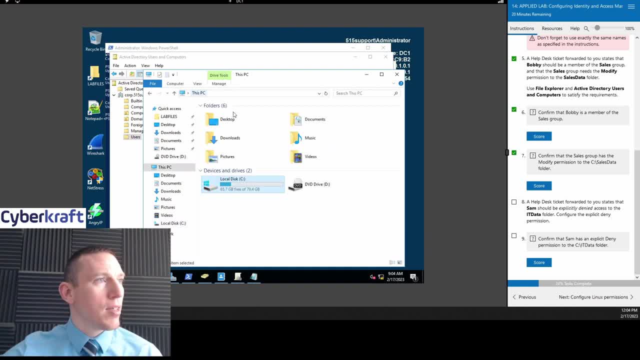 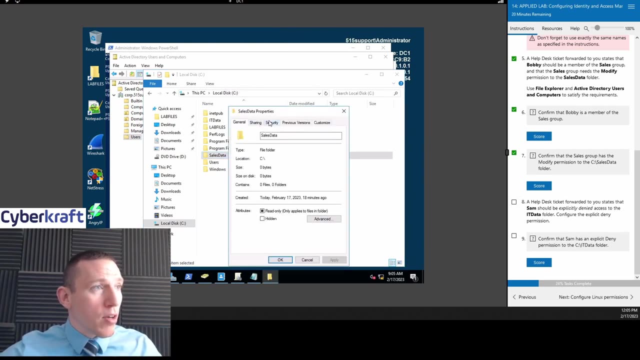 your confused as on why the group was here. you know, it's just just the just in this lab environment. that's how it's set up. so if that's confusing to you, that's okay. don't worry about that, that's so. we're gonna go ahead and right click here: properties, go to security, okay, and 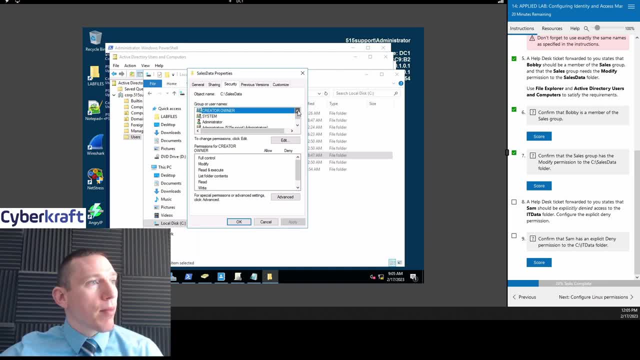 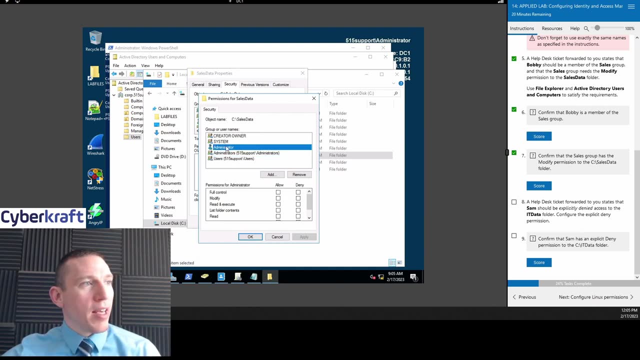 then from here, group or usernames, we can edit this. okay, we can add a administrator here or an owner. let's see the sales group has the modify permission. we can add one type: sales check names, sales okay, or hit OK there and now we have sales 515 support. 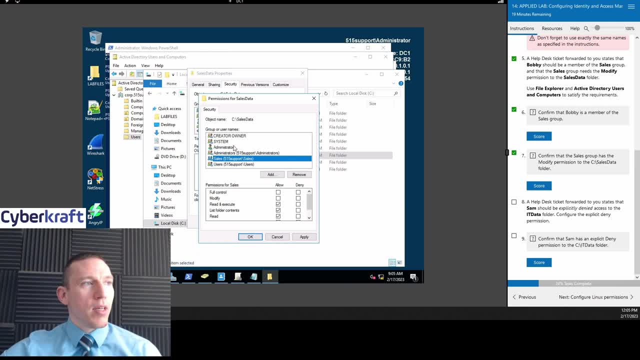 dot sales as a group here and once we've selected that as a group, we're gonna go ahead and go down here and allow modify permissions. okay, we'll keep the rest of the permissions. you know: rewrite, modify, execute. we have read and execute and now we're allowing modify. 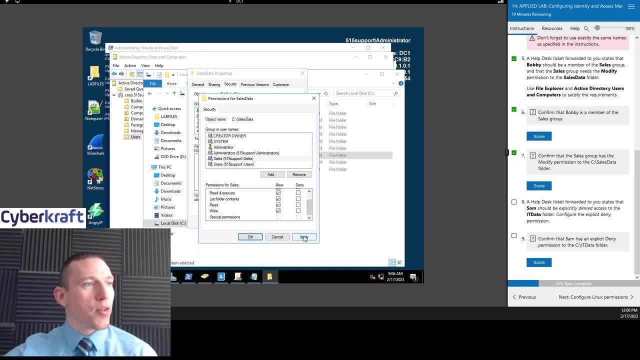 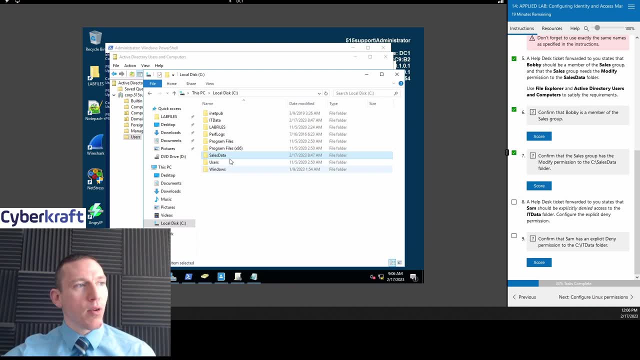 so almost full control essentially. well, basically full control. we're going to hit, apply there, and that's how we we've. we've done this at the permissions. we're going to hit, apply there, and that's how we've. we've done this at the permission level, okay. or we've done this at the folder level, which is how you're going to be doing it through. 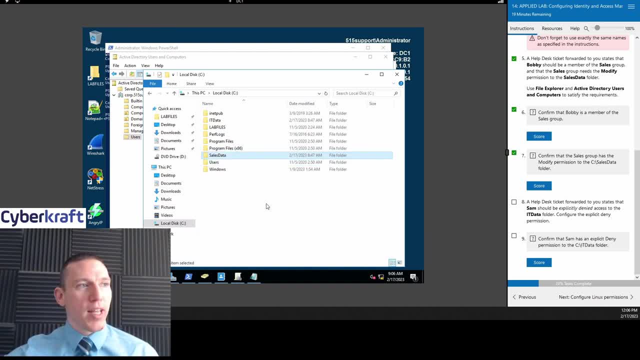 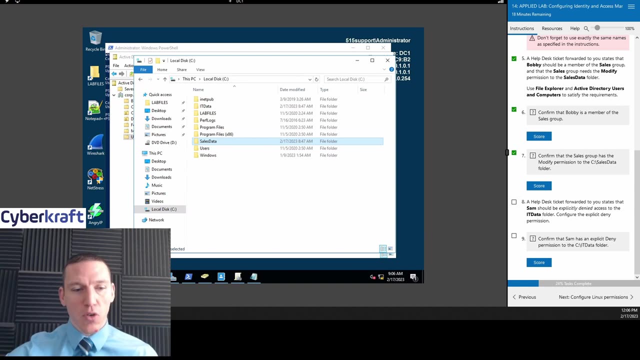 a new technology file system. you know the controls are done at the folder or the file system or file level. now, what type of access control method does this demonstrate for you guys? so if you remember, you have to look at your access control methods. which one would this demonstrate here? 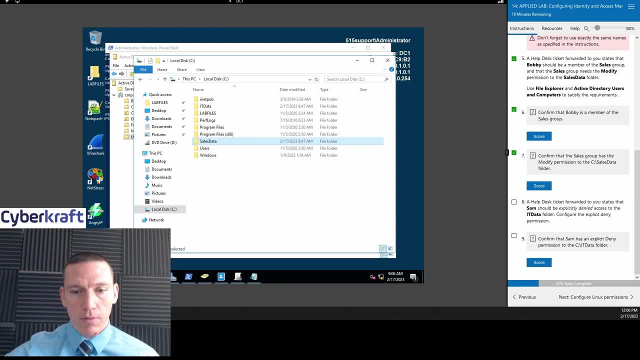 so, if you remember, you have to look at your access control method. which one would this demonstrate here? anyone want to take a stab? anyone want to take a stab? yeah, okay, so this is going to be discretionary access control or DAC d-a-c- all right? yeah, okay, so this is going to be discretionary access control or DAC d-a-c- all right. 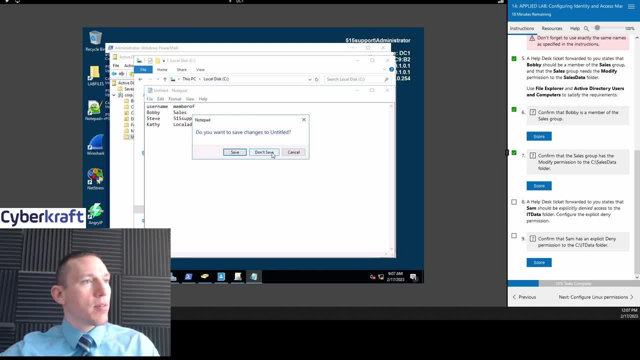 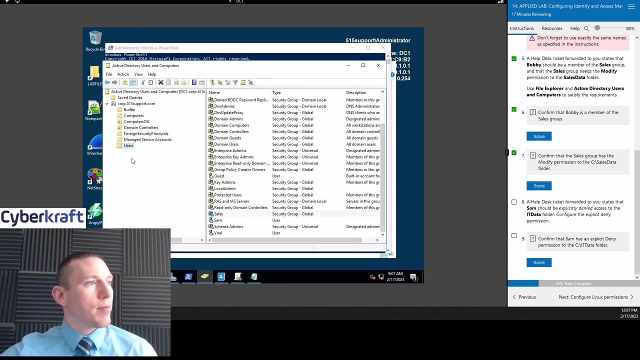 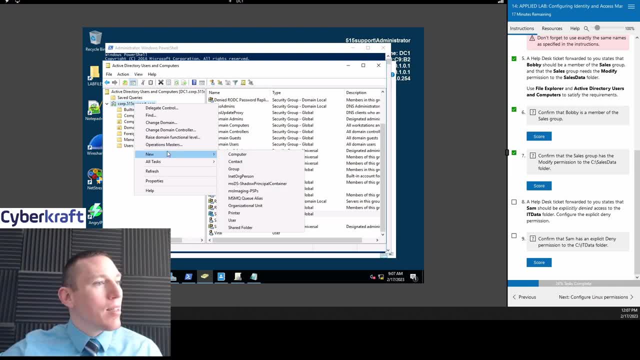 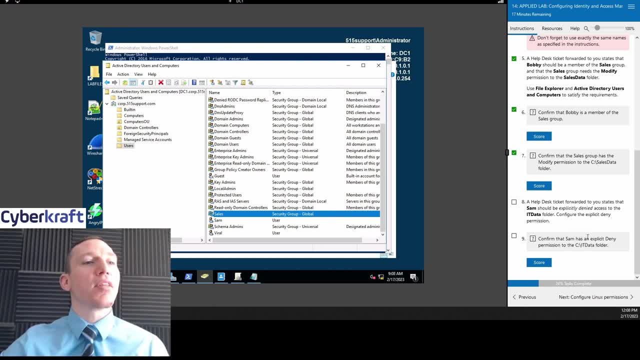 okay, but we do so. let's see, did we do? okay, but we do so. let's see, did we do everything? what else do we have to do everything? what else do we have to do everything? what else do we have to do? sam has to have explicit deny privileges. 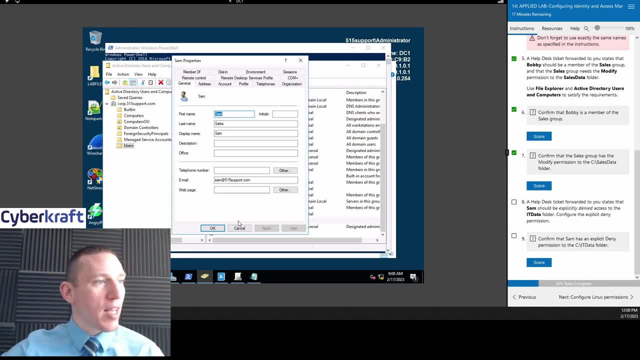 sam has to have explicit deny privileges. sam has to have explicit deny privileges to the it data folder. okay, so let's to the it data folder. okay, so let's to the it data folder. okay, so let's take a look at sam. he's a member of the. 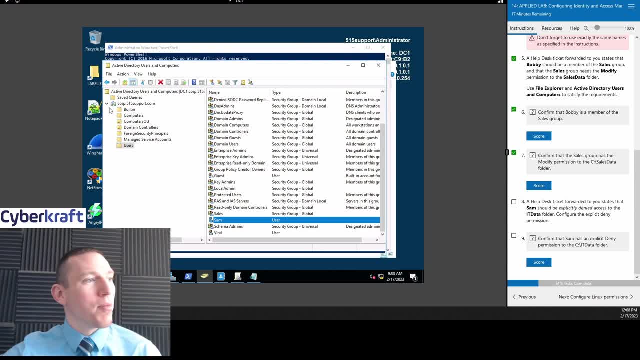 take a look at sam: he's a member of the. take a look at sam. he's a member of the domain users and the sales group domain users and the sales group domain users and the sales group. okay, so i don't know why the lab wants. okay, so i don't know why the lab wants. 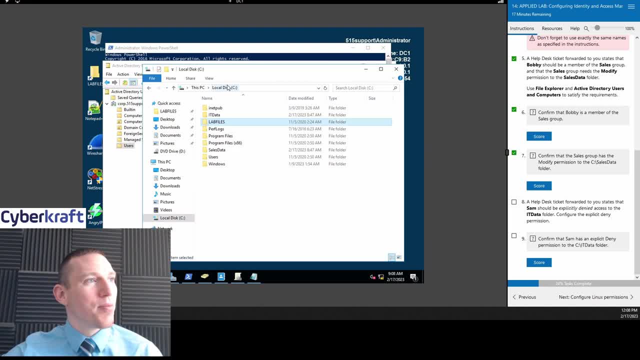 okay. so i don't know why the lab wants to uh, to uh, to uh, hate on sam so much. but they don't want hate on sam so much. but they don't want hate on sam so much. but they don't want sam to access this new folder. 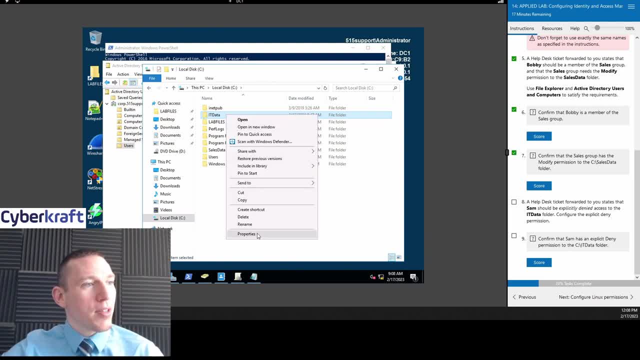 sam to access this new folder. sam to access this new folder. it data, so let's go ahead. and it data, so let's go ahead. and it data, so let's go ahead. and properties, so at the folder level properties, so at the folder level properties, so at the folder level, we're going to go ahead. 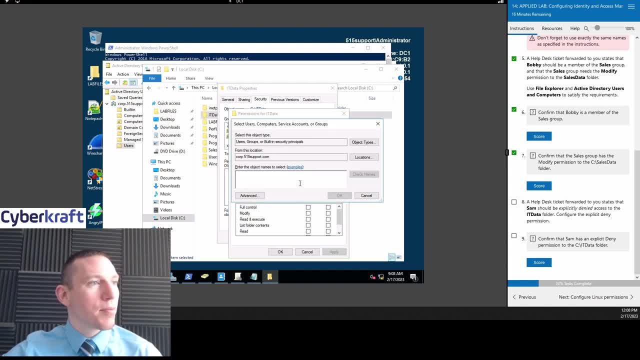 we're going to edit this. we're going to. we're going to edit this. we're going to. we're going to edit this. we're going to add: see, can we check? can we just add one? see, can we check? can we just add one person? yeah, we can. 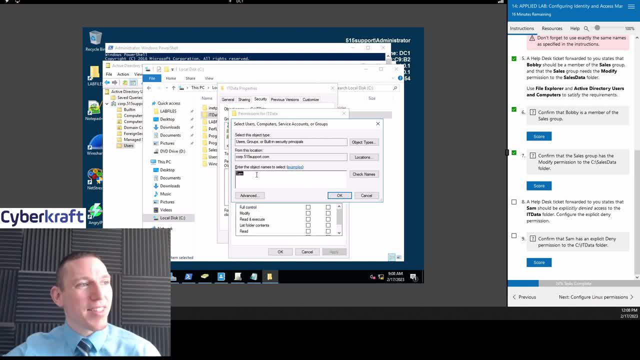 person. yeah, we can person, yeah, we can. okay. okay, so we're adding sam as an. okay, okay, so we're adding sam as an. okay, okay, so we're adding sam as an object here, object here. object here: uh, 515 support slash sam. okay, and we're gonna go ahead and let's. 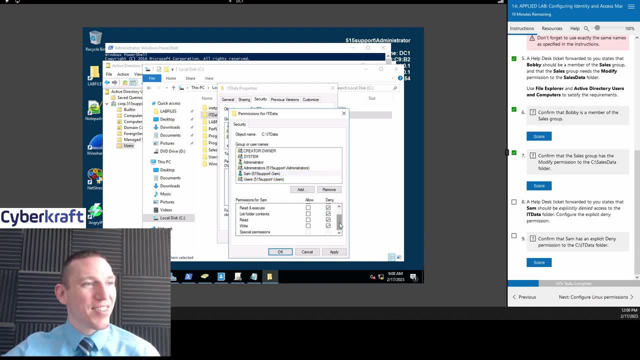 okay, and we're gonna go ahead, and let's okay, and we're gonna go ahead, and let's just just just deny him everything. so, deny him everything, so deny him everything. so what does it say explicit deny permission? what does it say explicit deny permission? what does it say explicit deny permission? okay, that's fine. 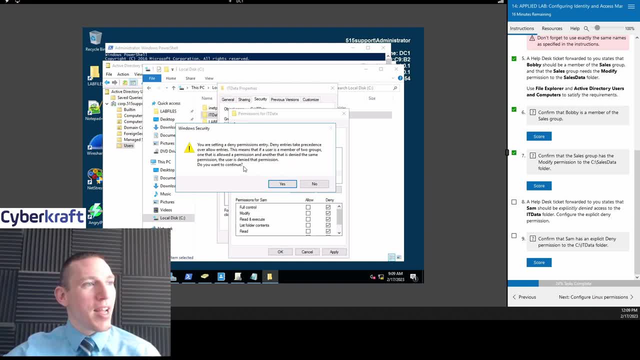 yep if the user of two groups one is yep if the user of two groups one is yep. if the user of two groups one is allowed permission, the other is denied allowed permission. the other is denied allowed permission, the other is denied the same permission. these are: 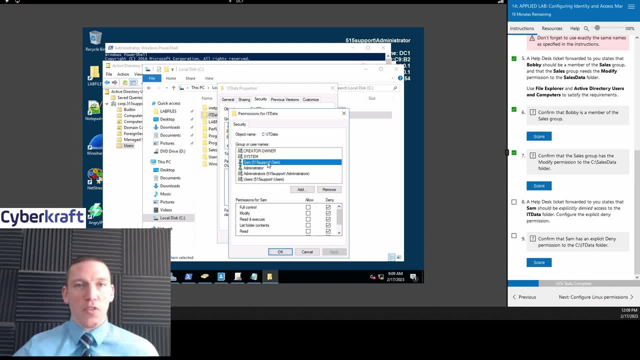 the same permission. these are the same permission. these are denying that permission. yeah, denying that permission. yeah, denying that permission. yeah, basically what that's saying is even basically what that's saying is even basically. what that's saying is: even though, if, though, if, though, if sam is part of, like, the admin group, okay, 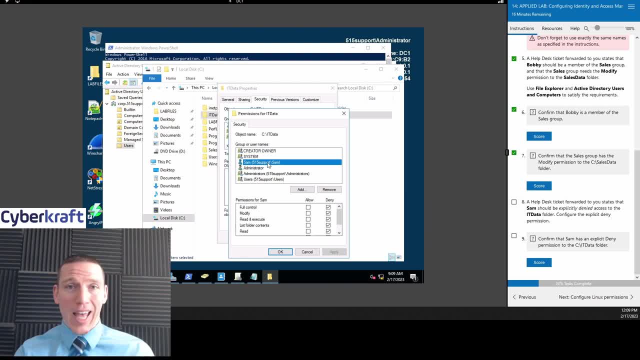 sam is part of, like the admin group, okay, sam is part of like the admin group, okay, and the admin group has full control. and the admin group has full control and the admin group has full control. full permission. full allow permissions on. full permission. full allow permissions on. 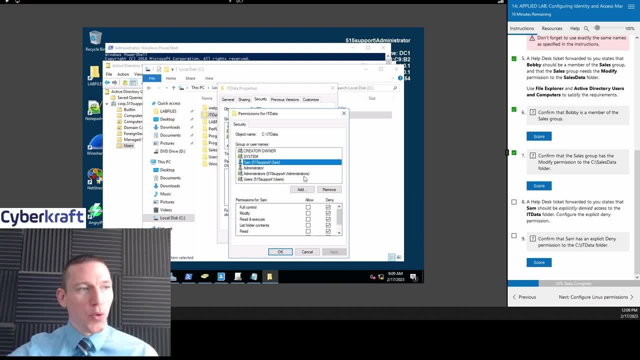 full permission, full allow permissions on that folder, that folder, that folder. since we've made this explicit deny rule, since we've made this explicit deny rule, since we've made this explicit deny rule where we're in denying everything, remember where we're in denying everything. remember where we're in denying everything. remember, explicit deny is denied by default. 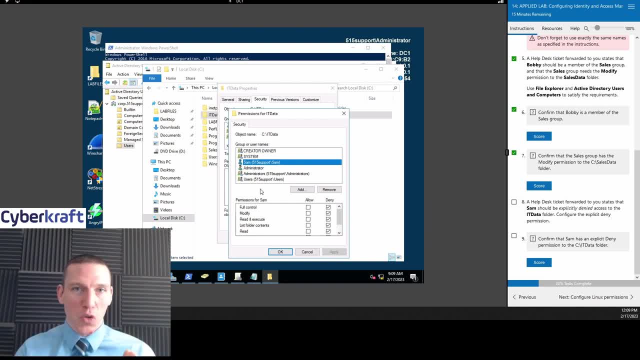 explicit deny is denied by default. explicit deny is denied by default. the deny rule would take precedence. the deny rule would take precedence. the deny rule would take precedence because we've created a special rule for. because we've created a special rule for. because we've created a special rule for sam. 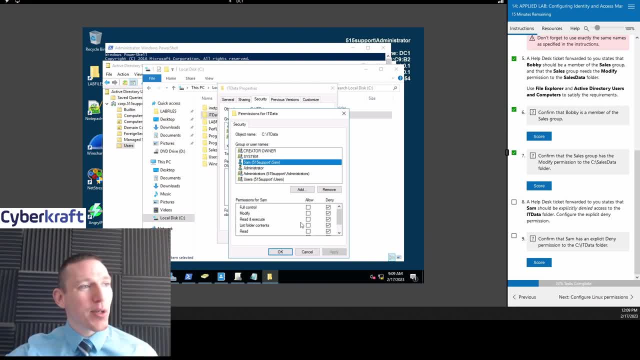 sam sam. apparently sam messed something up. apparently sam messed something up. apparently sam messed something up. apparent in the it data folder. apparent in the it data folder. apparent in the it data folder. and we're we're punishing him or we're, and we're we're punishing him or we're. 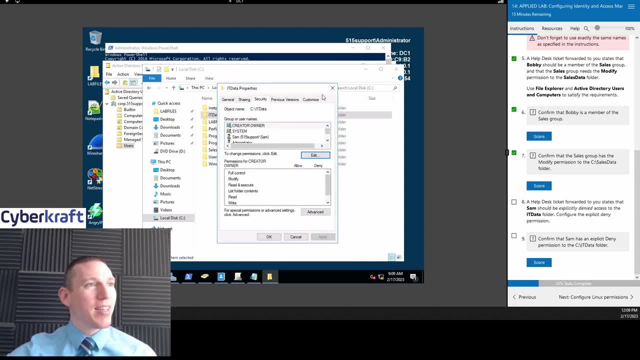 and we're we're punishing him or we're making sure he doesn't do that again. so making sure he doesn't do that again, so making sure he doesn't do that again. so we're putting this explicit deny, we're putting this explicit deny, we're putting this explicit deny: uh, permission on this folder itself. 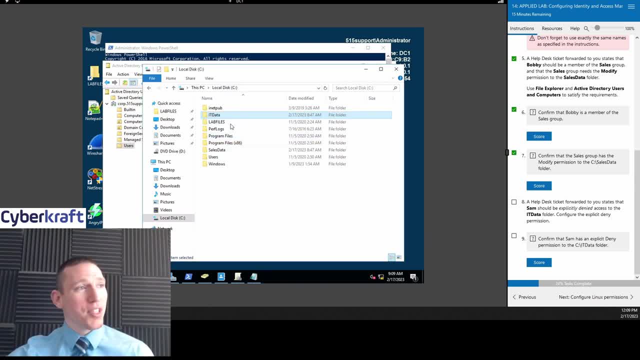 uh, permission on this folder itself. uh, permission on this folder itself. okay, so we're modifying this at the okay. so we're modifying this at the okay. so we're modifying this at the folder level, just like we did for folder level, just like we did for folder level, just like we did for bobby and the sales data. 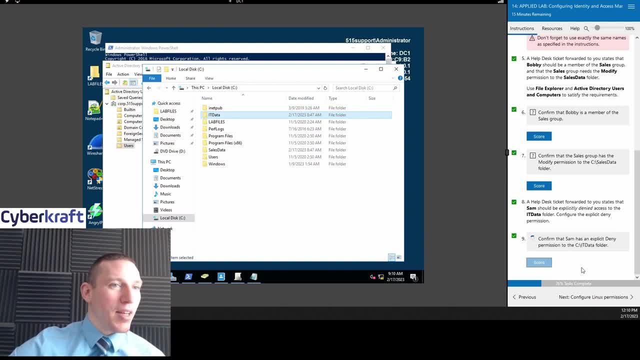 bobby and the sales data. bobby and the sales data. okay, so that's kind of interesting that. okay, so that's kind of interesting, that okay, so that's kind of interesting that we had to do that and then we can score. we had to do that and then we can score. 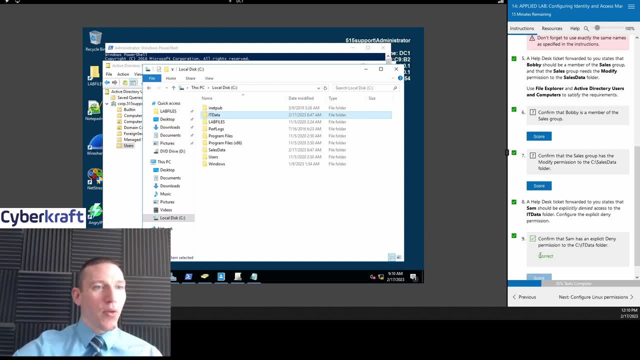 we had to do that, and then we can score that, that, that and that should work, and we did get it, and that should work, and we did get it, and that should work, and we did get it correct, all right, correct, all right, correct, all right. so great. so this, this part, could be a. 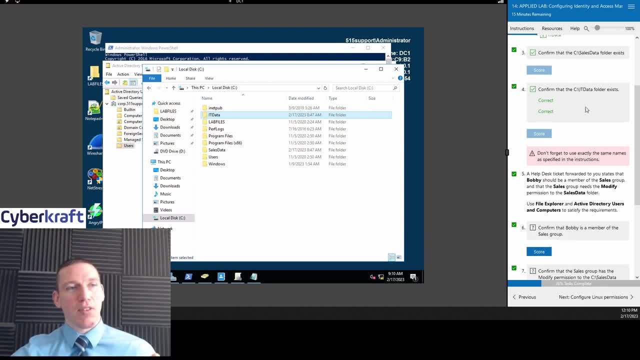 so great, so this this part could be a so great, so this this part could be a little confusing whenever they uh little confusing, whenever they uh little confusing, whenever they uh, whenever the lab doesn't, whenever the lab doesn't, whenever the lab doesn't tell you exactly where to go, you know. 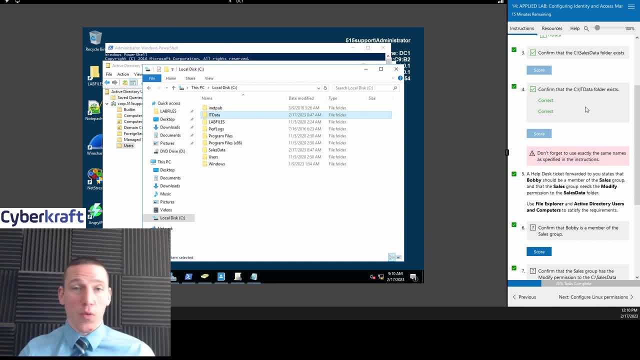 tell you exactly where to go. you know tell you exactly where to go. you know the way the lab is organized, the way the lab is organized, the way the lab is organized. that could be very different from what. that could be very different from what. that could be very different from what you'll see on the job. 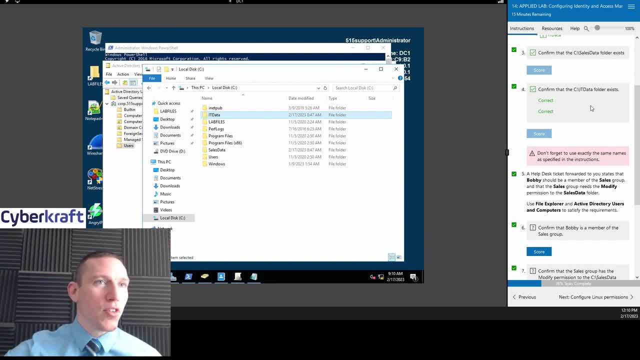 you'll see on the job. you'll see on the job. so it really should tell you exactly. so it really should tell you exactly. so it really should tell you exactly where these objects are. so, if you do get where these objects are, so if you do get, 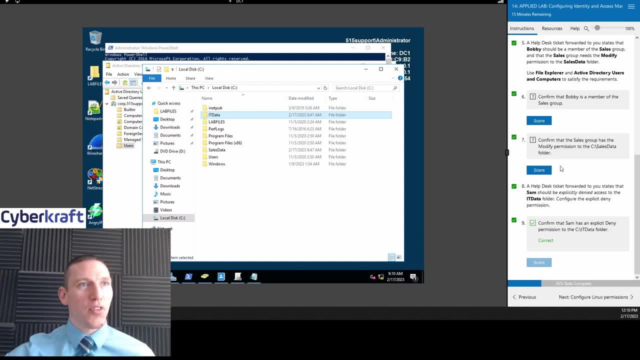 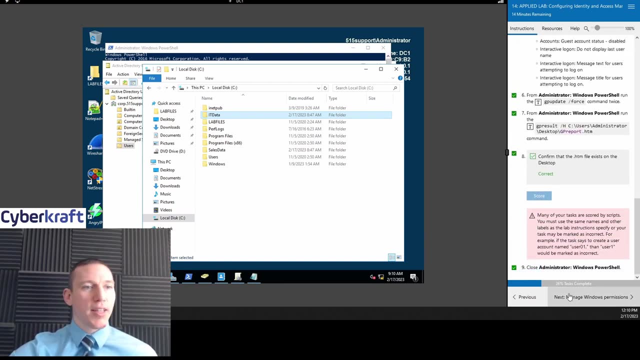 where these objects are. so if you do get a little confused, that's why i do these a little confused, that's why i do these a little confused, that's why i do these security policy, security policy, security policy section. and then the level of detail in section, and then the level of detail in 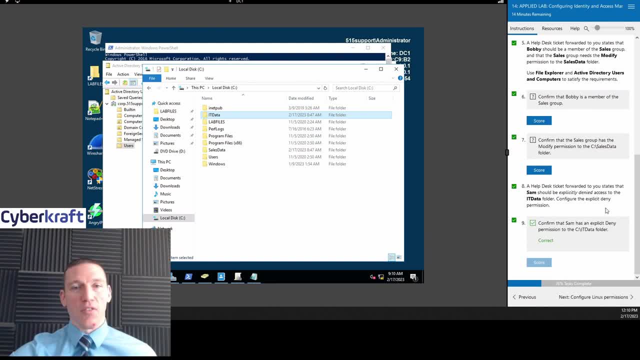 section and then the level of detail in the ntfs windows permissions. the ntfs windows permissions, the ntfs windows permissions section. they're very different. you have section. they're very different. you have section. they're very different. you have two different people writing these. two different people writing these. 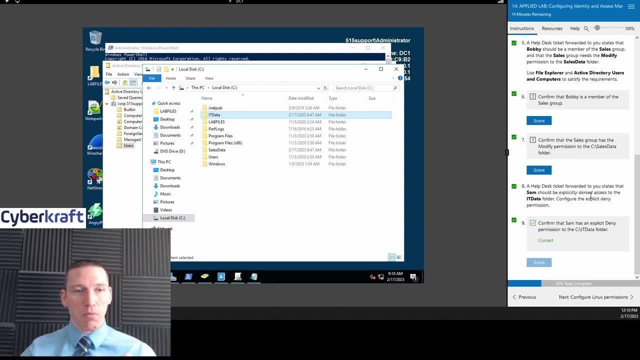 two different people writing these. okay, so the labs are kind of a hodgepodge. okay, so the labs are kind of a hodgepodge. okay, so the labs are kind of a hodgepodge of scenarios, of scenarios, of scenarios linked together, so sometimes they can. 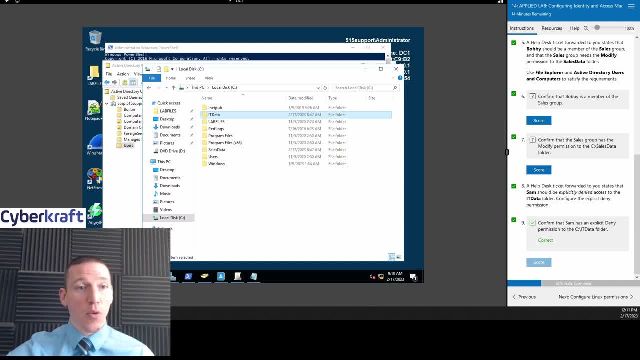 linked together. so sometimes they can linked together. so sometimes they can be very confusing and you can have a be very confusing and you can have a be very confusing and you can have a confusing section, confusing section, confusing section in an otherwise pretty easy to understand, in an otherwise pretty easy to understand. 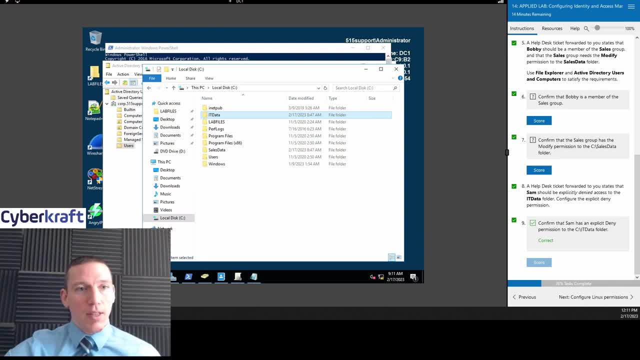 in an otherwise pretty easy to understand lab: lab, lab. so that's why we do these walkthroughs. so that's why we do these walkthroughs. so that's why we do these walkthroughs. okay, anyway, i think we should be good i. okay, anyway, i think we should be good i. 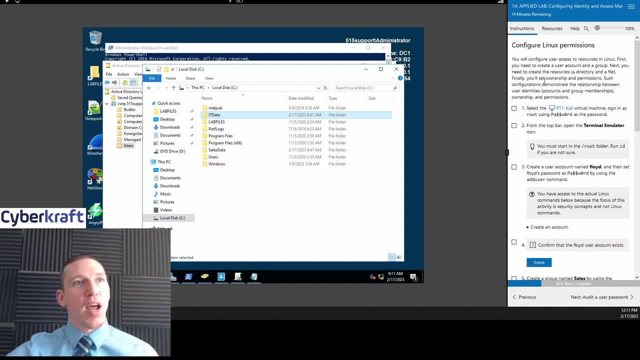 okay, anyway, i think we should be good. i don't know if we're gonna be using. don't know if we're gonna be using. don't know if we're gonna be using domain controller- one anymore domain controller, one anymore domain controller, one anymore. okay, so now we're gonna be doing linux. 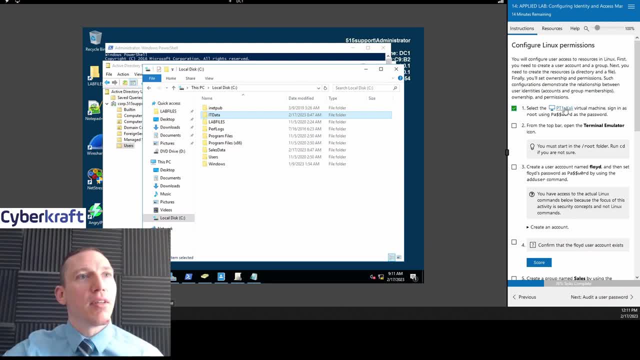 okay, so now we're gonna be doing linux. okay, so now we're gonna be doing linux. commands, actually, we'll probably commands. actually, we'll probably commands. actually, we'll probably, we'll probably go to ms1 to do the. we'll probably go to ms1 to do the. 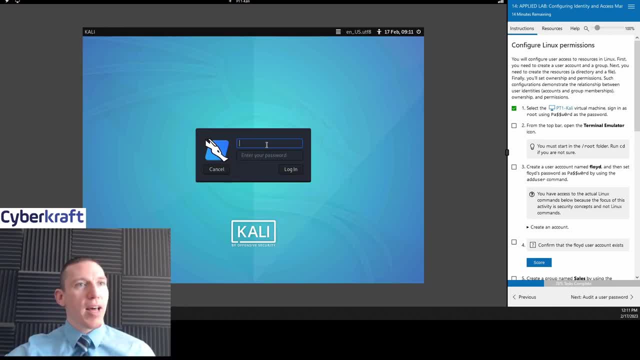 we'll probably go to ms1 to do the the ssl certificates. but let's go ahead, the ssl certificates, but let's go ahead, the ssl certificates, but let's go ahead and go to, and go to, and go to cali, uh, cali, uh, cali, uh, still using this old version of cali. so 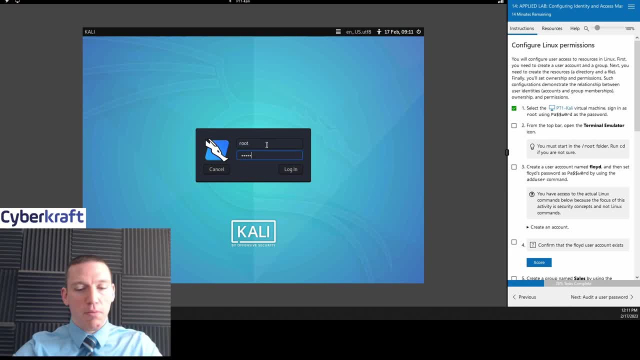 still using this old version of cali. so still using this old version of cali. so it's root and then password. it's root and then password. it's root and then password. make sure password has a zero and not a. make sure password has a zero and not a. 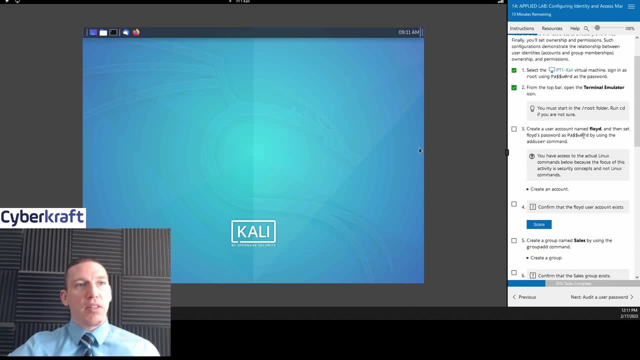 make sure password has a zero and not a o, and basically we're going to be doing, and basically we're going to be doing, and basically we're going to be doing everything through the terminal, everything through the terminal, everything through the terminal. this can be pretty easy, but if you mess, 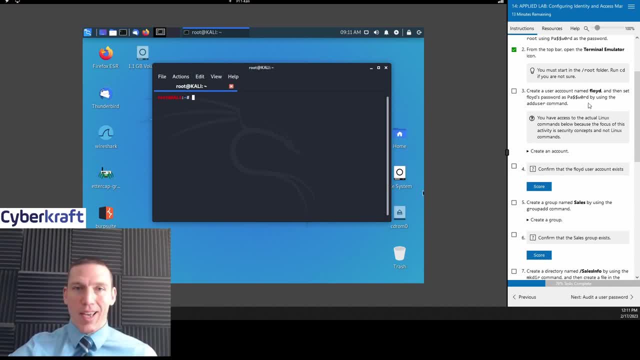 this can be pretty easy. but if you mess, this can be pretty easy. but if you mess up up up, you know with the the cali machine, you, you know with the the cali machine, you, you know with the the cali machine, you can't use that type. 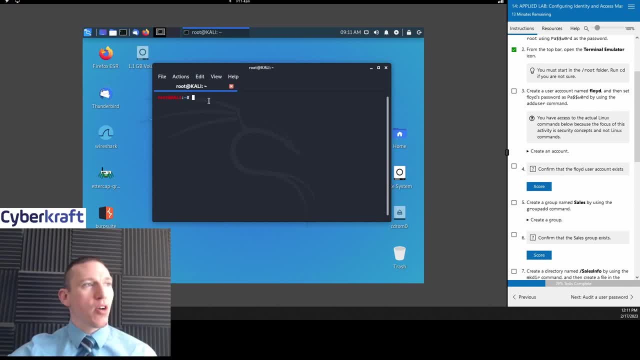 can't use that type. can't use that type set helper. you can't click the type set helper. you can't click the type set helper. you can't click the type. command- it's not going to work. command it's not going to work. command: it's not going to work because they didn't script this super. 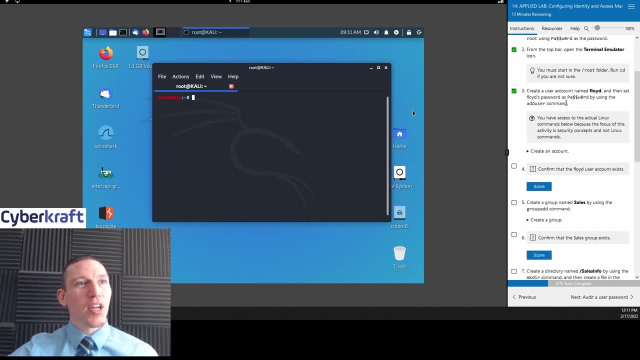 because they didn't script this super, because they didn't script this super well, well, well. so, what we're going to do, so, what we're going to do, so, what we're going to do, is work through our is work through our is work through our. we have to navigate. we're going to do. 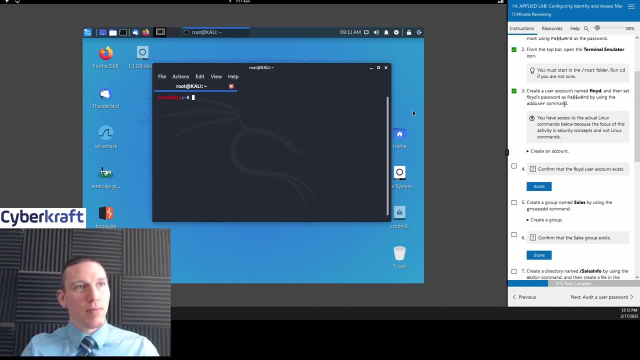 we have to navigate, we're going to do, we have to navigate, we're going to do this through linux. okay, through the this through linux. okay, through the this through linux. okay, through the linux command. linux command, linux command. okay, so let's see, are we in the root command? 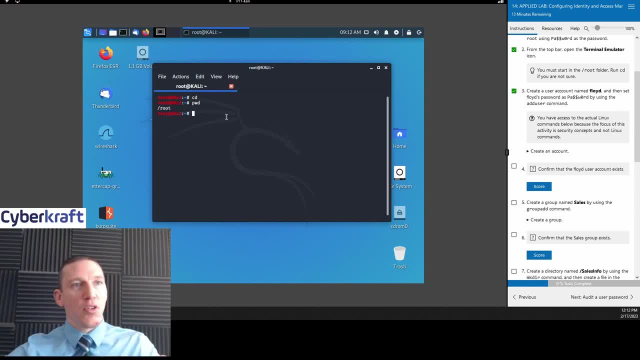 let's see. are we in the root command? let's see, are we in the root command? let's see. let's see. let's see. okay now. if you don't know if you're in, okay now. if you don't know if you're in, okay now. if you don't know if you're in the root directory. 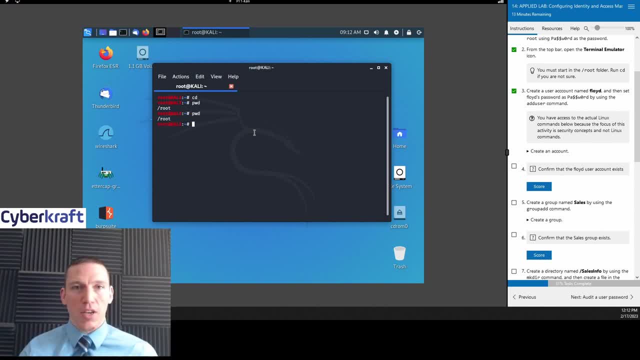 the root directory. the root directory just do: pwd. pwd tells you what your just do. pwd pwd tells you what your just do. pwd pwd tells you what your current directory is. current directory is, current directory is, and we should be in slash root. okay, and we should be in slash root okay. 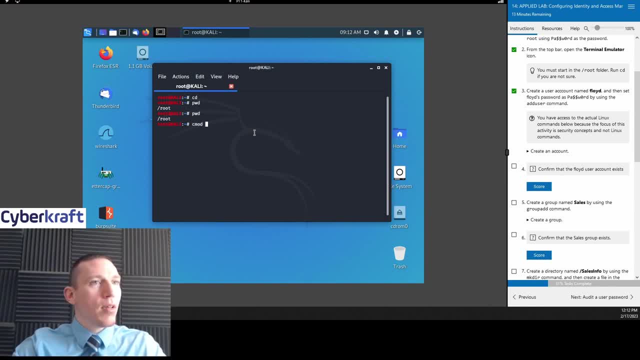 and we should be in slash root. okay, so we should do. we should add an account now, floyd now. we should add an account now, floyd now. we should add an account now floyd, now it should it's going to tell you. it should. it's going to tell you. 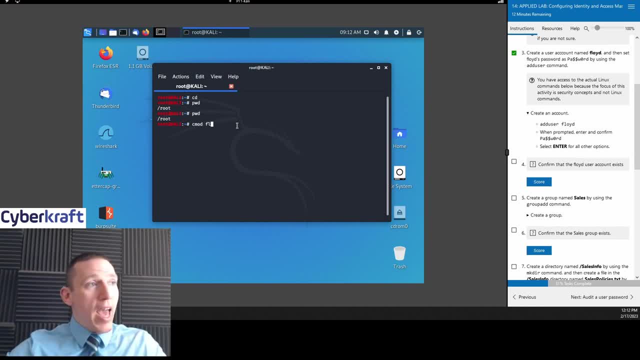 it should. it's going to tell you: oh yeah, what am i doing? oh yeah, what am i doing? oh yeah, what am i doing? add user floyd, sorry. add user floyd, sorry. add user floyd, sorry. we're not changing any permissions on. we're not changing any permissions on. 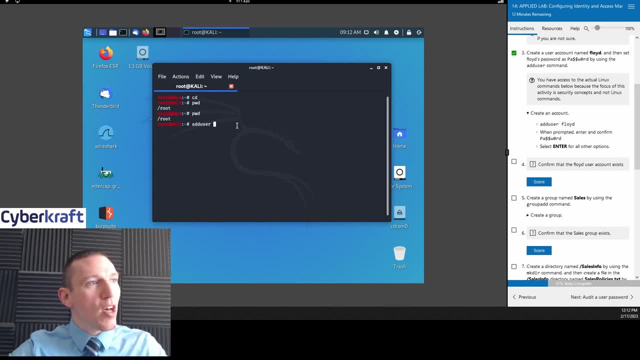 we're not changing any permissions on folders just yet. cmods used to change folders just yet. cmods used to change folders just yet. cmods used to change permissions on on certain objects. permissions on on certain objects. permissions on on certain objects. add user floyd. okay, we're going to create a password. 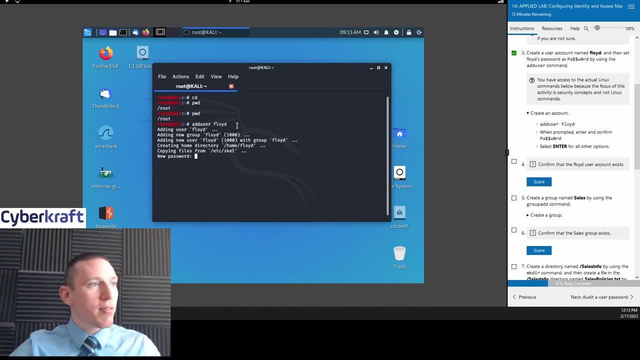 okay, we're going to create a password. okay, we're going to create a password for them. we're going to use that same for them. we're going to use that same for them. we're going to use that same password we use for everything. password, we use for everything. 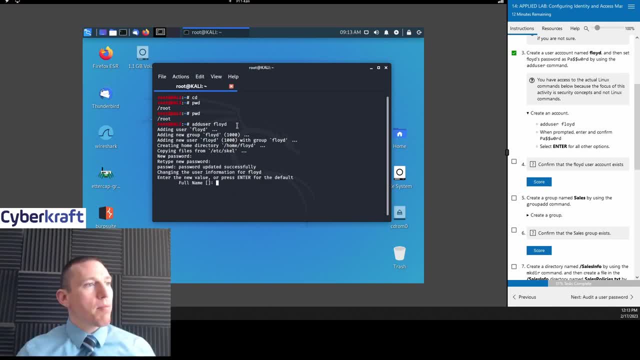 password we use for everything: retype that, retype that, retype that. okay, now, basically, we've created the user. okay, now, basically, we've created the user. okay, now, basically, we've created the user, now for now, for now, for called floyd. we've set his password as: 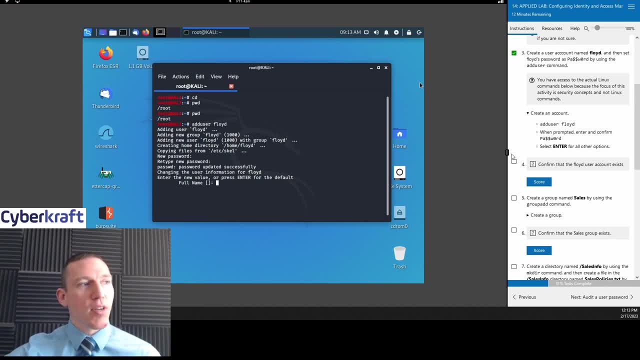 called floyd. we've set his password as called floyd. we've set his password as the password here, the password here. the password here: pa dollar sign. dollar sign w zero rd. pa dollar sign. dollar sign w zero rd. pa dollar sign. dollar sign w zero rd. okay. 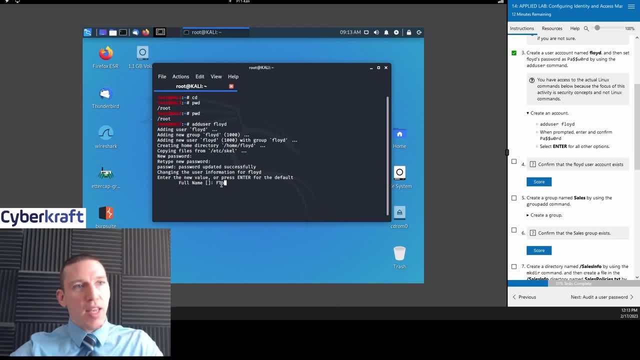 okay, okay, full name. it says to enter for all the other. it says to enter for all the other. it says to enter for all the other options. we can go ahead and do that options. we can go ahead and do that options. we can go ahead and do that. that's fine. yes, the information is: 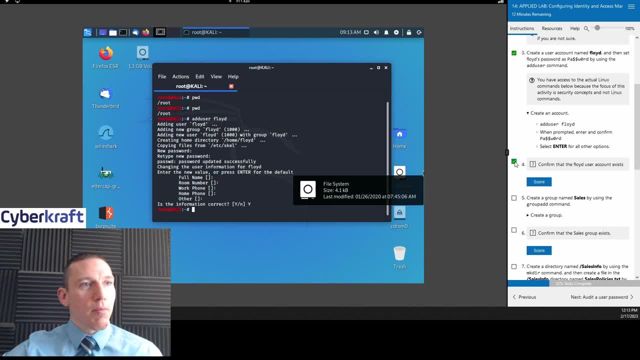 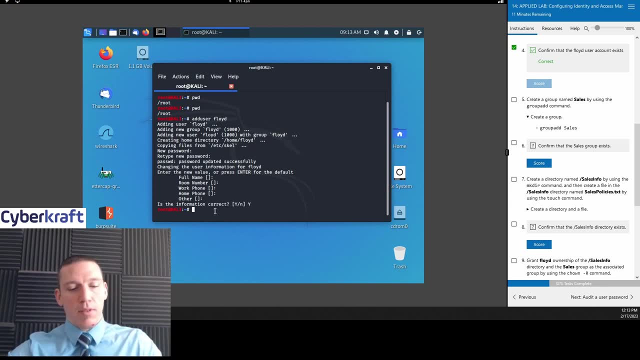 that's fine. yes, the information is. that's fine. yes, the information is correct, correct, correct, boom. okay. now we're going to create a group. okay, now we're going to create a group. okay, now we're going to create a group. okay, group add group add group, add sales. 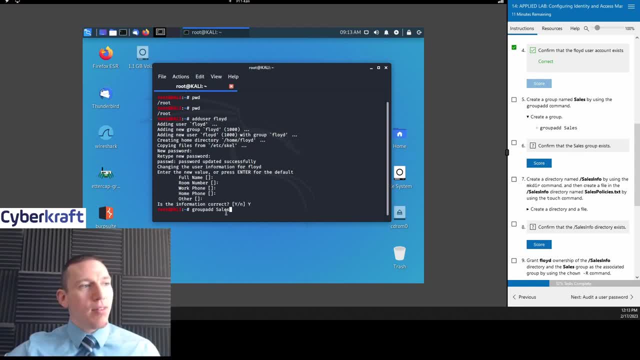 sales sales. group ad. group ad. group ad uh. group ad- uh. group ad uh. can be a little confusing because it's add can be a little confusing because it's add. can be a little confusing because it's add user and then group user and then group user and then group add. just remember that group ad. 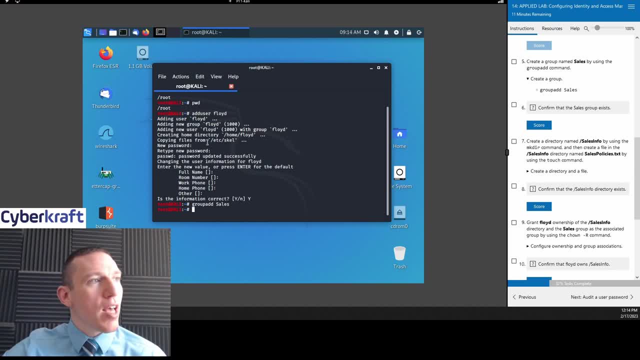 add, just remember that group ad. add, just remember that group ad. you know if you're going to add a group. you know if you're going to add a group. you know if you're going to add a group, flip-flop from, flip-flop from, flip-flop from add user. so we create that sales group it. 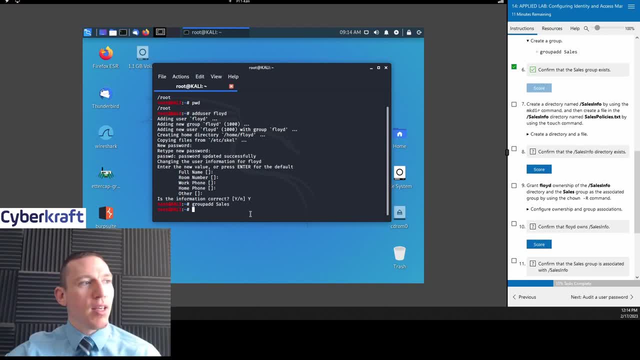 add user, so we create that sales group. it add user, so we create that sales group. it doesn't give us any more prompt for the, doesn't give us any more prompt for the, doesn't give us any more prompt for the sales group, sales group, sales group. so if it just goes right back to the 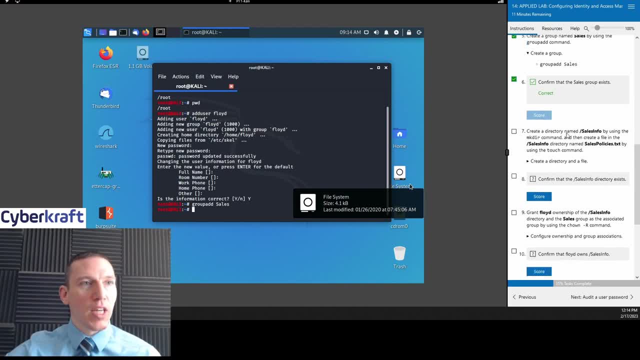 so if it just goes right back to the, so if it just goes right back to the terminal, it's fine terminal. it's fine terminal, it's fine. and if you score it with the script, we, and if you score it with the script, we, and if you score it with the script, we did it correctly because it scored. 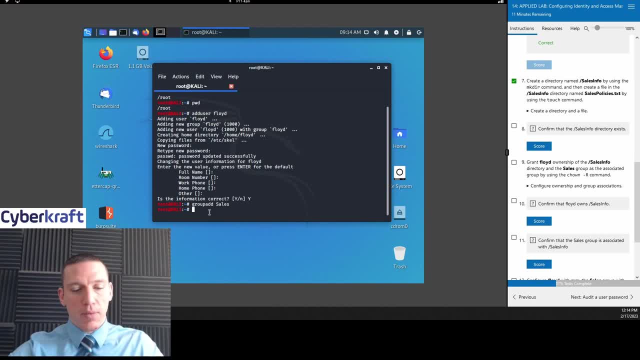 did it correctly because it scored. did it correctly because it scored, just right, okay. so now we're going to just right, okay, so now we're going to just right, okay. so now we're going to create a directory. create a directory, create a directory. mkdir, mkdir, mkdir. let me expand this out so you can see. 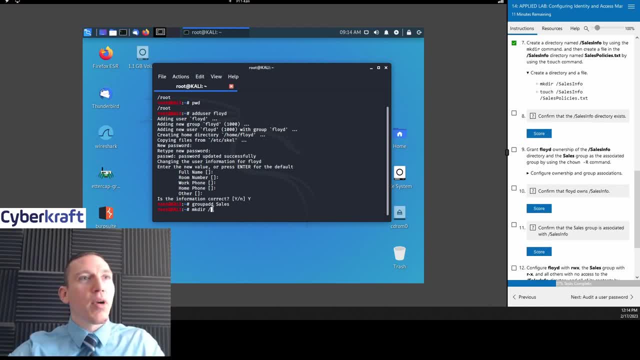 let me expand this out so you can see. let me expand this out so you can see. this, this, this slash, what does it want us to? sales slash? what does it want us to sales slash? what does it want us to sales info, info, info. wants us to call this sales info. 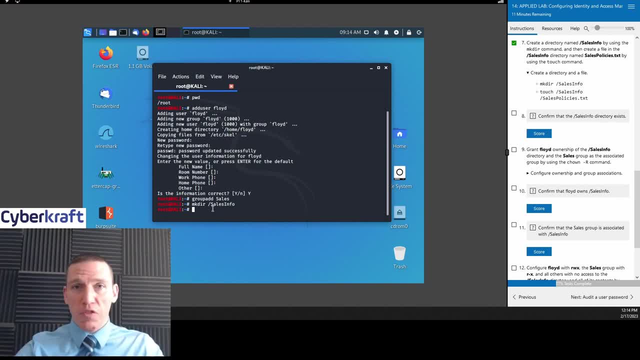 okay, and then we're going to create, okay, and then we're going to create okay, and then we're going to create a file. remember to create a file. use the a file. remember to create a file. use the a file. remember to create a file. use the touch command. 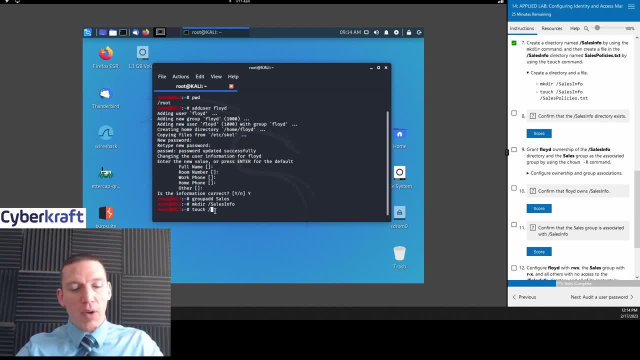 touch, and then we're going to specify touch. and then we're going to specify touch. and then we're going to specify where we want that file, so sales where we want that file. so sales where we want that file, so sales info. and then we're going to. 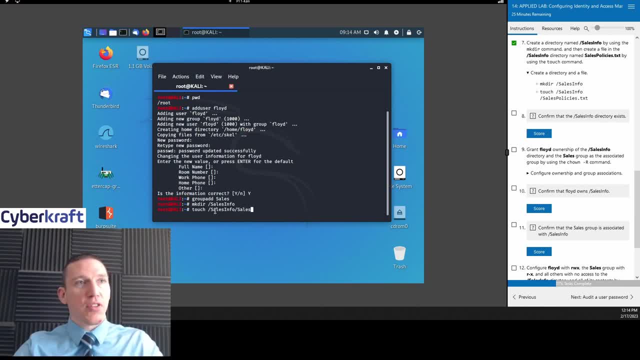 info, and then we're going to info, and then we're going to specify the file that we want to create. specify the file that we want to create, specify the file that we want to create and that file is going to be sales and that file is going to be sales. 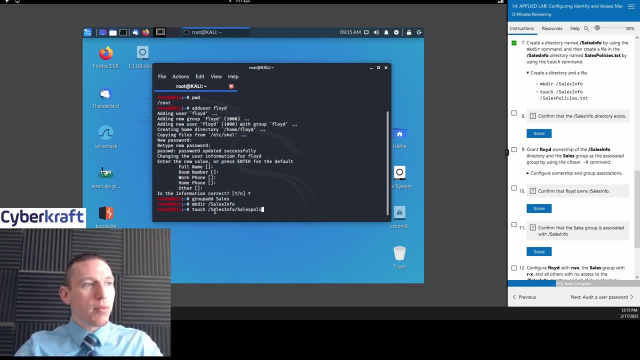 and that file is going to be sales policies, policies, policies, policies, plural. we'll make sure the text, we'll make sure the text, we'll make sure the text matches the case, matches the case matches the case. okay, sales policiestxt. okay, sales policiestxt. okay, sales policiestxt. creating a text file using the touch. 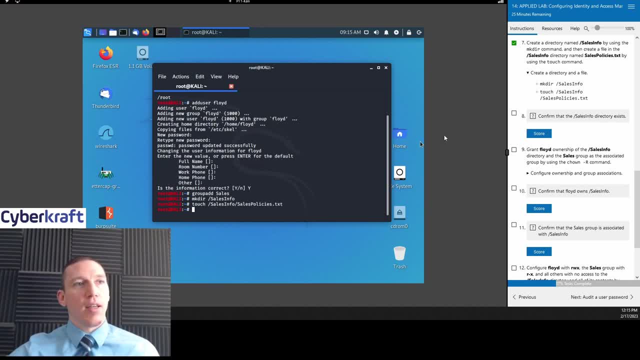 creating a text file using the touch. creating a text file using the touch command in the sales info file. command in the sales info file. command in the sales info file. now the script is going to help ensure, now the script is going to help ensure, now the script is going to help ensure that we did that correctly. 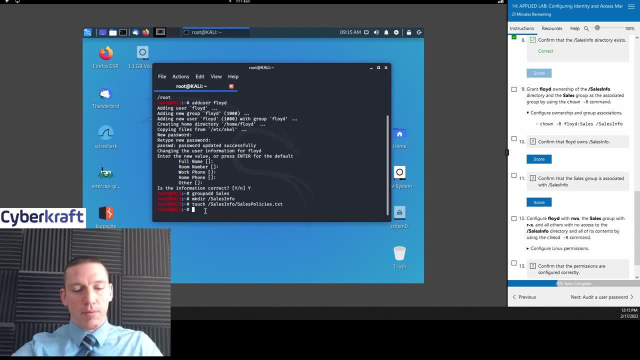 that we did that correctly, that we did that correctly, okay, and now we're going to make sure, okay, and now we're going to make sure, okay, and now we're going to make sure that, um, that, um, that, um, floyd has permissions to that, so we're. 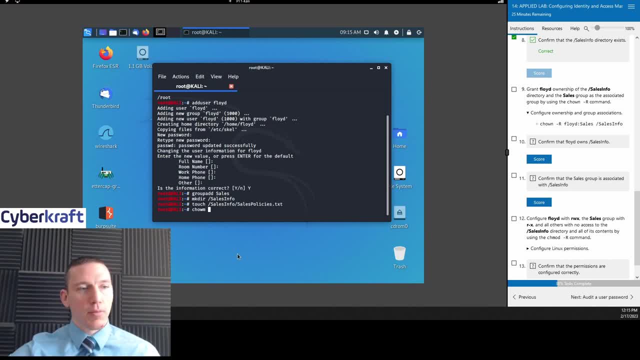 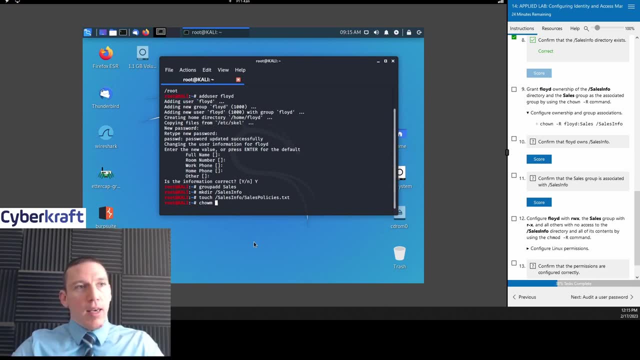 floyd has permissions to that, so we're. floyd has permissions to that, so we're going to c own and uh c own, not own. and uh c own, not own and uh c own, not own. change ownership, ch own, change ownership, ch own, change ownership, ch own. dash r putting the dash r flag in. 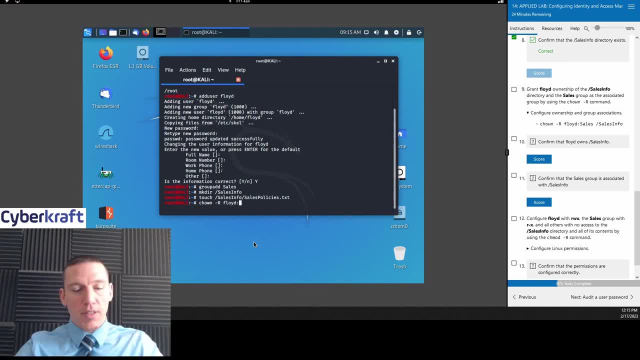 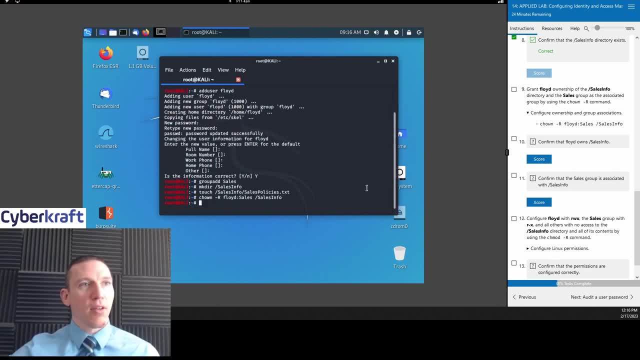 what we've done here, dash r, what we've done here, dash r promotes uh, changes it to the read. promotes uh, changes it to the read. promotes uh. changes it to the read command okay. or the um command okay, or the um command okay, or the um grants him ownership. 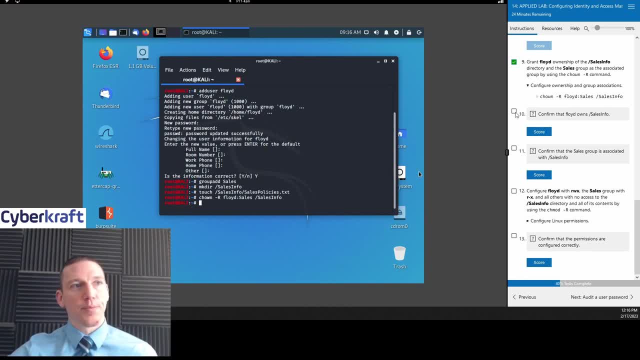 grants him ownership. grants him ownership within uh that command that flag dash. within uh that command that flag dash. within uh that command that flag dash r. it's not read it's full owner. it's not read it's full owner. it's not read it's full owner ownership. 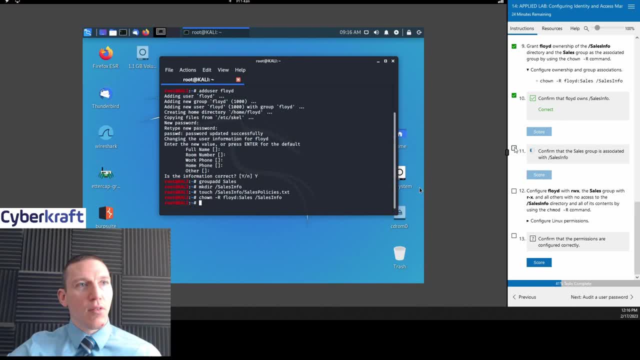 ownership, ownership, okay. so now let's see, we should confirm this, both of it there's. we should confirm this, both of it there's. we should confirm this, both of it there's. one command, one command, one command. uh, everything that we've done so far, uh, everything that we've done so far. 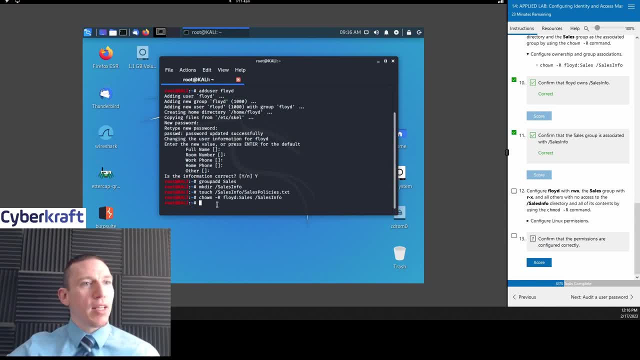 uh, everything that we've done so far should line up, should line up, should line up, and then let's see we can go ahead, and and then let's see we can go ahead, and and then let's see we can go ahead and configure floyd. configure floyd. 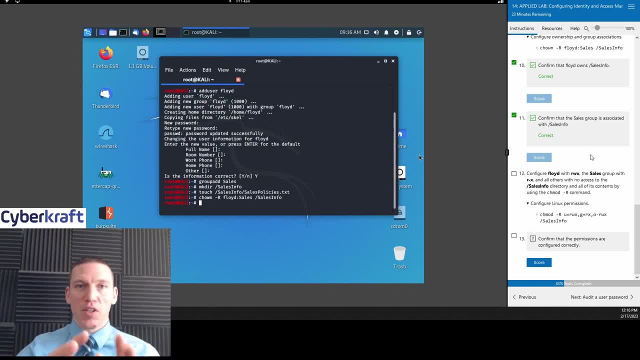 configure floyd now. this is a pretty good. this section is now. this is a pretty good. this section is now. this is a pretty good. this section is written pretty well, written pretty well. written pretty well. very self-explanatory, very easy to. very self-explanatory, very easy to. 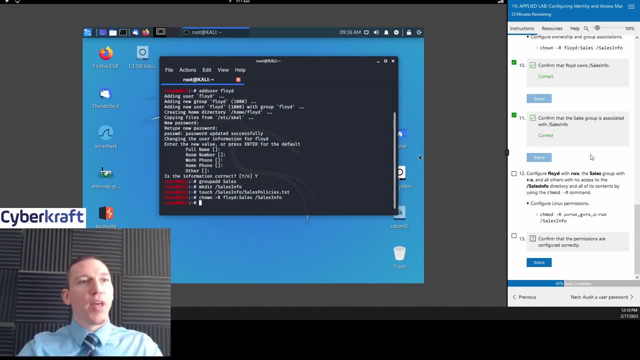 very self-explanatory, very easy to follow. so we're going to configure floyd follow. so we're going to configure floyd follow. so we're going to configure floyd with the, with the, with the read, write and execute, read, write and execute, read, write and execute in the sales group with. 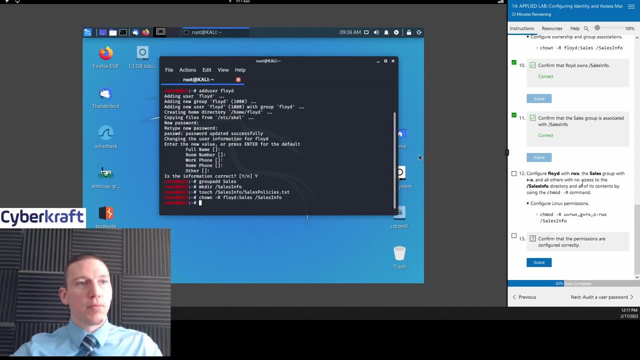 in the sales group with in the sales group with read. we're going to exclude, write and read. we're going to exclude, write and read. we're going to exclude, write and execute, execute, execute and all others with no access to sales and all others with no access to sales. 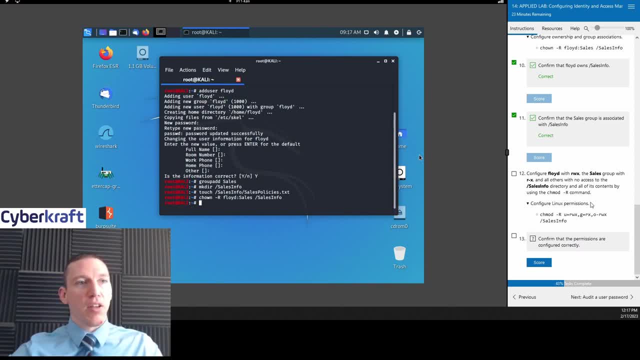 and all others with no access to sales info directory. info directory. info directory: all of its contents by using the c mod. all of its contents by using the c mod. all of its contents by using the c mod. change r okay, change r okay, change r okay. all right, so we're going to go to change. 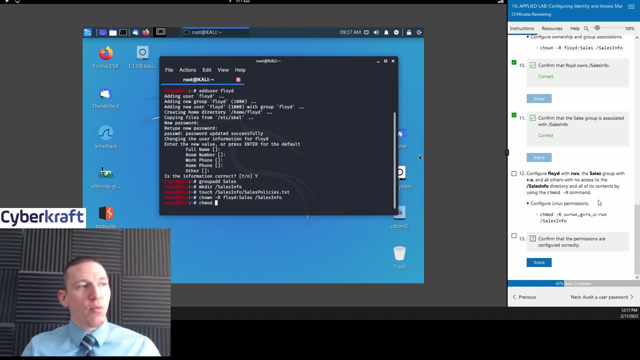 all right, so we're going to go to change. all right, so we're going to go to change ownership, ownership ownership, or see modify. we're going to modify using a dash r. we're going to modify using a dash r. we're going to modify using a dash r flag. 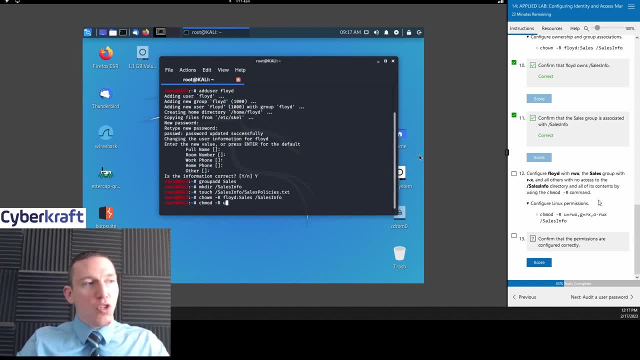 flag flag. now we're going to say: u equals rx, u equals rx, u equals rx. rwx- okay, remember rwx. okay, remember rwx. okay, remember, read, write and execute rwx. that's what read, write and execute rwx. that's what read, write and execute rwx. that's what those stand for. 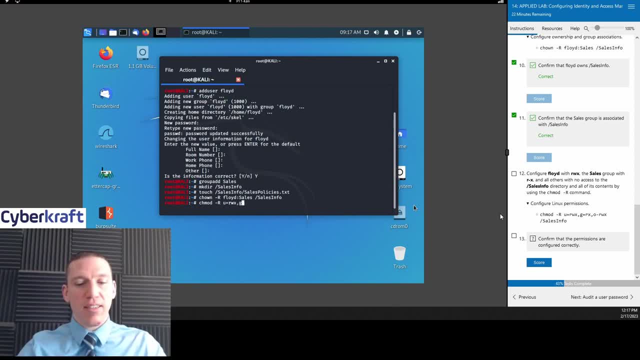 those stand for. those stand for: make sure you have a comma, no space g. make sure you have a comma, no space g. make sure you have a comma, no space g. equals, equals, equals, rx, rx, okay, okay, okay, o rwx, rwx, rwx, slash sales, slash sales. 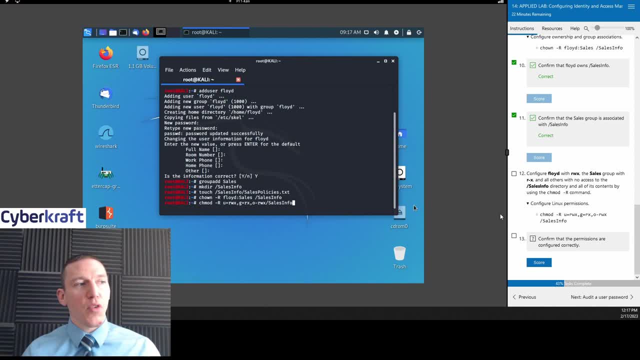 slash sales info, info, info. okay. so what have we done here? okay. so what have we done here? okay. so what have we done here? u is going to stand for the user, okay? so let's see: configure floyd with rwx. so let's see: configure floyd with rwx. 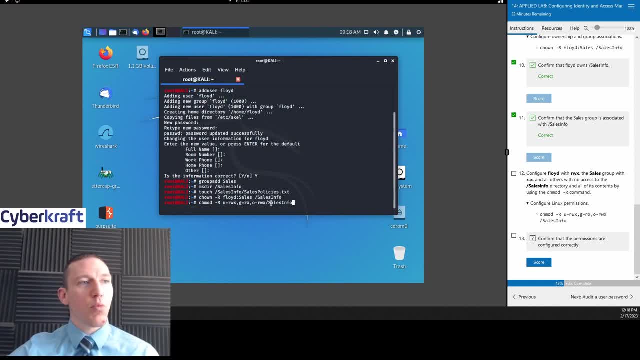 so let's see, configure floyd with rwx so that's going to be, so, that's going to be, so that's going to be. floyd there group, floyd there group, floyd there group. sales group with r. sales group with r. sales group with r. read, no, write and execute. so read and. 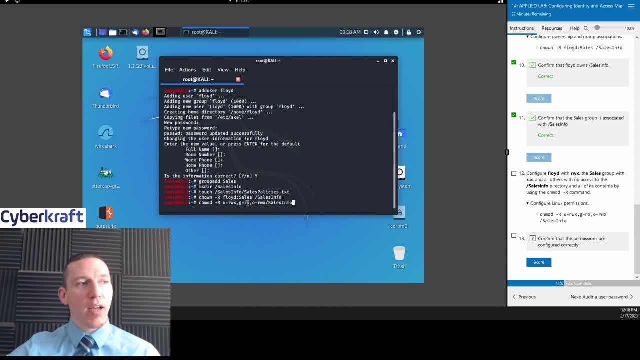 read, no write and execute. so read and read. no write and execute. so read and execute, execute, execute. okay, and we would just do that with rx. you okay, and we would just do that with rx. you okay, and we would just do that with rx. you don't need to put that dash in there. 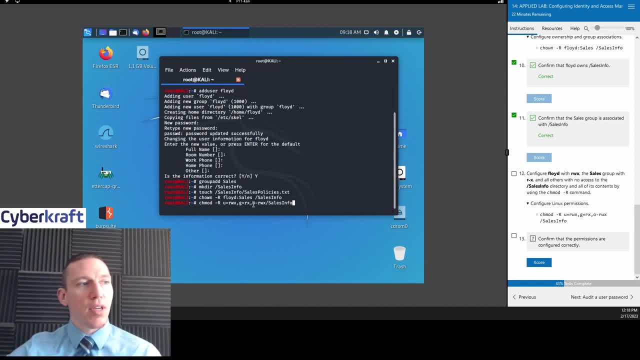 don't need to put that dash in there, don't need to put that dash in there. and then, and then, and then, uh, all others, uh, all others, uh, all others, others, others, others, read, write, execute, read, write, execute, read, write, execute or no, uh, others are going to be. 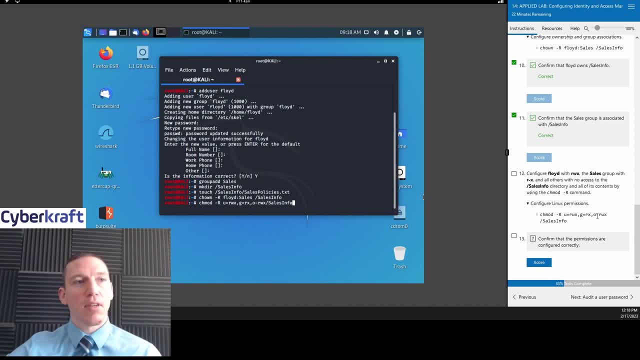 or no? uh, others are going to be, or no, uh, others are going to be without that. so we put that without that. so we put that without that. so we put that at minus rewrite: execute okay. at minus rewrite: execute okay. at minus rewrite: execute okay, so. and then we specify with the slash: 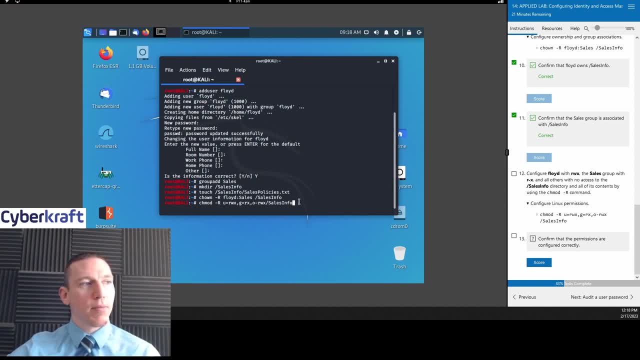 so, and then we specify with the slash so, and then we specify with the slash: sales info, sales info, sales info. the directory. i hope that makes sense. the directory. i hope that makes sense. the directory. i hope that makes sense. if you have any questions, let me know. but 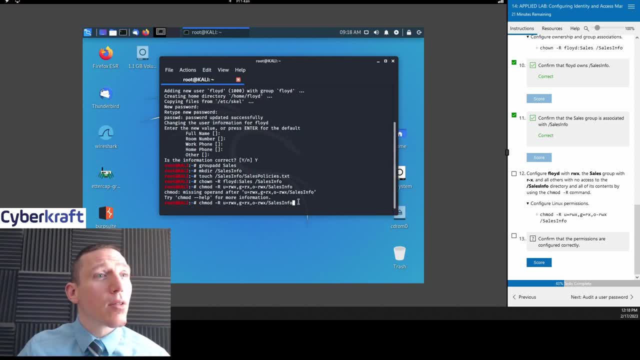 if you have any questions, let me know. but if you have any questions, let me know. but did i mess something up? i think did i mess something up. i think did i mess something up, i think, let's see, let's see, let's see. make sure your spacing is correct, i think. 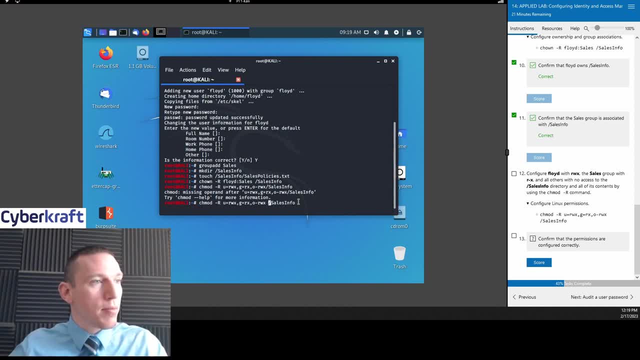 make sure your spacing is correct. i think, make sure your spacing is correct. i think there's a space here. there's a space here. there's a space here. yeah, so there's a space after uh rwx. yeah, so there's a space after uh rwx. 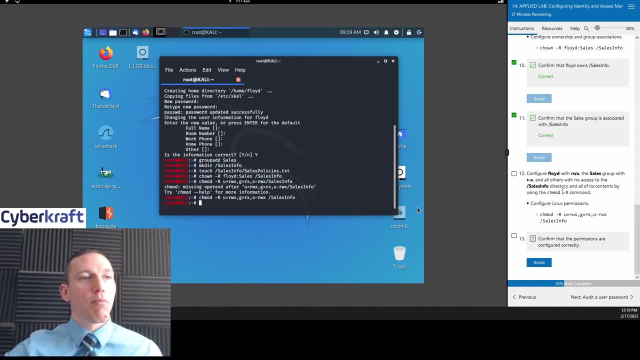 yeah, so there's a space after uh rwx here before sales info. you have to have here before sales info. you have to have here before sales info. you have to have a space before you, a space before you, a space before you specify the directory and then, if we 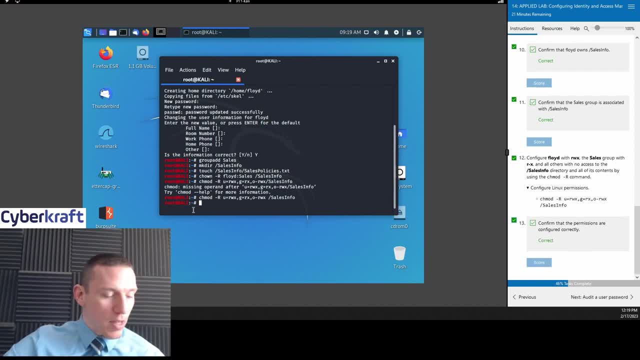 specify the directory. and then, if we specify the directory and then if we score that that should be correct there, score that that should be correct there, score that that should be correct there. so we, uh, we change those permissions. so we, uh, we change those permissions. so we, uh, we change those permissions correctly. 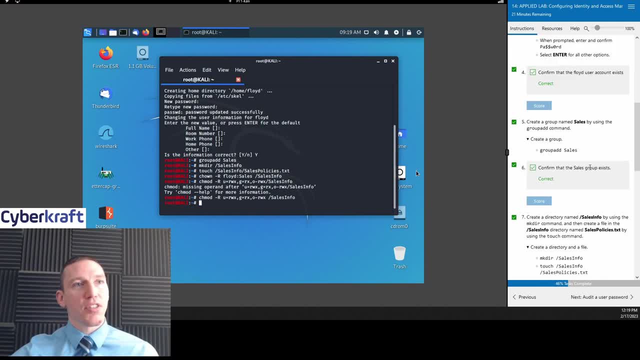 and this is a pretty straightforward i and this is a pretty straightforward i and this is a pretty straightforward, i like this little section. this is just a like this little section. this is just a like this little section. this is just a review on some of these basic linux. 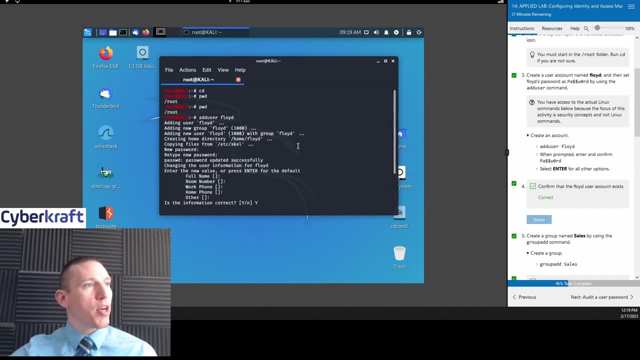 review on some of these basic linux review on some of these basic linux commands that you need to practice with, commands that you need to practice with commands that you need to practice with. so it's a pretty good one. so it's a pretty good one, so it's a pretty good one. and then 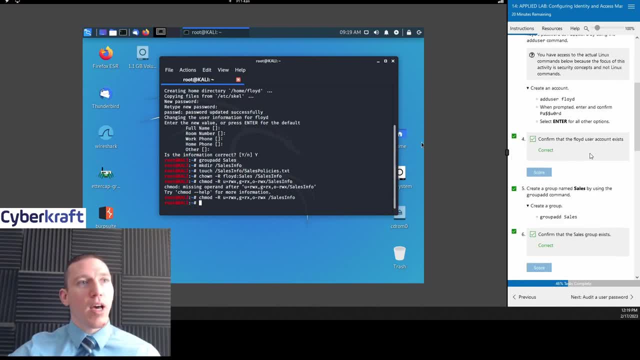 and then, and then, yeah, yeah, yeah, can't really say too much else. i mean can't really say too much else. i mean can't really say too much else. i mean i hope this makes sense what we've done. i hope this makes sense what we've done. 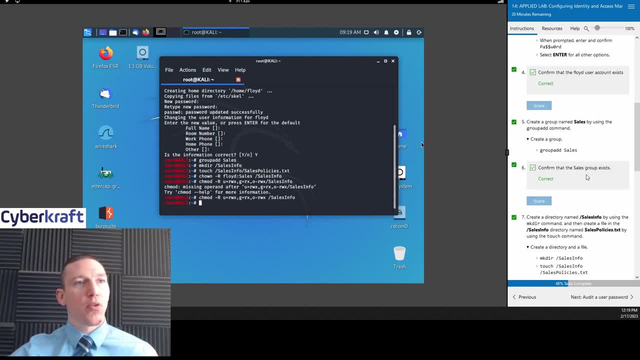 i hope this makes sense what we've done here. we've added floyd as a user. here we've added floyd as a user. here we've added floyd as a user. we created a sales group with group ad. we created a sales group with group ad. 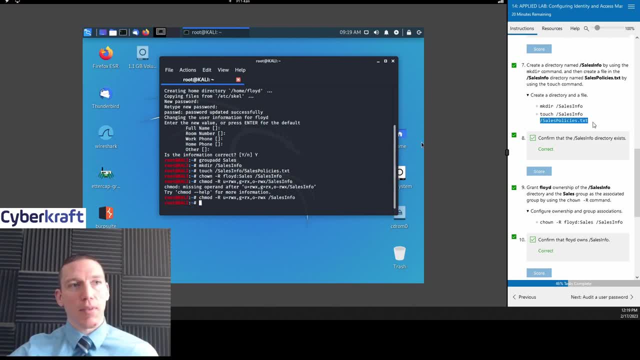 we created a sales group with group ad. we then made a directory called sales. we then made a directory called sales. we then made a directory called sales info. we made a info. we made a info. we made a file in there- a text file okay. file in there, a text file okay. 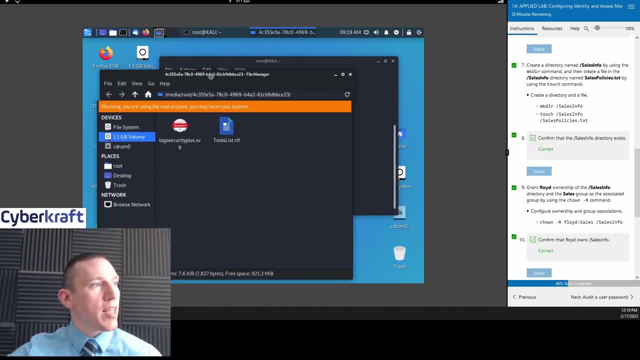 file in there, a text file. okay, uh, uh uh. yeah, you know we can, it's pretty easy. yeah, you know we can, it's pretty easy. yeah, you know we can, it's pretty easy. what we've done here, what we've done here, what we've done here, let's see and go to. 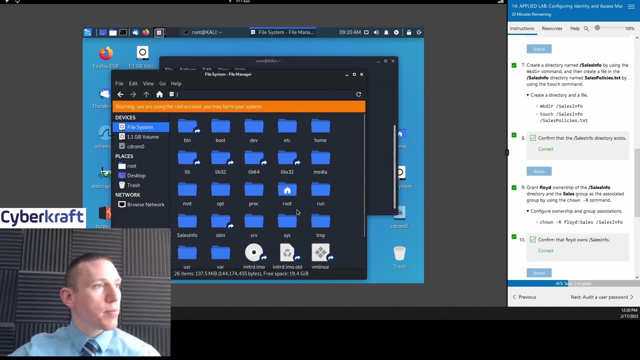 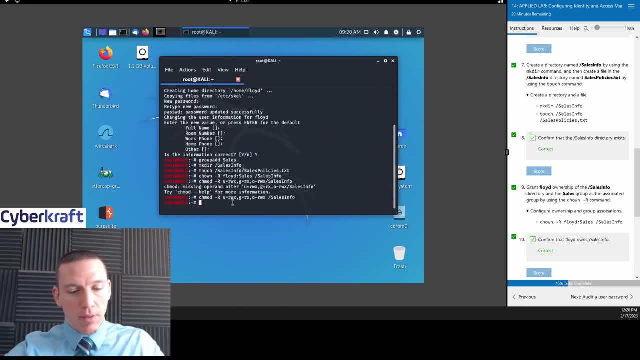 let's see and go to. let's see and go to. let's find our, our stuff here. well, we can, we can just do this through. well, we can, we can just do this through. well, we can, we can just do this through the terminal, the terminal, the terminal. let's see. 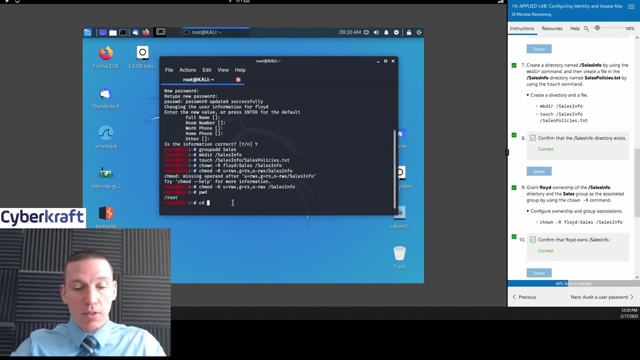 let's see. let's see where are we we're in root? we could. where are we we're in root? we could. where are we we're in root? we could. change directory, change directory. change directory to slash sales info. to slash sales info. to slash sales info. okay. 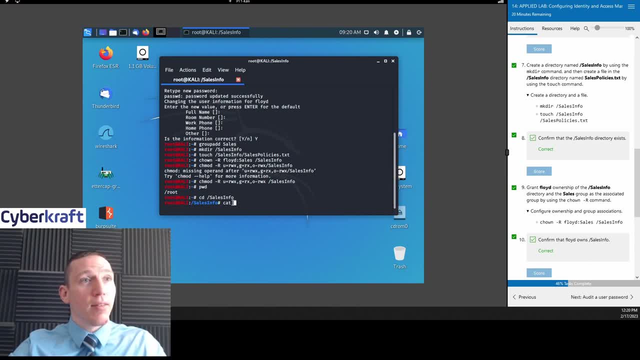 okay, okay, then we could do cat, then we could do cat, then we could do cat, uh, uh uh. sales, sales, sales policy, policy, policy, dot txt, dot txt, dot txt. there's nothing in there. there's nothing in there. there's nothing in there because we didn't. we made the text file. because we didn't we made the text file. because we didn't we made the text file. we didn't put anything in there. we didn't put anything in there. we didn't put anything in there. but you know we've changed the directory. but you know, we've changed the directory. 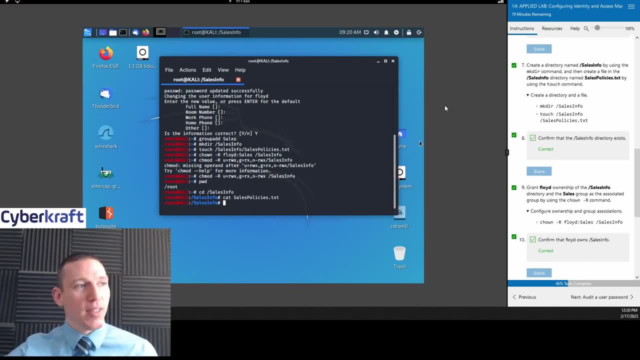 but you know we've changed the directory to that sales info. shows you that that to that sales info. shows you that that to that sales info. shows you that that sales info directory exists, that we sales info directory exists, that we sales info directory exists, that we created. 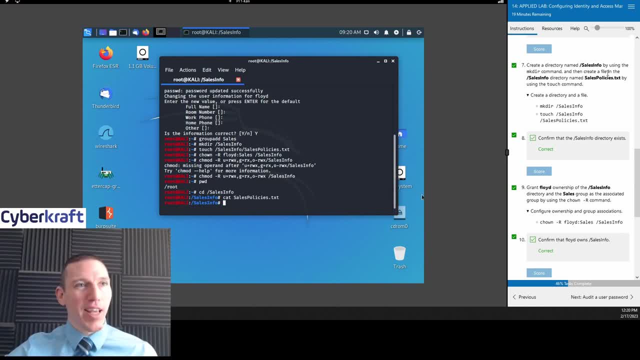 created: created. and then i'm showing the results: the. and then i'm showing the results: the. and then i'm showing the results: the contents of sales policy at txt. with the contents of sales policy at txt. with the contents of sales policy at txt, with the cat command. but there's 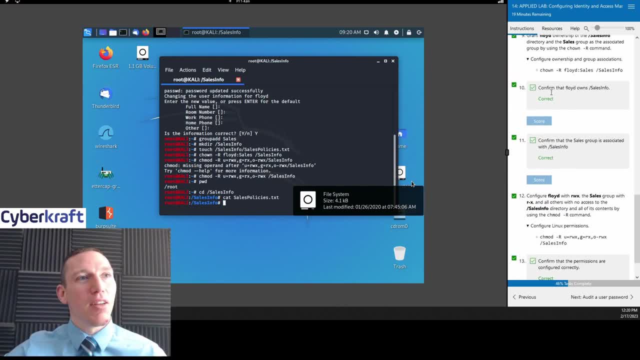 cat command, but there's cat command, but there's. you know there's nothing in that text. you know there's nothing in that text. you know there's nothing in that text box is a blank text. file box is a blank text. file box is a blank text file. but yeah, pretty good, all right, so we've. 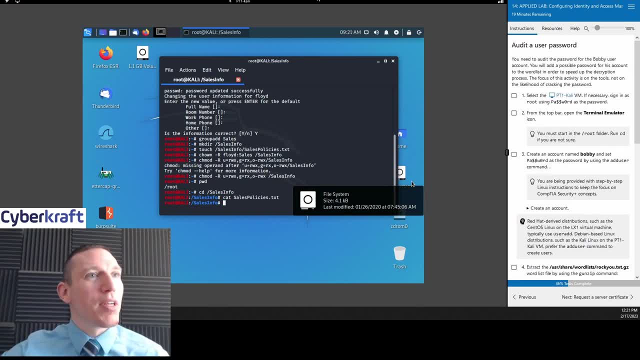 but yeah, pretty good, all right, so we've. but yeah, pretty good, all right, so we've done that. created that user. modify the. done that. created that user, modify the. done that. created that user. modify the permissions looks really good. permissions looks really good. permissions looks really good, okay, okay. well, we're gonna be doing. 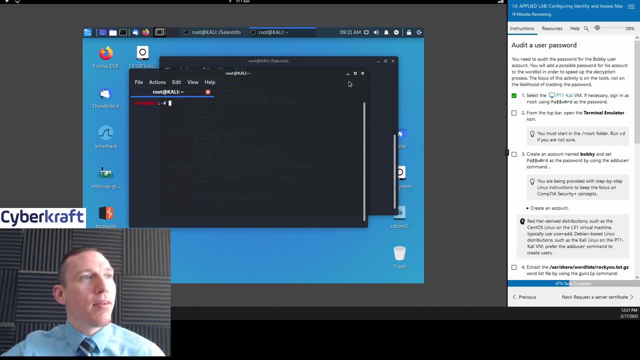 okay, okay, well, we're gonna be doing okay, okay, well, we're gonna be doing. something else in cali here- that's great. something else in cali here, that's great. something else in cali here, that's great. uh, well, i'll put up a fresh terminal. 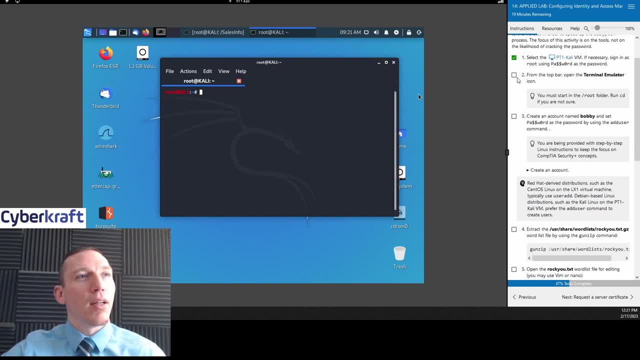 uh well, i'll put up a fresh terminal. uh well, i'll put up a fresh terminal just to make this easier. let's see again we're going to make. let's see again we're going to make. let's see again, we're going to make sure we're in the root folder. 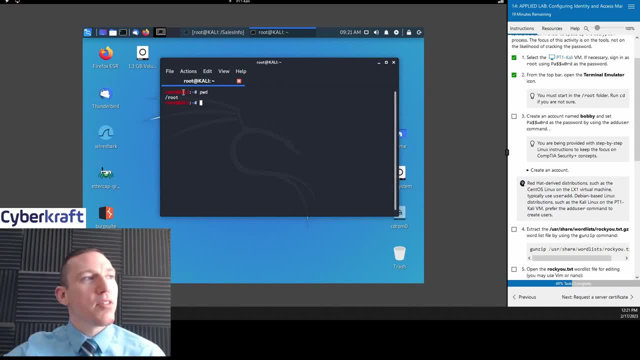 sure we're in the root folder. sure, we're in the root folder. pwd shows you where your root. your pwd shows you where your root. your pwd shows you where your root your directory is and we should be in root. directory is, and we should be in root. 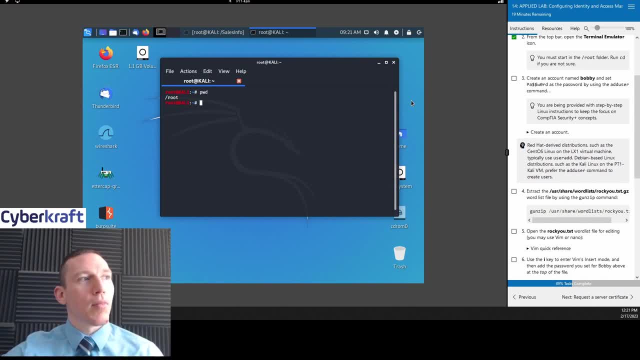 directory is and we should be in root. okay, we can also change directory. we can also change directory. we can also change directory to the root folder cd. to the root folder cd. to the root folder cd: slash. it's going to change you to the slash. it's going to change you to the. 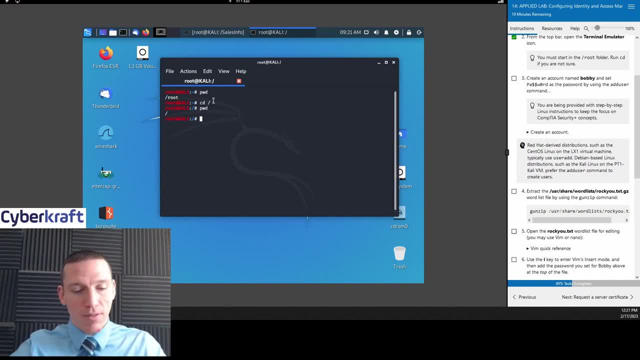 slash. it's going to change you to the root root root account. okay, actually, account. okay, actually, account. okay, actually. that's going to change me to uh slash. that's going to change me to uh slash. that's going to change me to uh slash. slash. root would change us to. 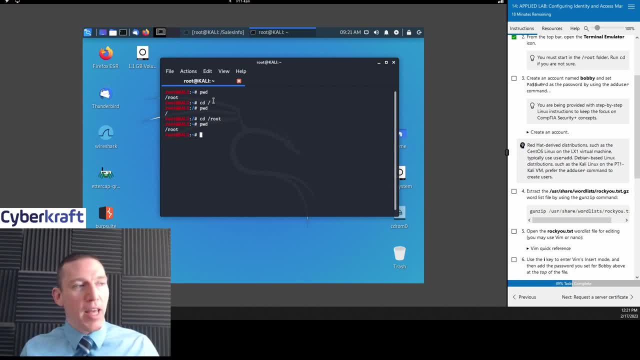 slash root would change us to slash root would change us to root. so now you know you're back in the root. so now you know you're back in the root. so now you know you're back in the flash root. so if you ever need to, just 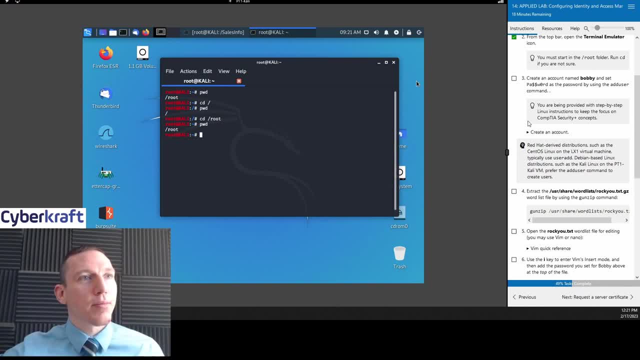 flash root. so if you ever need to just flash root, so if you ever need to just change directory slash root, and you'll change directory slash root and you'll change directory slash root and you'll be back in there. be back in there. be back in there. okay, so now we're gonna uh. 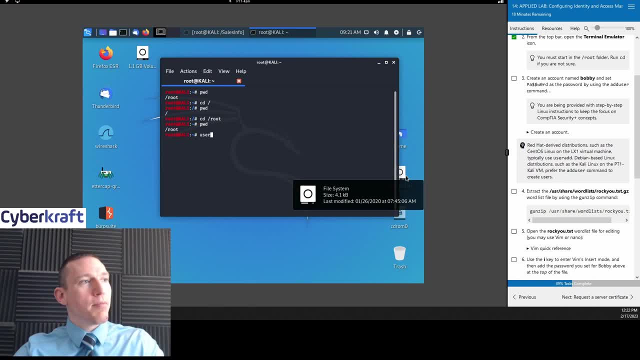 okay. so now we're gonna uh okay. so now we're gonna uh: add user. wait, no, add user. wait. no, add user. wait, no user add bobby user. add bobby user. add bobby. okay, we create bobby. okay, we create bobby. okay, we create bobby. all right, it's add user, right. 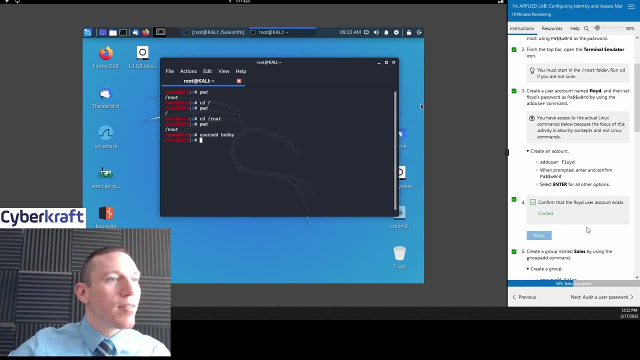 all right, it's add user, right. all right, it's add user. right? i get mixed up too sometimes. let's see, i get mixed up too sometimes. let's see i get mixed up too. sometimes, let's see, it says it says it says add user. it's group ad. add user. add user. 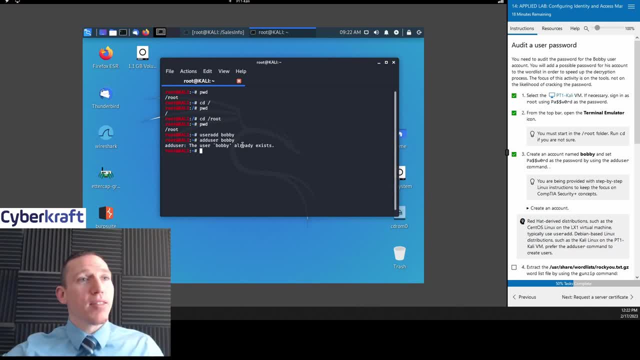 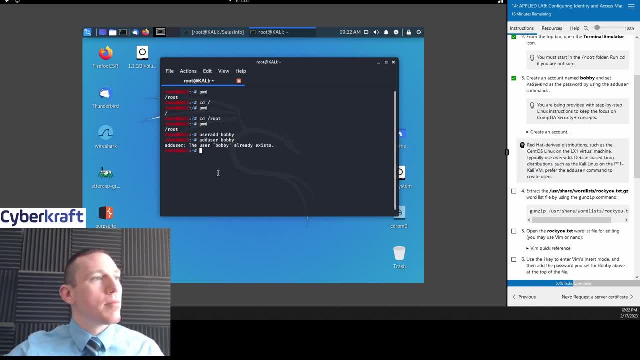 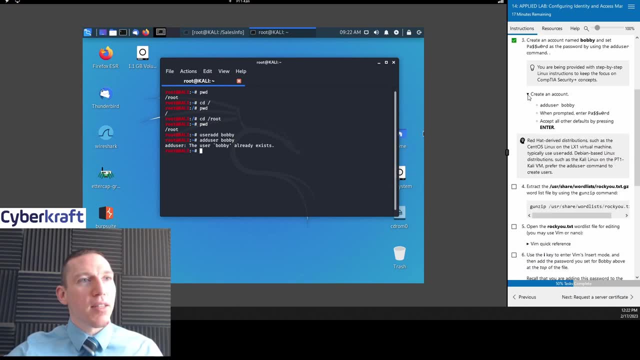 okay, so why is it asking us to add bobby? even says: add user command: all right, bobby already exists here. so all right, bobby already exists here. so all right, bobby already exists here. so he probably already has that password we. he probably already has that password we. 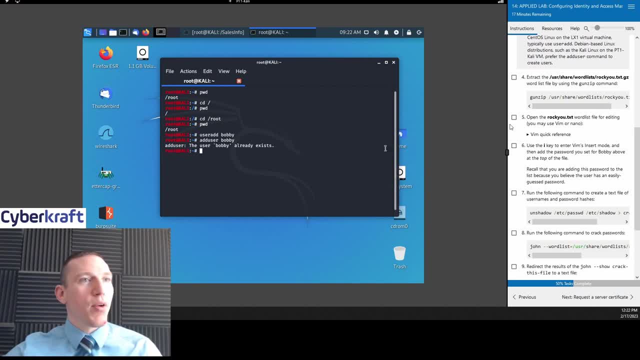 he probably already has that password. we don't have to worry about that. don't have to worry about that. don't have to worry about that, uh, all right. so now we're going to uh. all right. so now we're going to uh. all right. so now we're going to extract a file. 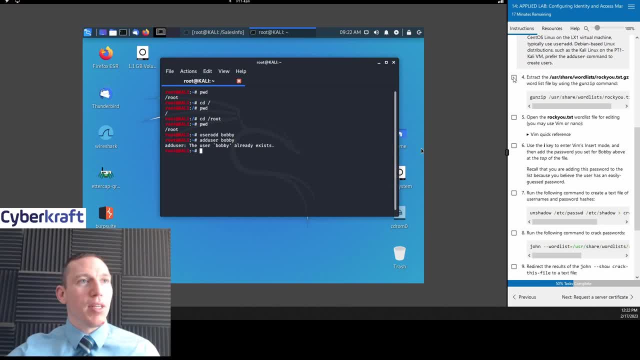 extract a file. extract a file: rockutxtgz. okay. so now we're going to rockutxtgz. okay, so now we're going to rockutxtgz. okay, so now we're going to be. bobby is always the screw up in these. bobby is always the screw up in these. 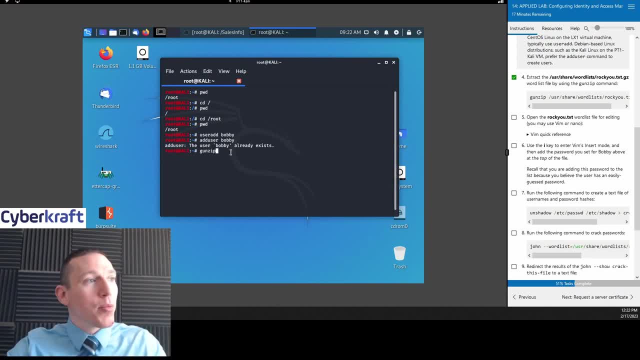 bobby is always the screw up in these scenarios, so he's going to be scenarios. so he's going to be scenarios. so he's going to be opening up some sort of malware. i'm sure opening up some sort of malware. i'm sure opening up some sort of malware. i'm sure we're going to do that with a gun zip. 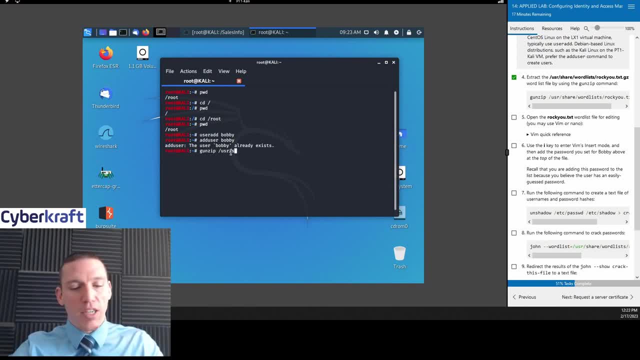 we're going to do that with a gun zip. we're going to do that with a gun zip. command, gun, zip, slash, command, gun, zip, slash, command, gun, zip, slash, usr, slash, share, usr, slash, share, usr, slash, share, slash word lists, slash word lists. slash word lists, slash rocku dot txt. 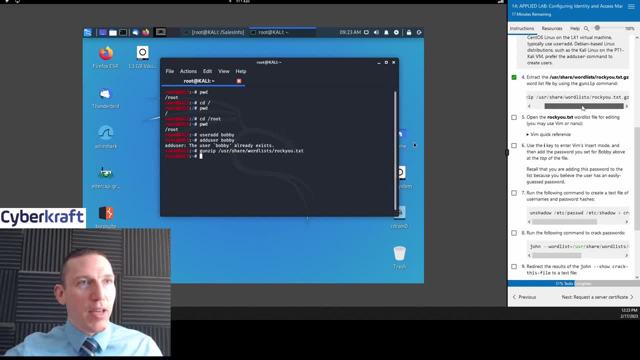 slash rocku dot txt. slash rocku dot txt. now, this might not be a malware. this, now, this might not be a malware. this, now, this might not be a malware. this might just be a list of passwords, oh no, might just be a list of passwords, oh no. 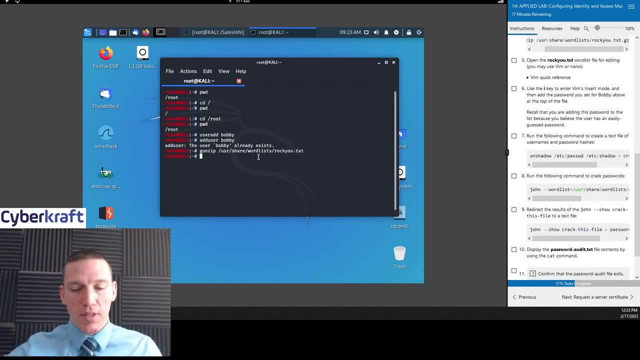 might just be a list of passwords. oh no, txtgz it's going to be gz. that's why txtgz it's going to be gz. that's why txtgz it's going to be gz. that's why we're using the guns up command. we're using the guns up command. 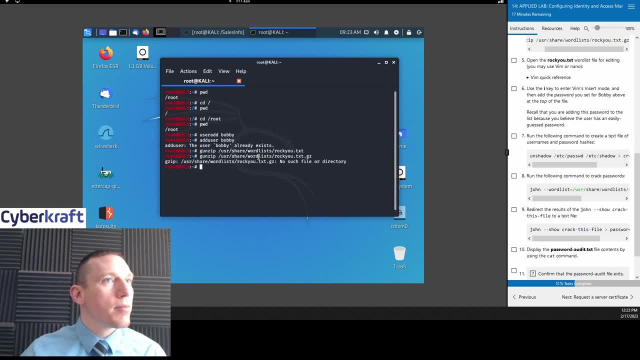 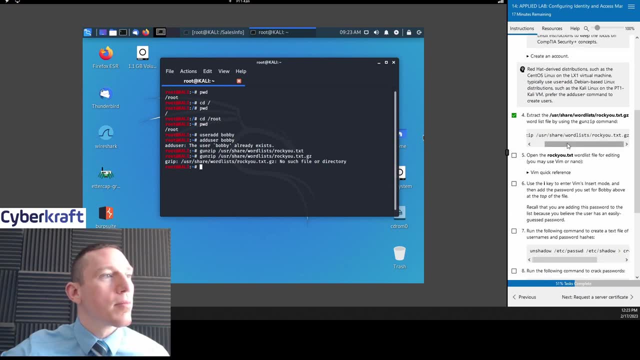 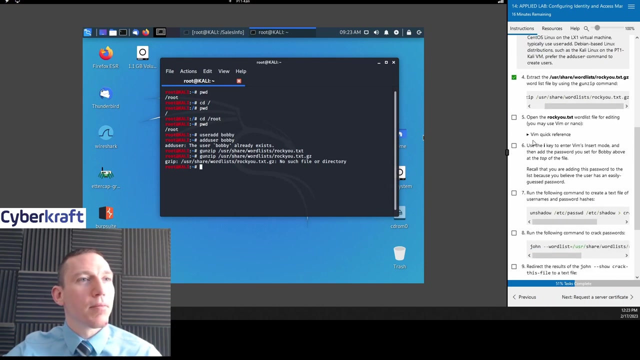 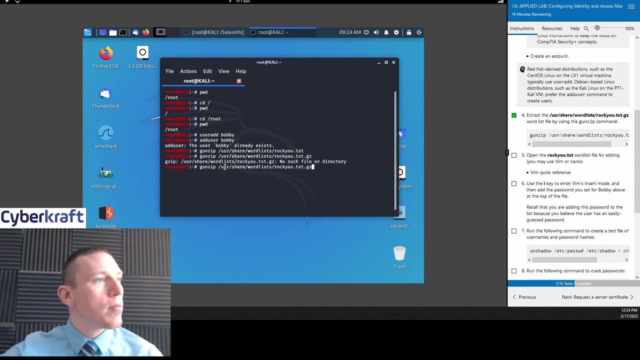 we're using the guns up command jot gz. okay, no such file or directory exists. let me verify that i type this correctly: arcutxtgz. hmm, i think i typed that correctly. user. i think i typed that correctly. user. i think i typed that correctly. user- share wordless. 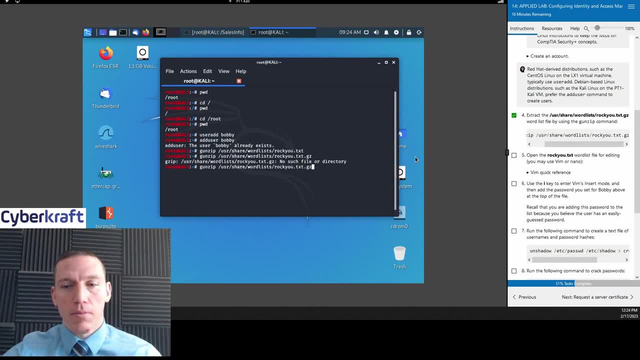 share wordless, share, wordless, slash. rock you dot txt. yeah, this is a 601 lab. yep, this is identity access management. huh, that should work, but it's not working. let's take a look in the directory there. okay, there, so we're navigating to the directory. we see rock you dot. 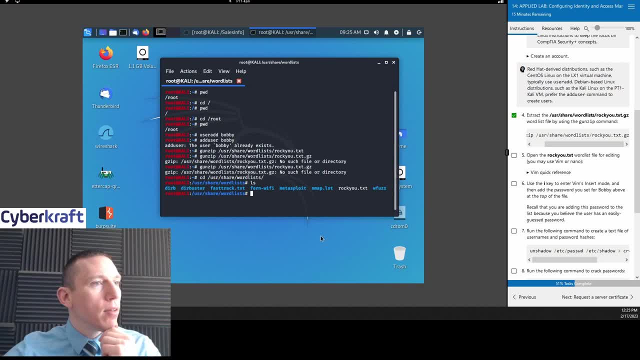 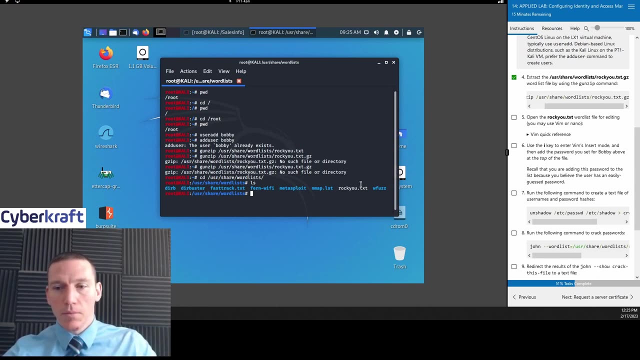 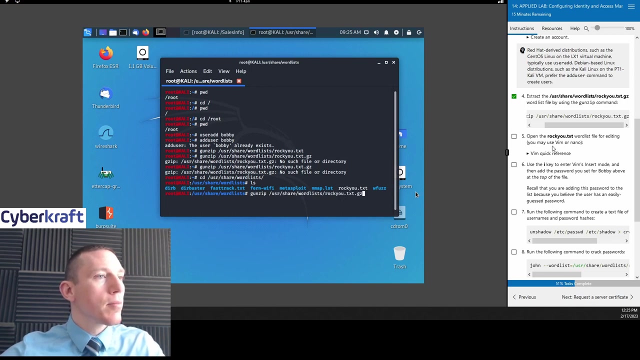 txt. so we're navigating to the directory. we see rock you dot txt. okay there. so we're navigating to the directory. we see rock you dot txt. why is this not working? yeah, yeah, that's good advice, uh-huh. yeah, yeah, that's good advice, uh-huh. 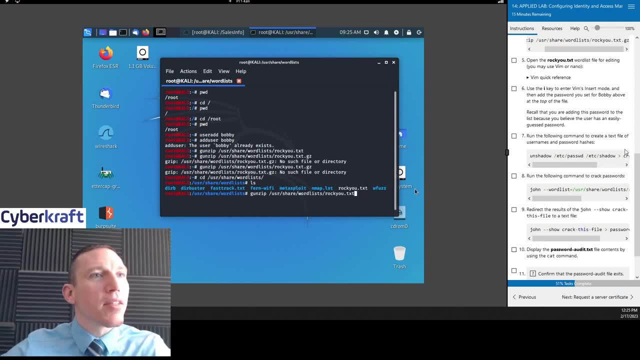 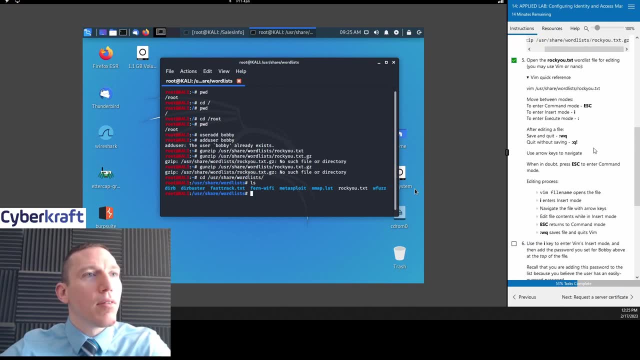 i think it's already extracted. i think it's already extracted. i think it's already extracted, because now it's a txt file. so because now it's a txt file, so because now it's a txt file. so, honestly, i think we should be okay. all right, let's just try and work with. 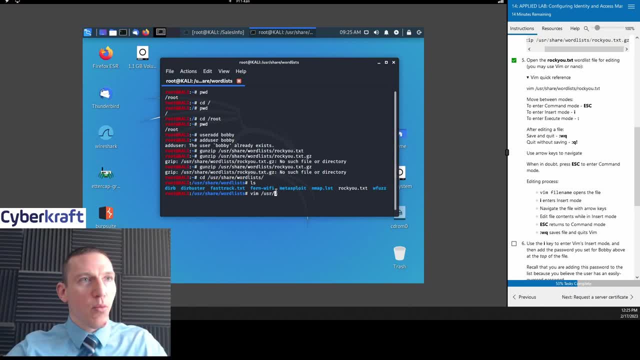 all right, let's just try and work with. all right, let's just try and work with it, it, it. i think there's some things. i think this, i think there's some things, i think this. i think there's some things. i think this one's not written very well. 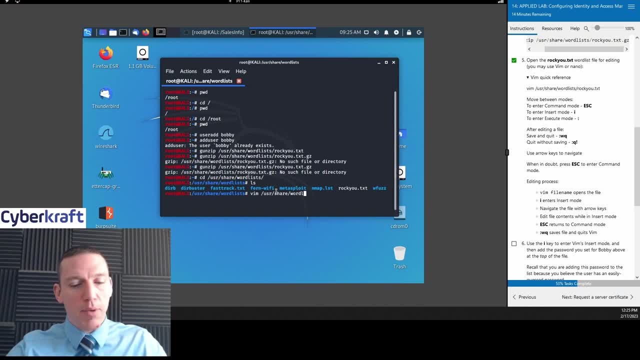 one's not written very well. one's not written very well because- because, because i think this was already extracted and i think this was already extracted, and i think this was already extracted and bobby was already created. bobby was already created. bobby was already created in this version, so they probably 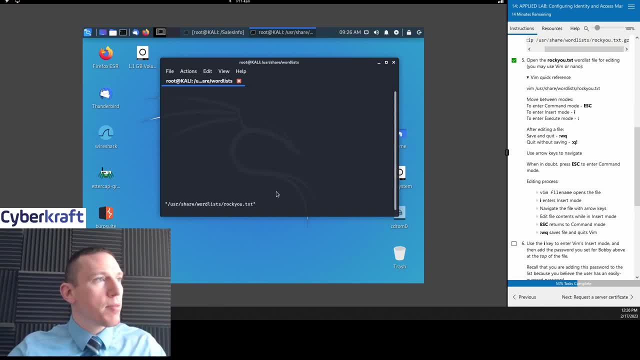 in this version. so they probably in this version. so they probably probably saved the wrong image. probably saved the wrong image, probably saved the wrong image. okay, okay, okay, all right. so, yeah, this was already all right. so yeah, this was already all right. so, yeah, this was already extracted, so we 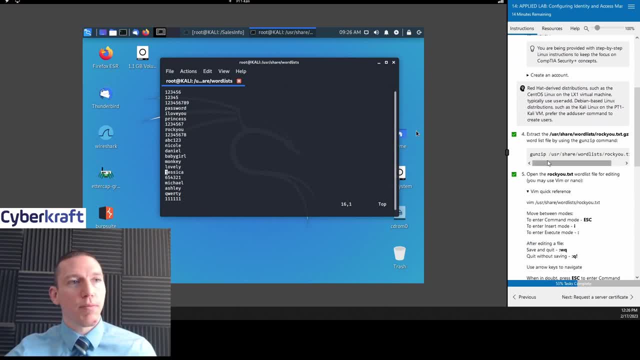 extracted, so we extracted, so we. if you're going through a slab, skip the. if you're going through a slab, skip the. if you're going through a slab, skip the. gun zip number four. gun zip number four. gun zip number four. now, this would be if this was still in. 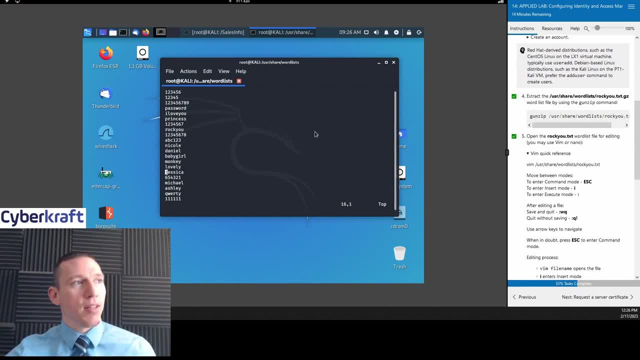 now this would be if this was still in now. this would be if this was still in a archive format. a archive format, a archive format, but it isn't it's. you know when we went, but it isn't it's. you know when we went, but it isn't it's. you know when we went through the list. 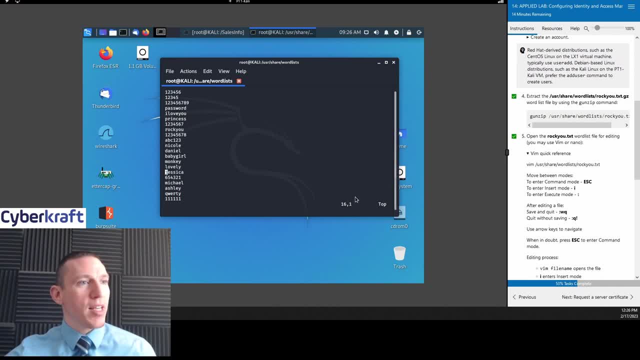 through the list, through the list command the ls command. we saw that command, the ls command. we saw that command, the ls command. we saw that rockutxt was rockutxt was. rockutxt was already extracted, so we don't need to do. already extracted, so we don't need to do. 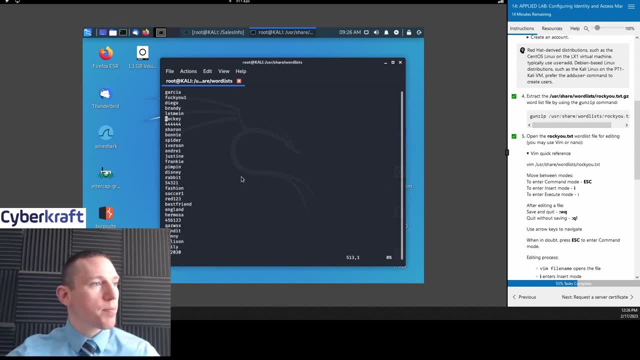 already extracted, so we don't need to do that. now we have a list of passwords. that now we have a list of passwords. that now we have a list of passwords. essentially, that's what we're doing here. okay, it's a pretty long list of. okay, it's a pretty long list of. 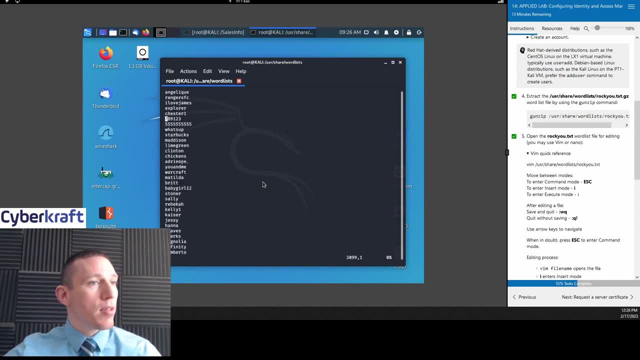 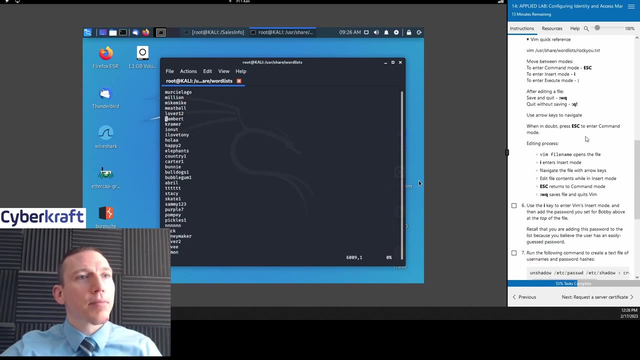 okay, it's a pretty long list of passwords. okay, okay, okay, okay. so now it's going to. so, now it's going to. so now it's going to ask us to, i think, edit something. ask us to, i think, edit something. ask us to, i think, edit something. now we're using vim uh to to edit this. 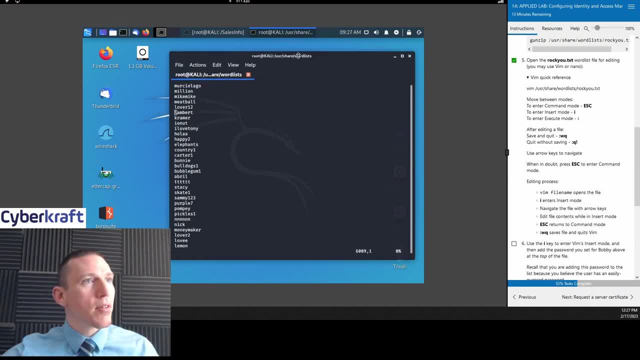 now we're using vim uh to to edit this. now we're using vim uh to to edit this. just a utility within just a utility within just a utility within cali linux, within cali linux, within cali linux, within most uh ubuntu or debian, most uh ubuntu or debian. 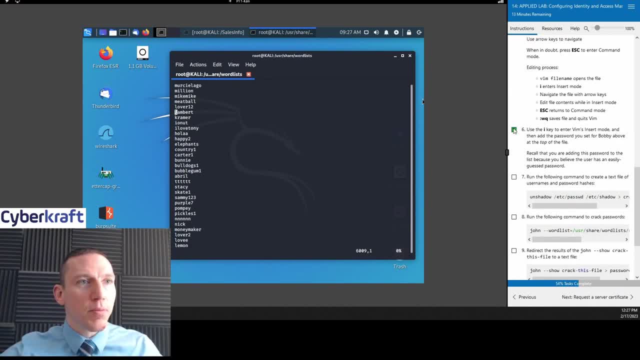 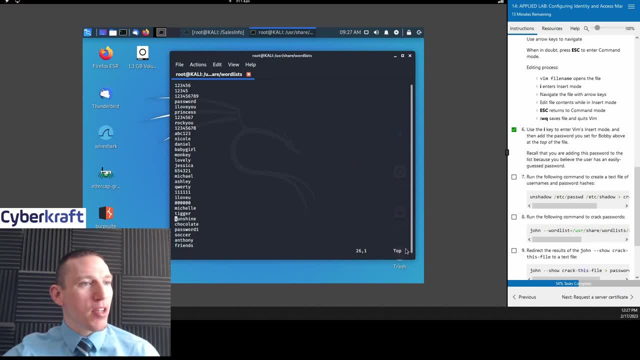 top. it's just going to speed things up top. it's just going to speed things up if it's at the top. if it's at the top, if it's at the top, okay, and you could also anyway. okay, and you could also anyway. okay, and you could also anyway. so we're gonna go, uh, click here, we're. 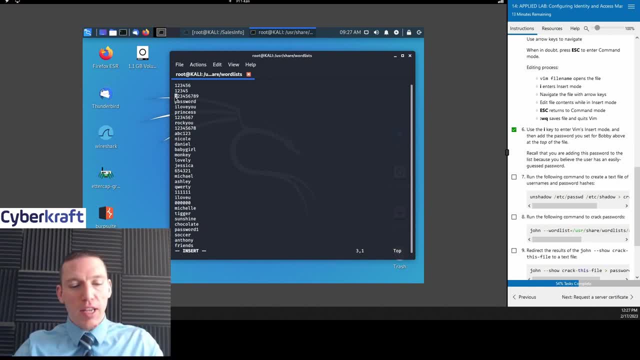 so we're gonna go uh click here. we're so we're gonna go uh click here. we're gonna. i gonna, i gonna, i insert. we're gonna insert. insert bobby's password. i'm just gonna insert bobby's password. i'm just gonna insert bobby's password. i'm just gonna delete this other password. 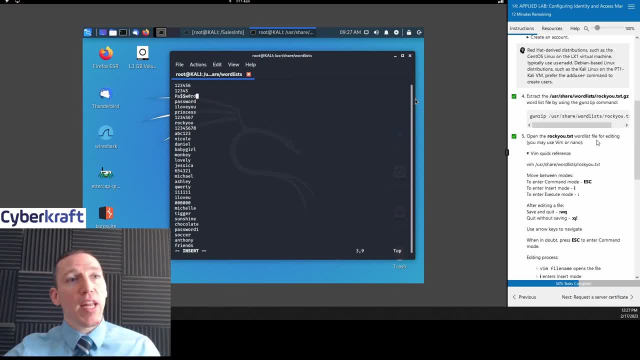 delete this other password. delete this other password. we don't need it. so this is the password. we don't need it. so this is the password. we don't need it. so this is the password for bobby, even though we didn't create for bobby, even though we didn't create. 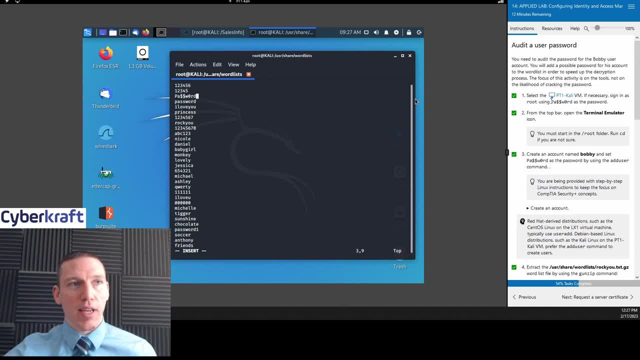 for bobby, even though we didn't create bobby bobby. bobby bobby was already created. i'm sure that he was already created. i'm sure that he was already created. i'm sure that he is created using a default password. is created using a default password. 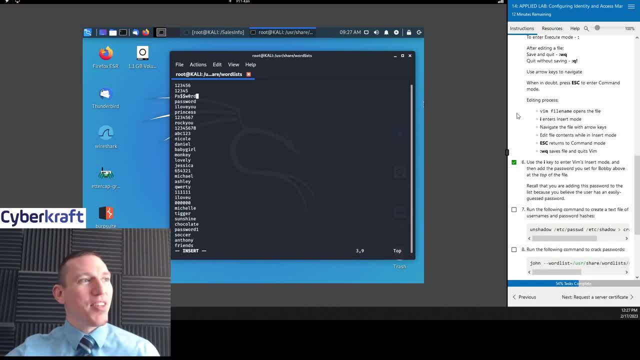 is created using a default password. i would stake my entire career on that. i would stake my entire career on that. i would stake my entire career on that with these labs. that's the only password with these labs. that's the only password with these labs. that's the only password they ever, ever use. 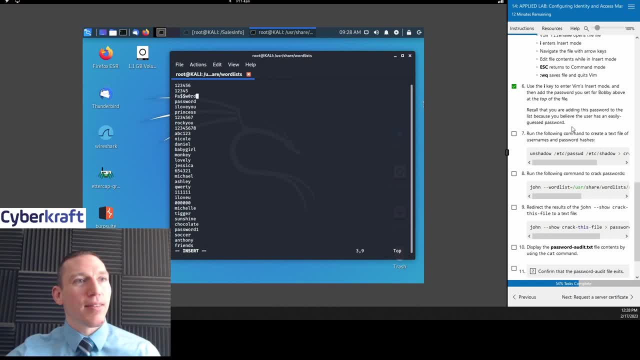 they ever ever use. they ever ever use. okay, so we're gonna go ahead. uh, okay, so we're gonna go ahead. uh, okay, so we're gonna go ahead. uh, yeah, we're adding this password list. yeah, we're adding this password list. yeah, we're adding this password list because believe the user has an easily. 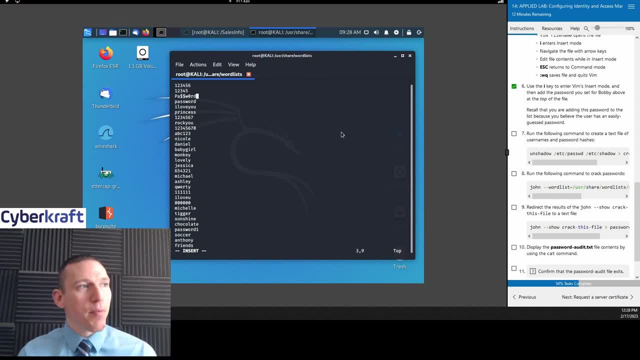 because believe the user has an easily, because believe the user has an easily guessed password. so basically, right now guessed password. so basically, right now guessed password. so basically, right now, in this scenario. it's not explaining it in this scenario. it's not explaining it in this scenario. it's not explaining it very well. 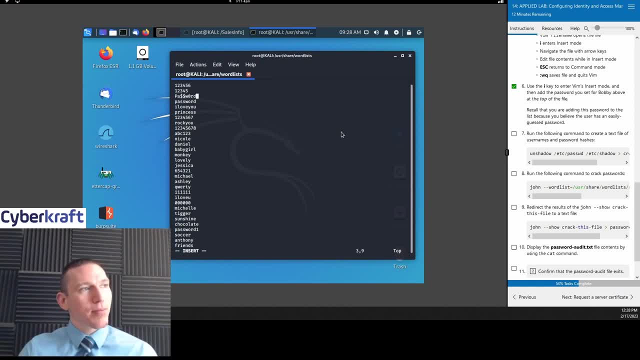 very well, very well. is we're acting as a hacker? is we're acting as a hacker? is we're acting as a hacker? we're going to be using a word list to. we're going to be using a word list to. we're going to be using a word list to help us crack. 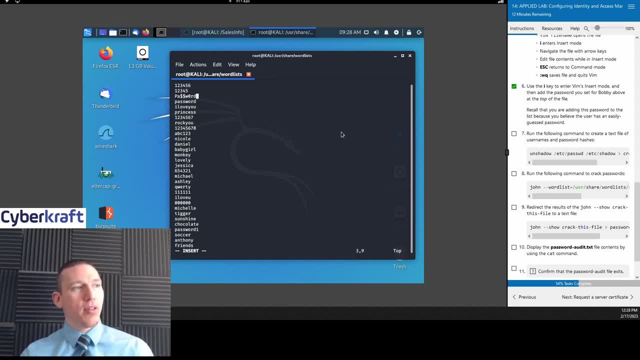 help us crack. help us crack a password okay and a password okay and a password okay and we're. this is a list of words that we we're. this is a list of words that we we're. this is a list of words that we have have have. this is like a dictionary or a rainbow. 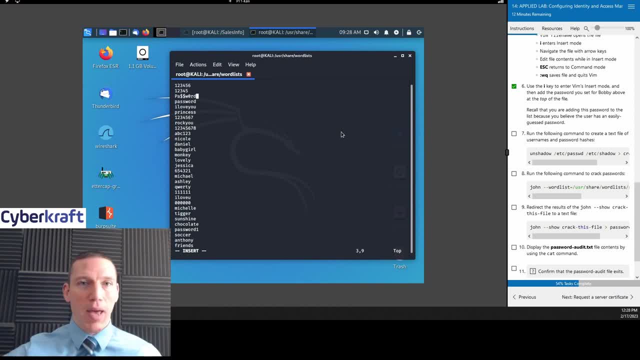 this is like a dictionary or a rainbow. this is like a dictionary or a rainbow table we might have table. we might have table we might have that we're using to crack the passwords that we're using to crack the passwords that we're using to crack the passwords of. 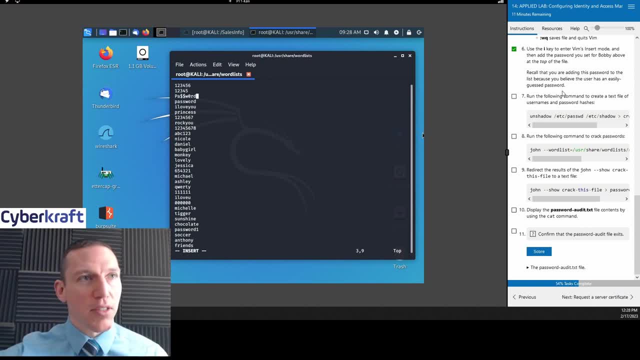 of of. you know say we got a list of hashes. you know say we got a list of hashes. you know say we got a list of hashes. we're trying to crack those password. we're trying to crack those password. we're trying to crack those password hashes. 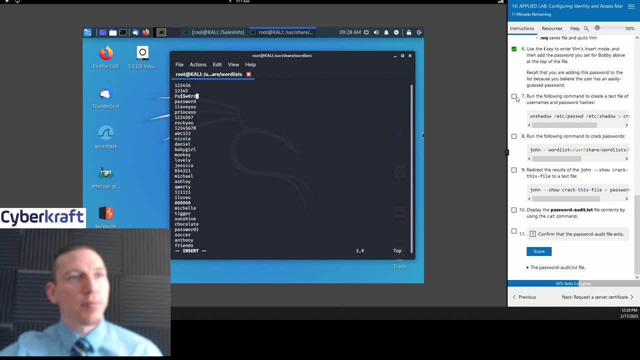 hashes, hashes, so we've, we've found those. um, so we've, we've found those. um, so we've, we've found those. um those password hashes, and now we're those password hashes. and now we're those password hashes, and now we're trying to, trying to. 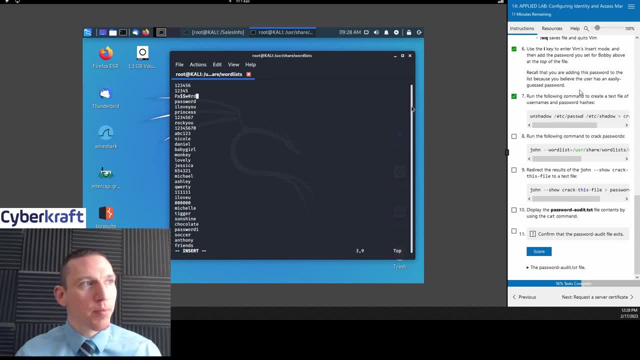 trying to match those hashes to plain text. match those hashes to plain text. match those hashes to plain text. passwords that we have, passwords that we have, passwords that we have. so we're gonna go ahead and let's see. so we're gonna go ahead and let's see. 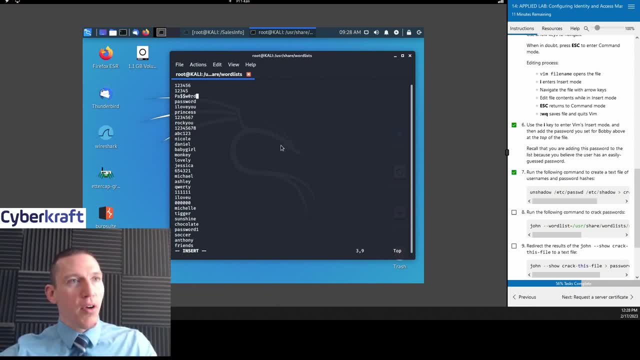 so we're gonna go ahead and let's see, we've inserted that, we've inserted that, we've inserted that, uh, we're gonna go ahead and escape. uh, we're gonna go ahead and escape. uh, we're gonna go ahead and escape, okay, and then we're gonna do: 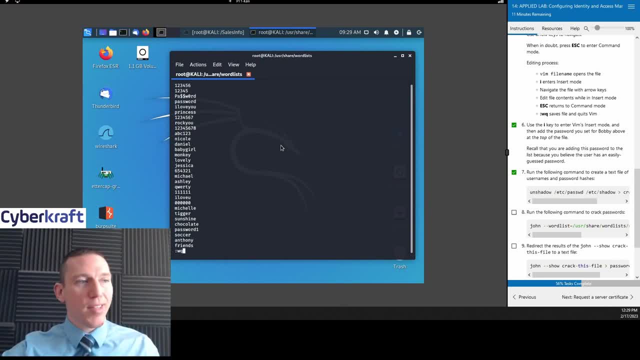 okay, and then we're gonna do okay, and then we're gonna do colon, colon, colon, wq. wq is gonna save and quit wq. wq is gonna save and quit wq. wq is gonna save and quit vim. and there, so we've saved, we've quit. 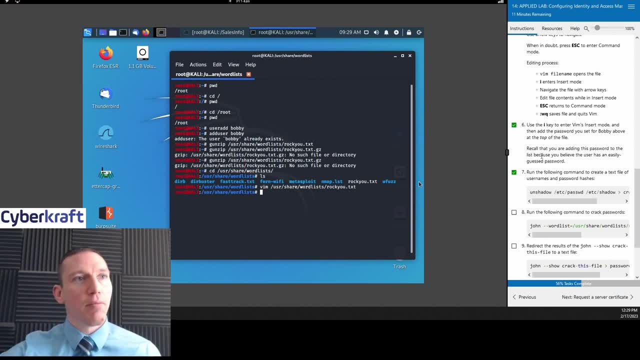 vim and there, so we've saved, we've quit vim and there, so we've saved, we've quit vim. and now rockutxt should be vim and now rockutxt should be vim. and now rockutxt should be modified. should have that, uh that modified. should have that, uh that. 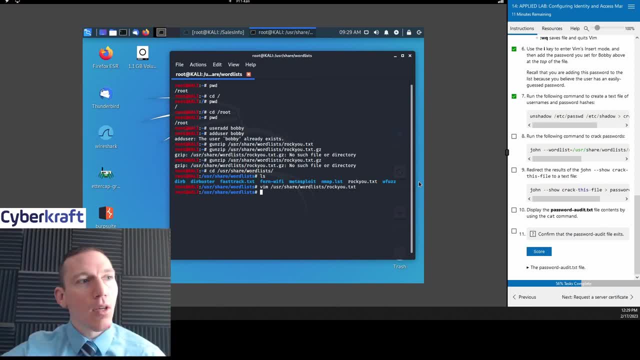 modified. should have that, uh, that bobby's password in there. a great question. this is a virtual. a great question. this is a virtual, a great question. this is a virtual machine. machine machine through comptia, when you sign up for through comptia, when you sign up for 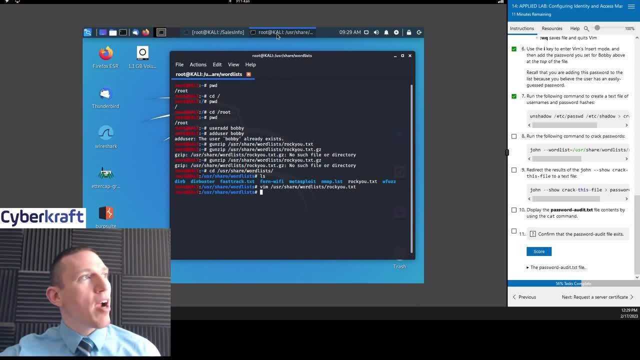 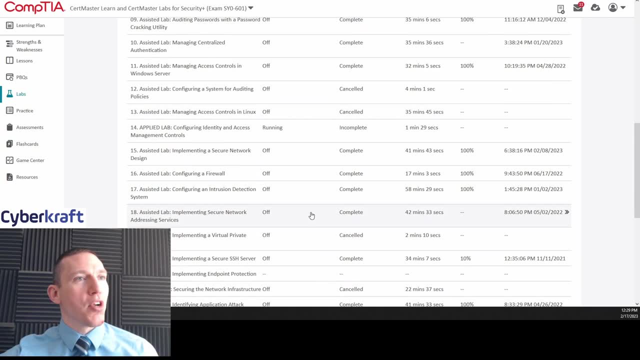 through comptia. when you sign up for any of my courses, you get access to the. any of my courses, you get access to the any of my courses, you get access to the the lab environment with comptia and the lab environment with comptia and the lab environment with comptia and labs for security plus. we're doing lab. 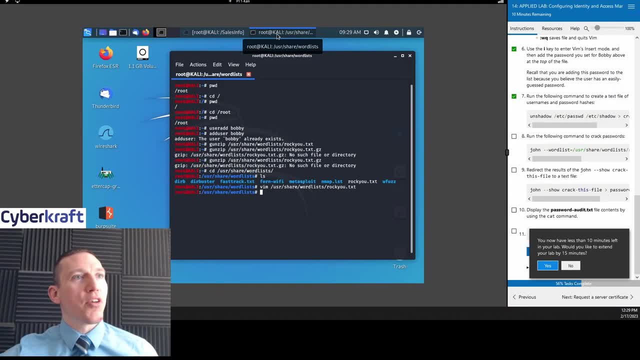 labs for security plus. we're doing lab labs for security plus. we're doing lab 14 here, 14 here, 14 here. so this is all browser based, you don't? so this is all browser based, you don't? so this is all browser based. you don't have to install anything. have to install anything. have to install anything, though, also when you sign up for a course. though, also when you sign up for a course, though also when you sign up for a course, i always to also teach you how to make. i always to also teach you how to make. 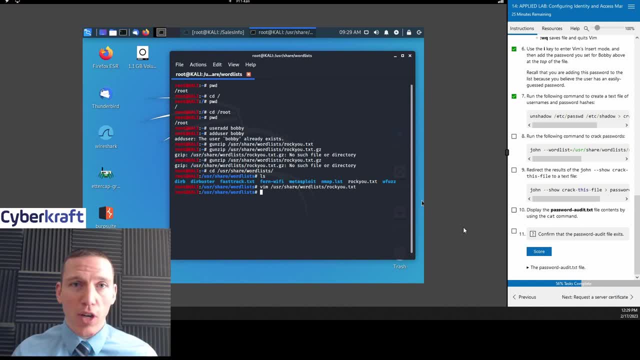 i always to also teach you how to make your own lab environment like this. if your own lab environment like this, if your own lab environment like this, if you're interested in doing that, go to. you're interested in doing that, go to. you're interested in doing that, go to cybercrafttrainingcom. 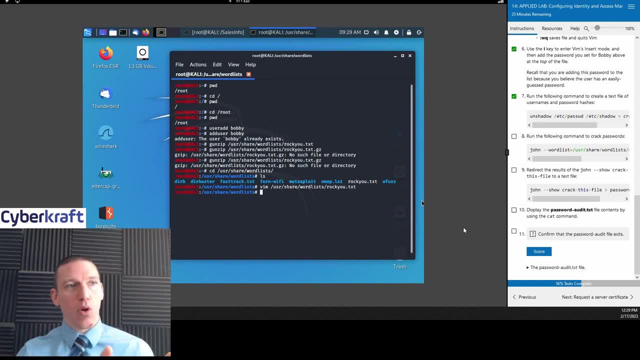 cybercrafttrainingcom. i got a home lab course. it's a few hours. i got a home lab course. it's a few hours. i got a home lab course. it's a few hours long. teaches you how to make your own. long teaches you how to make your own. 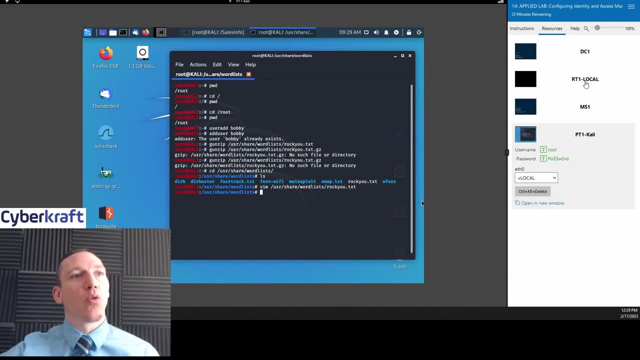 long teaches you how to make your own lab environment like this one lab environment like this one lab environment like this one linked with a domain controller: one ms1. linked with a domain controller: one ms1. linked with a domain controller: one ms1- dc1. all that. 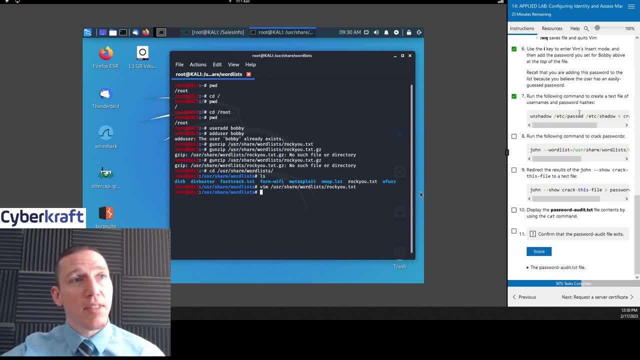 dc1, all that, dc1, all that. so a great question. um you can easily set. so a great question. um you can easily set. so a great question. um you can easily set. well, it's not super easy, it takes. well, it's not super easy, it takes. 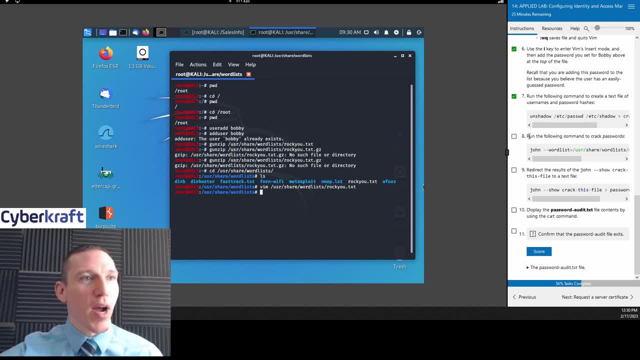 well, it's not super easy. it takes several hours, but you can set up a lab several hours, but you can set up a lab several hours, but you can set up a lab environment like this on your own and environment like this on your own and environment like this on your own, and practice these things. 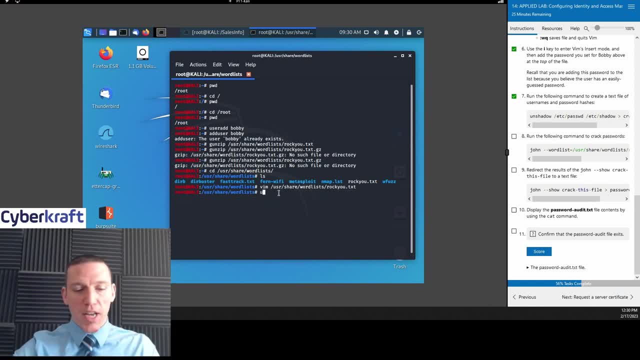 practice these things. practice these things, okay, okay. so now, what we're doing is okay, okay. so now, what we're doing is okay, okay. so now what we're doing is: we're using the unshadow command. we're using the unshadow command. we're using the unshadow command, okay. a password is known to be shadowed. 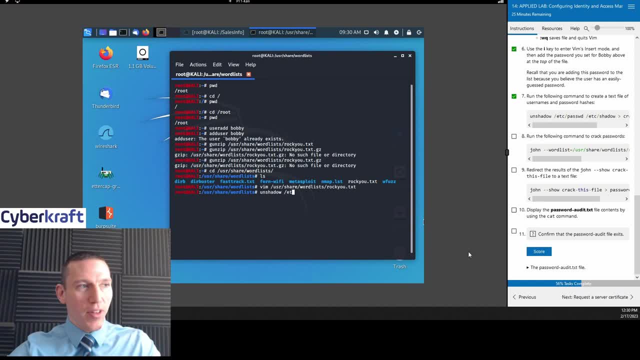 okay, a password is known to be shadowed. okay, a password is known to be shadowed when it's encrypted, when it's secure, when it's encrypted, when it's secure, when it's encrypted, when it's secure. and we're gonna unshadow that using the. 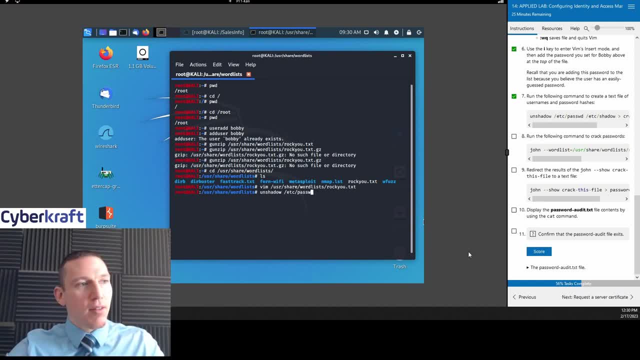 and we're gonna unshadow that using the. and we're gonna unshadow that using the unshadow command. unshadow command, unshadow command. so we're gonna make it. uh, we're gonna. so we're gonna make it. uh, we're gonna. so we're gonna make it. uh, we're gonna decrypt it, so we're new. 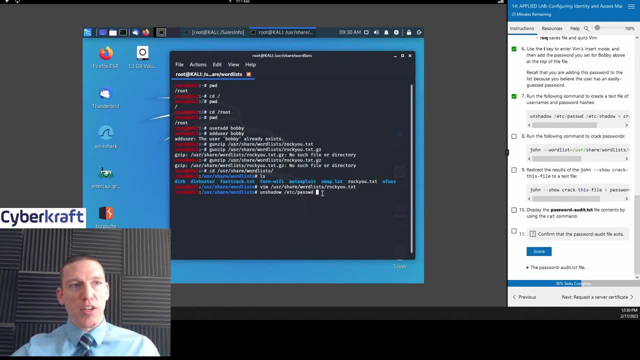 decrypt it. so we're new. decrypt it. so we're new in the slash etc. password file. that's in the slash etc. password file. that's in the slash etc. password file. that's where you'll find your password, where you'll find your password, where you'll find your password. slash etc. slash shadow. 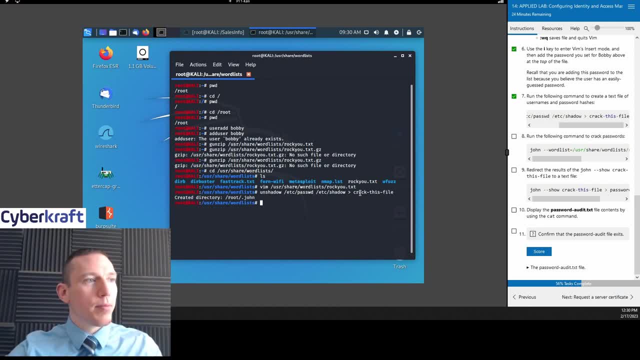 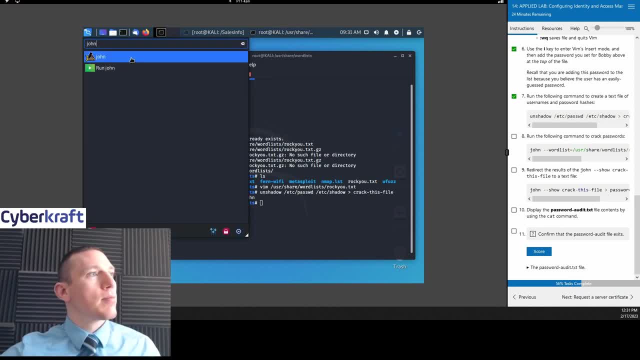 to do this. john the ripper is one of to do this. john the ripper is one of these utilities. within cali winix, we can open john the ripper like this: we can open john the ripper like this: we can open john the ripper like this, but we're just doing it through the. 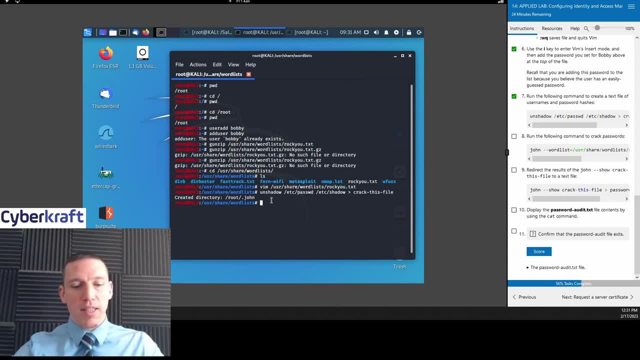 but we're just doing it through the, but we're just doing it through the terminal commands, okay, terminal commands, okay, terminal commands, okay, so, so. so, the syntax for john the ripper is john, the syntax for john the ripper is john. the syntax for john the ripper is john. double dash. 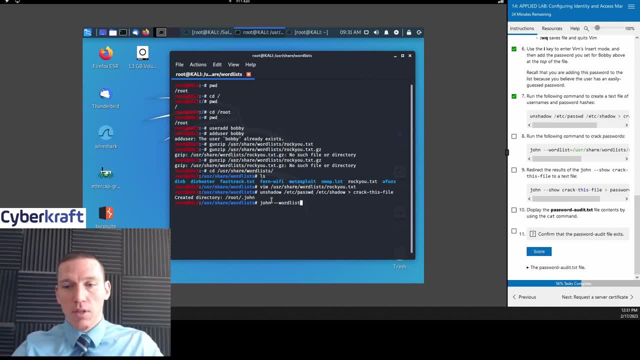 double dash, double dash. we're going to specify a word list to. we're going to specify a word list to. we're going to specify a word list to use, and then, and then, and then. we're going to hit equal. we're going to hit equal. we're going to hit equal. slash the user. 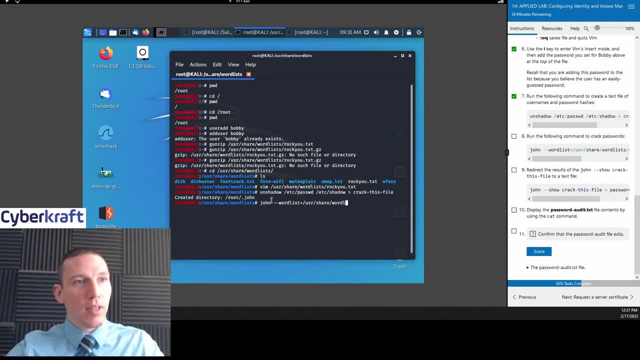 share share share, slash word, slash word, slash word lists. we're just specifying the directory lists. we're just specifying the directory lists. we're just specifying the directory where that word list is. word list, slash word list, slash word list, slash rock you dot txt. now we're specifying. 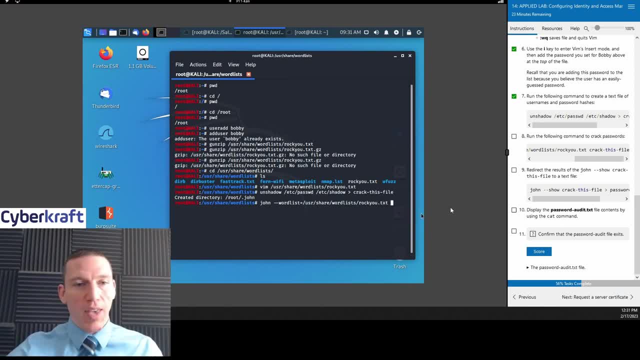 rock you dot txt. now we're specifying: rock you dot txt. now we're specifying that, that that rock you dot txt. uh word list that we had. rock you dot txt. uh word list that we had. rock you dot txt. uh word list that we had already. that we've modified. 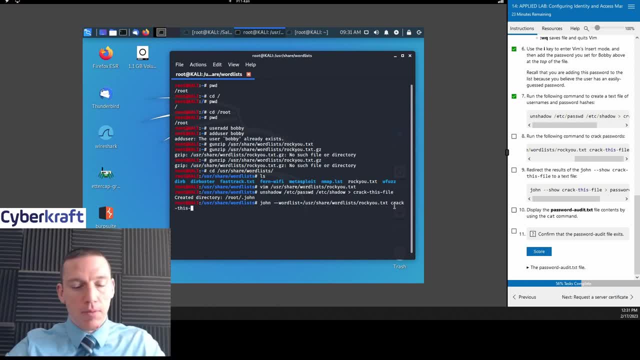 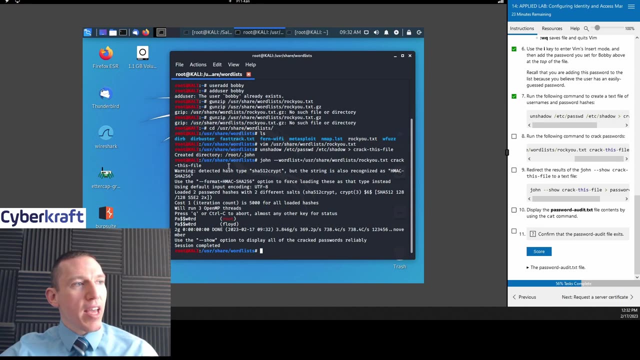 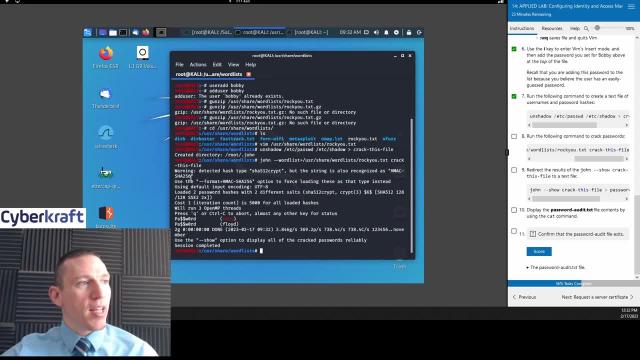 so we've detected a hash. so we've detected a hash. i'm going to read this from top bottom. i'm going to read this from top bottom. i'm going to read this from top bottom: this output so you can understand it. this output so you can understand it. 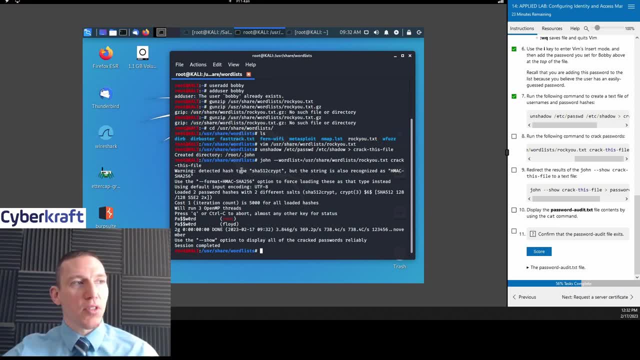 this output so you can understand it. warning detected hash type: sha 512. warning detected hash type: sha 512. warning detected hash type: sha 512 crypt. okay, so this is a secure hashing crypt. okay, so this is a secure hashing crypt. okay, so this is a secure hashing algorithm. 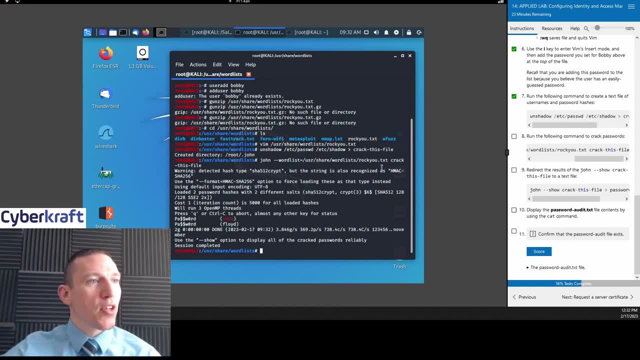 algorithm. algorithm: 512, 512, 512, 512, 512 bits there, but the bits there, but the bits there. but the string is also rage. recognizes h mac string is also rage. recognizes h mac string is also rage. recognizes h mac. sha 256, okay so. sha 256, okay so. 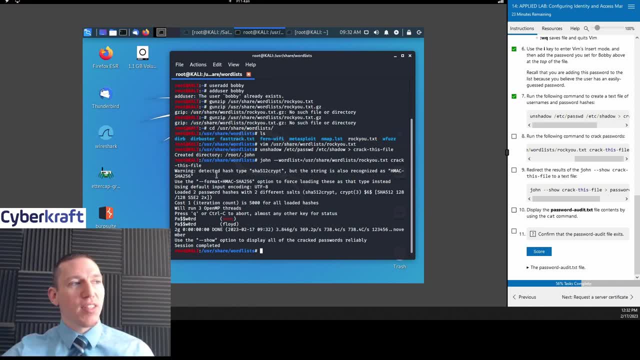 sha 256 okay. so, uh, it's probably a sha secure hashing. uh, it's probably a sha secure hashing. uh, it's probably a sha secure hashing. algorithm 256 bit hash- okay. algorithm 256 bit hash, okay. algorithm 256 bit hash- okay, hmac hash, hmac hash. 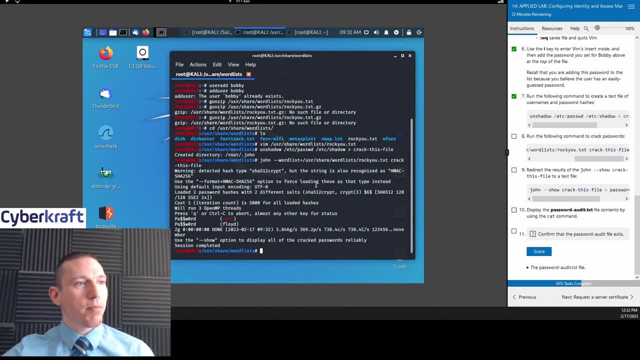 hmac hash. so it uses, so it uses, so it uses the sha 256 option, the sha 256 option, the sha 256 option. so john the ripper is trying to identify. so john the ripper is trying to identify. so john the ripper is trying to identify what hashes it's looking at, it thinks 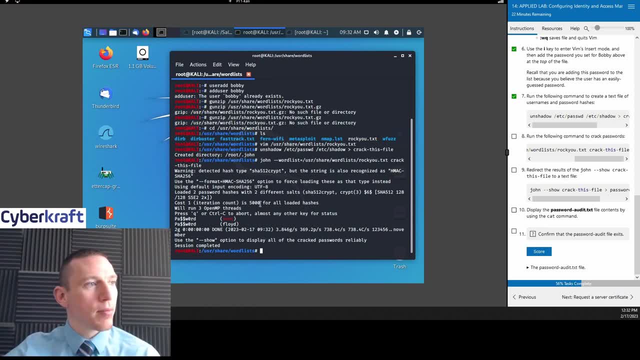 what hashes it's looking at. it thinks what hashes it's looking at. it thinks it's looking at a sha 256 hash. okay, it's looking at a sha 256 hash. okay, it's looking at a sha 256 hash. okay, loads two password hashes with two. 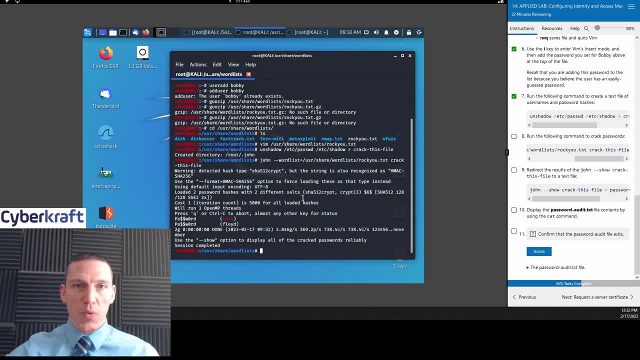 loads two password hashes with two loads, two password hashes with two different salts. remember salt is extra different salts. remember salt is extra different salts. remember salt is extra variable that you add to increase the variable that you add. to increase the variable that you add to increase the complexity of a hash. 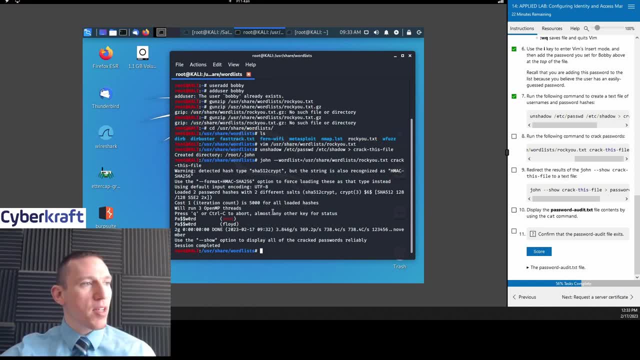 okay, and it's loading the uh the word okay, and it's loading the uh the word okay, and it's loading the uh the word. list that we have, list that we have, list that we have, and what it finds here is it finds a. and what it finds here is it finds a. 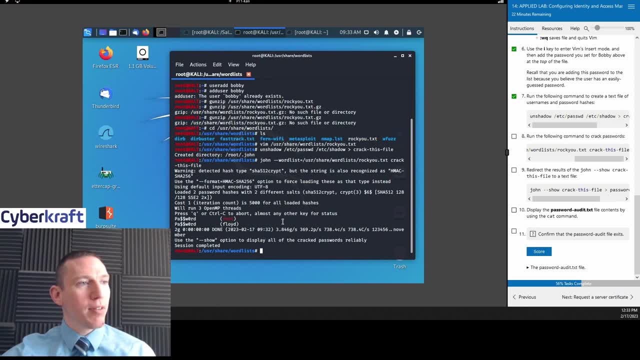 and what it finds here is: it finds a password for root and a password for password for root and a password for password for root and a password for floyd, floyd, floyd that we created earlier. remember we that we created earlier? remember we that we created earlier? remember we created that floyd account? 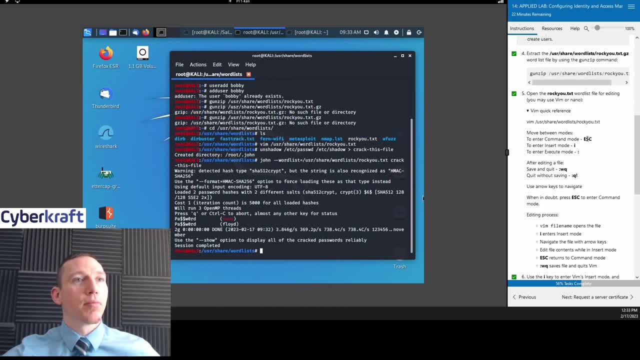 created that floyd account. created that floyd account. so i guess bobby was not created with. so i guess bobby was not created with. so i guess bobby was not created with that password, that password, that password. wow, i'm gonna have to retire. i staked my. 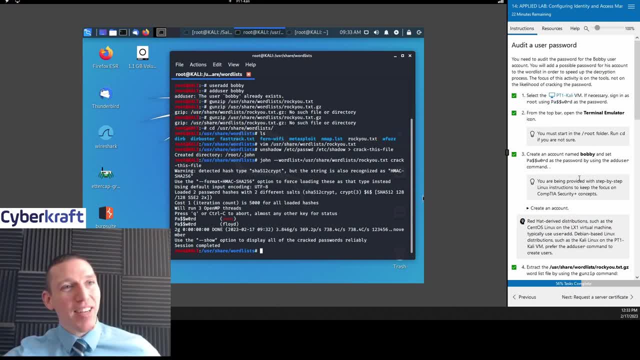 wow, i'm gonna have to retire. i staked my wow, i'm gonna have to retire. i staked my career on that career, on that career on that. but we did create another user earlier, but we did create another user earlier, but we did create another user earlier, which you know. i don't think this um. 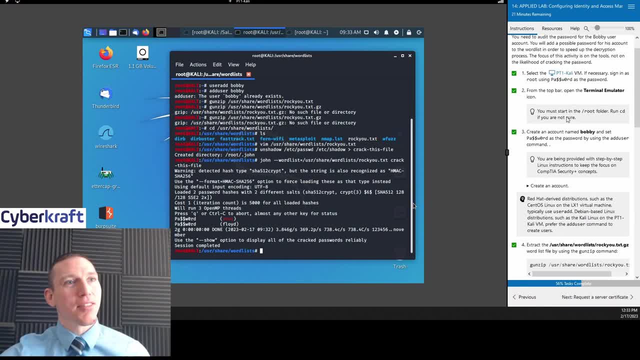 which you know, i don't think this um which you know, i don't think this um, these two labs were written by two. these two labs were written by two. these two labs were written by two different people. probably these two different people, probably these two different people, probably these two sections. 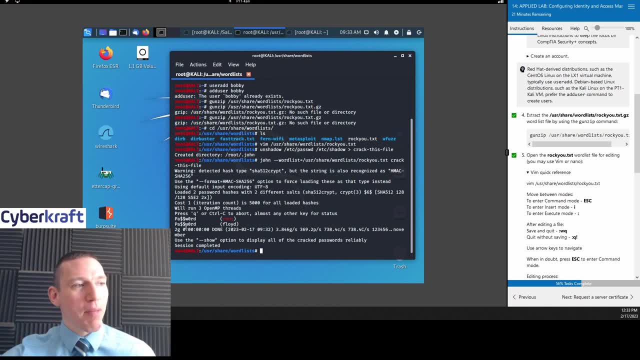 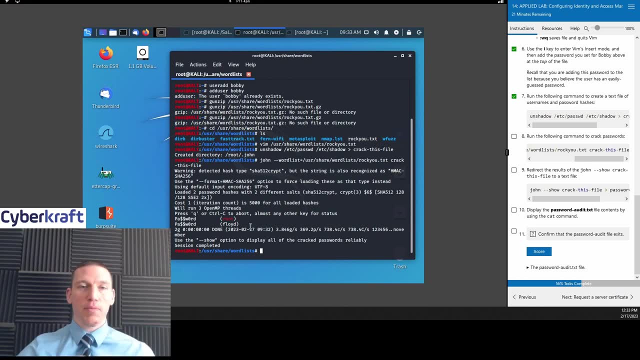 sections, sections, account. so since we've we included that account, so since we've we included that account, so since we've we included that password, password, password as a known plain plain text value, as a known plain plain text value, as a known plain plain text value. basically, what john the ripper is doing. 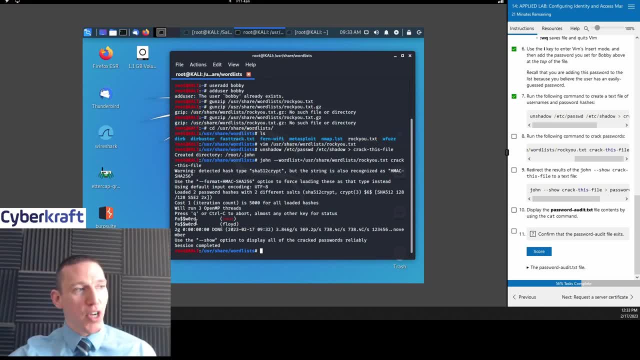 basically what john the ripper is doing. basically what john the ripper is doing. is it's taking a hash of that word? is it's taking a hash of that word? is it's taking a hash of that word? password- okay, shot 256 hash. password- okay, shot 256 hash. 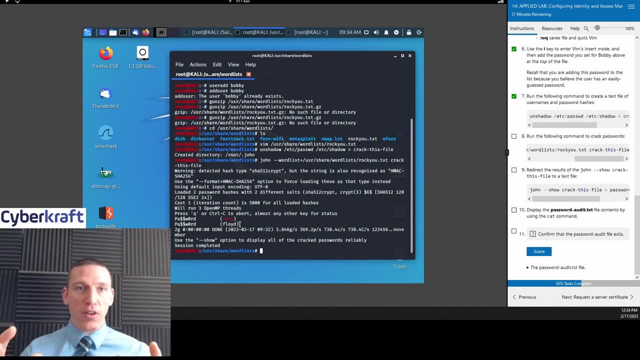 password: okay, shot 256, hash. and then it's examining the hashes. and then it's examining the hashes, and then it's examining the hashes that are found in the shadow folder. that are found in the shadow folder. that are found in the shadow folder. okay, in the cracklist file. 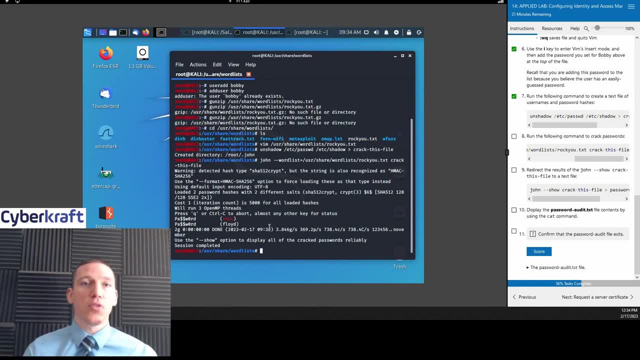 okay in the cracklist file. okay in the cracklist file and it's seeing if there's any matches and it's seeing if there's any matches. and it's seeing if there's any matches. and if there are, then it knows. and if there are, then it knows. 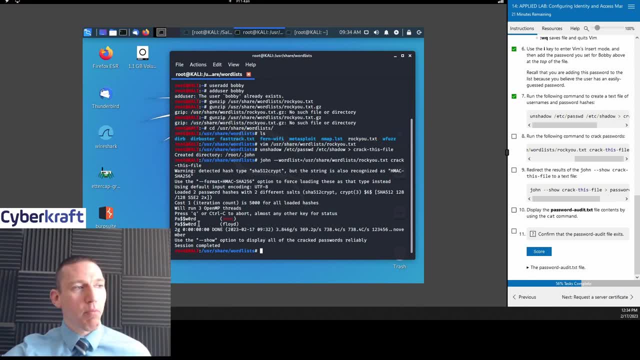 and if there are, then it knows that that hash represents that word, that hash represents that word, that hash represents that word. password- i hope that makes sense. password. i hope that makes sense. password. i hope that makes sense. we go over this a lot more in. i go over. 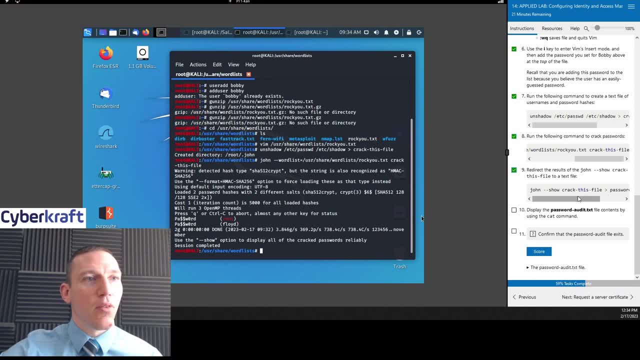 we go over this a lot more in. i go over. we go over this a lot more in. i go over this a lot more in my password, cracking this a lot more in my password, cracking this a lot more in my password, cracking video, video, video. but you know what we've done here, john. 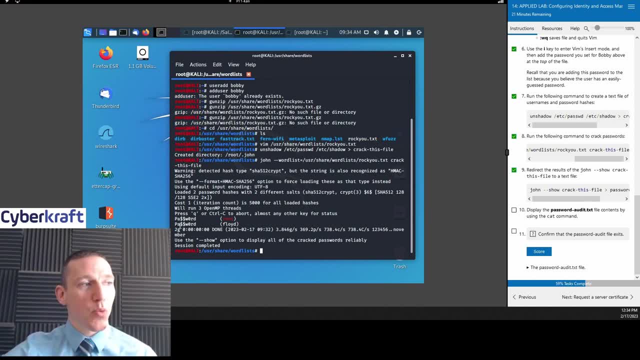 but you know what we've done here, john. but you know what we've done here, john. the ripper successfully identified. the ripper successfully identified. the ripper successfully identified that floyd's password is this password. that floyd's password is this password. that floyd's password is this password. so now we have. 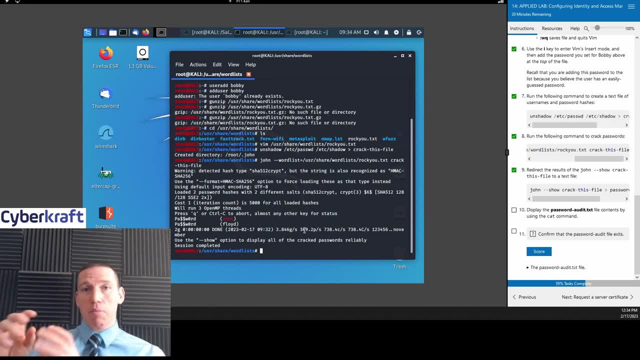 so now we have. so now we have the plain text value for floyd's password. the plain text value for floyd's password. the plain text value for floyd's password. okay, that password wasn't being okay. that password wasn't being okay, that password wasn't being stored. 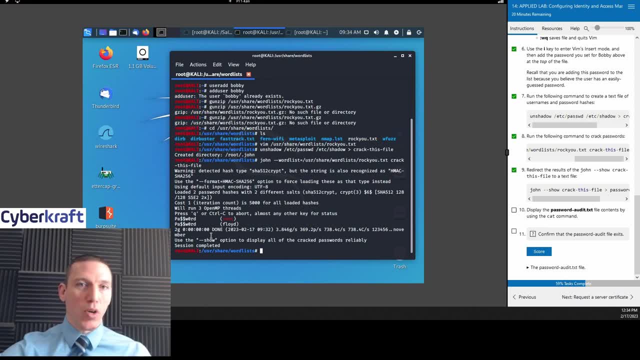 stored. stored in a text file. you know out of the blue in a text file. you know out of the blue in a text file. you know out of the blue. it was being stored as a password hash. it was being stored as a password hash. it was being stored as a password hash for added security. 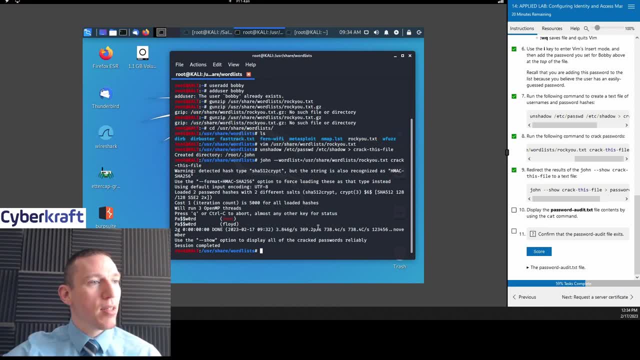 for added security. for added security, a shot 256 hash, to be precise. a shot 256 hash, to be precise. a shot 256 hash, to be precise. okay, so great. and then, uh, let's see, and then, uh, let's see, and then, uh, let's see file. 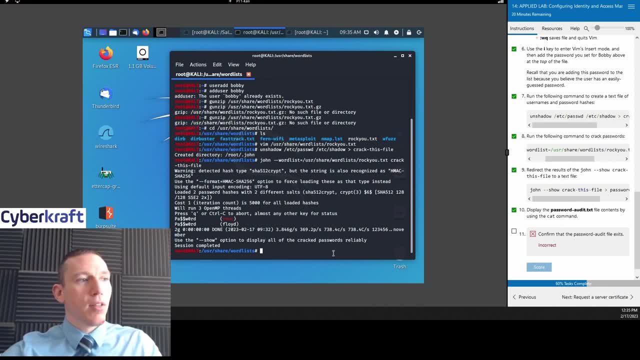 file file. uh, let's see. so we got to do john, so we got to do john, so we got to do john, double dash show, double dash show, double dash show, crack, crack, crack. this, this, this file, password, audittxt. now, what we're doing here is we're. 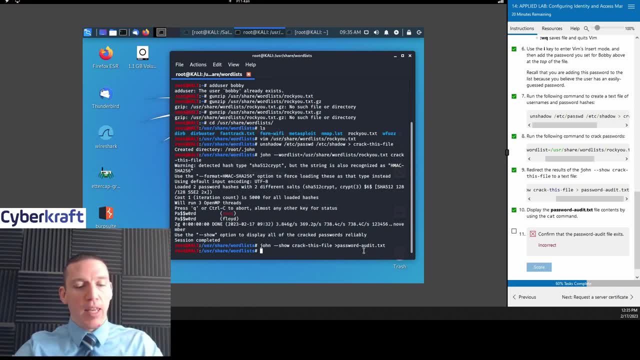 now, what we're doing here is: we're now what we're doing here is we're creating a file, creating a file, creating a file with our results, okay, and then we can with our results, okay, and then we can with our results, okay, and then we can show that file. 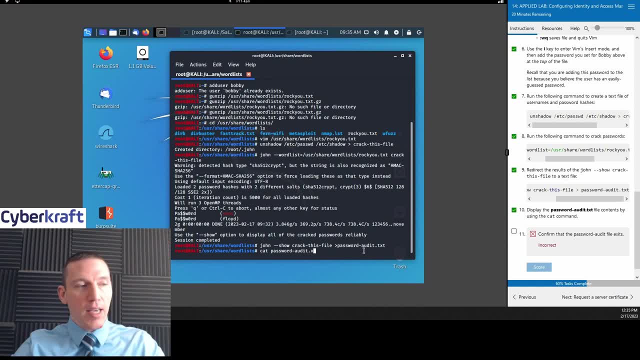 show that file. show that file: password: audit password. audit password. audit dot txt. dot txt, dot txt. i'm showing the results of that file by. i'm showing the results of that file by. i'm showing the results of that file by just using the cat command. and here we. 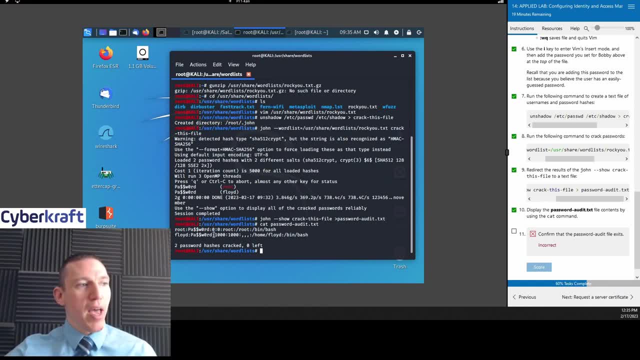 just using the cat command. and here we just using the cat command. and here we see root. the root password is password, see root. the root password is password: see root. the root password is password and floyd's password is password. okay, and floyd's password is password, okay. 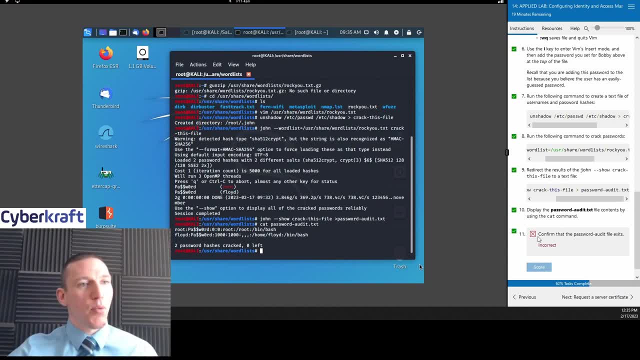 and floyd's password is password, okay. so now if we score this? oh, we can't. so now if we score this? oh we can't. so now if we score this? oh, we can't score that again. but we have it correct. score that again, but we have it correct. 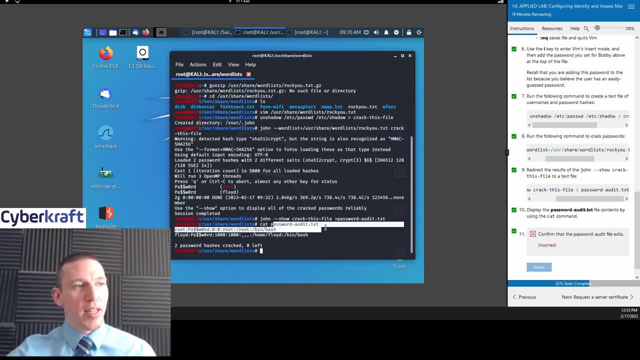 score that again, but we have it correct now because this is uh. this is the now because this is uh, this is the now because this is uh. this is the password audittxt that we had to create, password audittxt that we had to create, password audittxt that we had to create in this step nine. 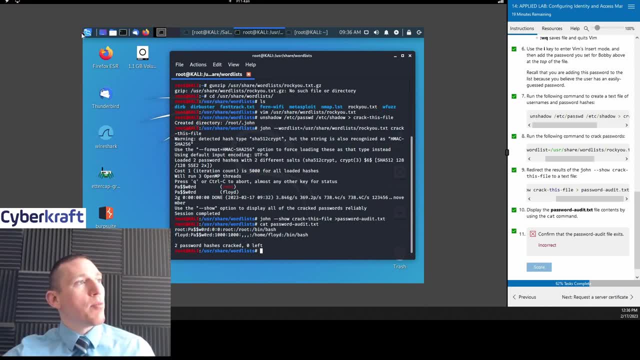 in this step. nine in this step. nine: all right, so great so we've used john. all right, so great, so we've used john. all right, so great so we've used john the ripper successfully, the ripper successfully, the ripper successfully. you can also access john the ripper. 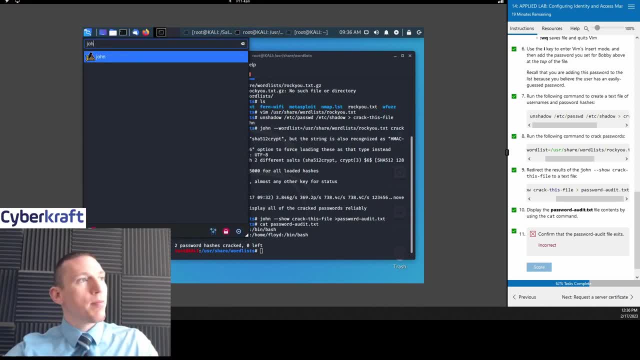 you can also access john the ripper. you can also access john the ripper through through, through you know, through here, you know through here, you know through here, through your, your main, through your, your main, through your, your main, drop down, and here you see a lot of. 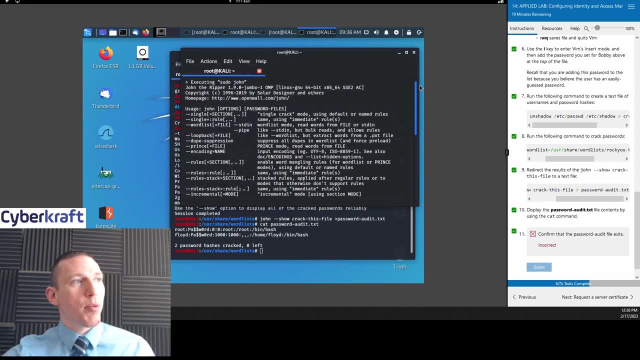 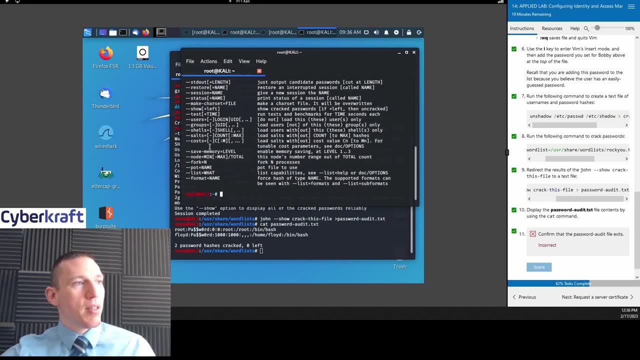 drop down, and here you see a lot of drop down, and here you see a lot of. this is how, if you want to learn more, this is how, if you want to learn more, this is how, if you want to learn more about john the ripper, you can. 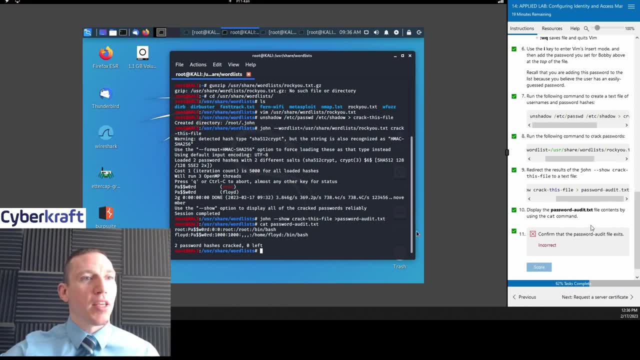 about john the ripper. you can about john the ripper. you can look through there pretty useful password. look through there pretty useful password. look through there pretty useful password. cracking utility- all right, so great cracking utility- all right, so great cracking utility- all right, so great, all right. so now we're going to go ahead. all right, so now we're going to go ahead. all right, so now we're going to go ahead and create a server certificate man and create a server certificate man and create a server certificate man. it's a long lab. this could probably be. it's a long lab, this could probably be. 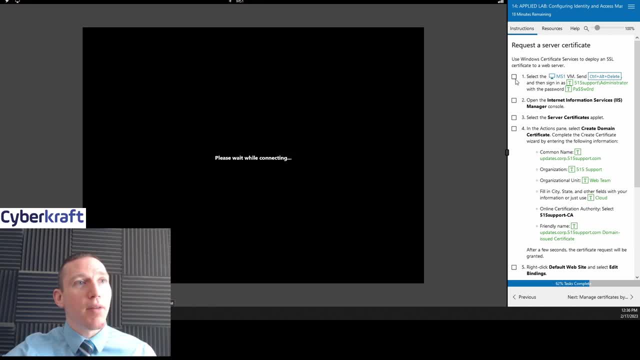 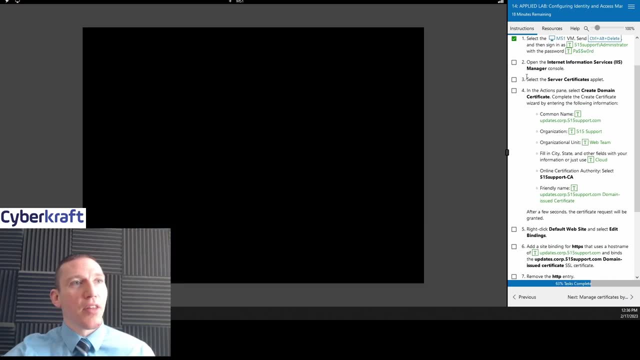 it's a long lab. this could probably be broken out into three labs. broken out into three labs. broken out into three labs. honestly, so we're going to go to ms1 honestly. so we're going to go to ms1 honestly. so we're going to go to ms1, and these aren't really linked together. 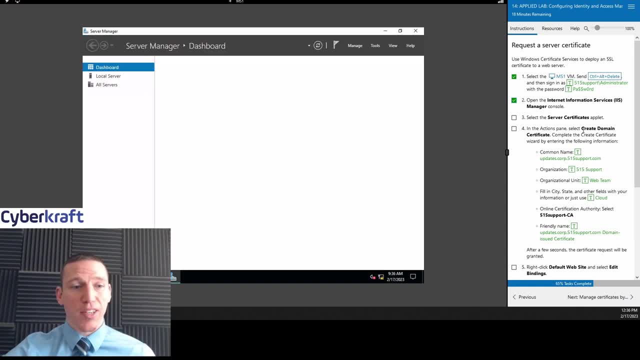 and these aren't really linked together and these aren't really linked together very well, all right. so now we're going very well, all right, so now we're going very well, all right, so now we're going to be opening to create certificates ssl, to be opening to create certificates ssl. 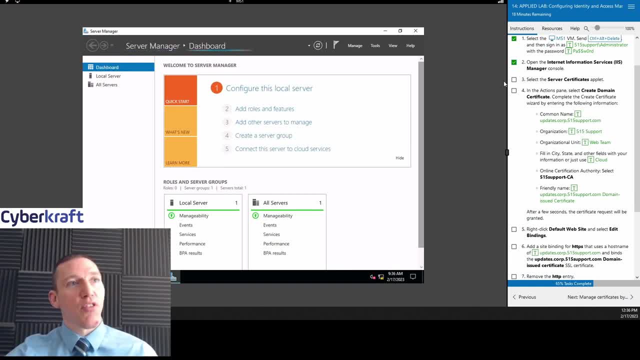 to be opening to create certificates, ssl certificates, tls certificates. we're certificates, tls certificates. we're certificates, tls certificates. we're going to be opening internet, going to be opening internet, going to be opening internet. information services: iis console information services. iis console information services. iis console: okay, 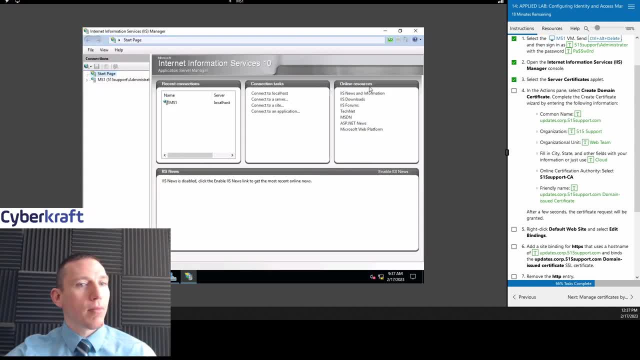 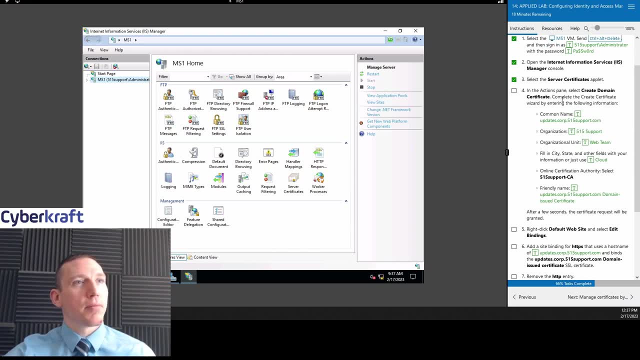 ias manager. okay, so from here we're going to go. okay, so from here we're going to go. okay, so from here we're going to go ahead and do 515 support administrator ahead and do 515 support administrator ahead and do 515 support administrator. server certificates. double click this. 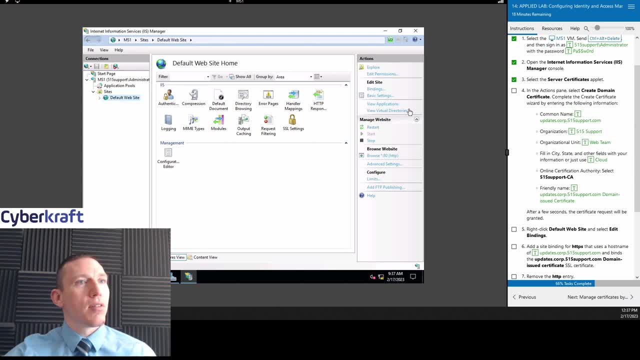 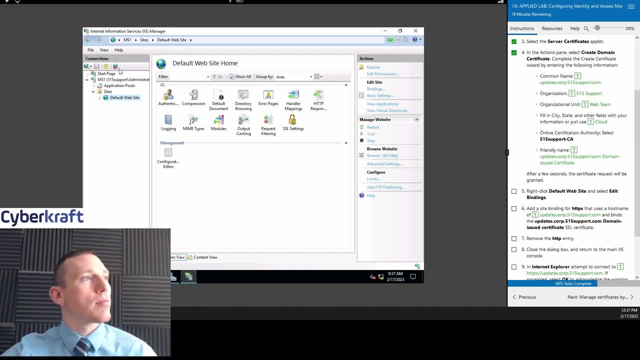 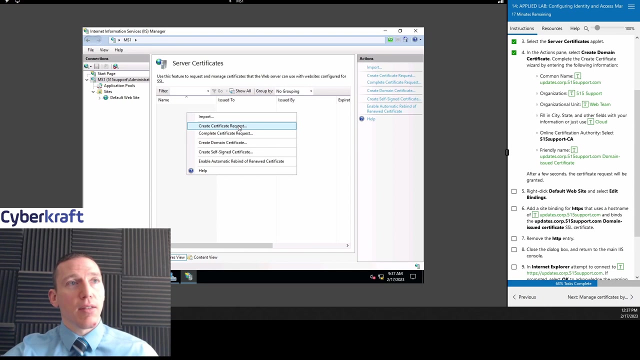 server certificates, double click this. server certificates, double click this. we go to sites. let's see what we're trying to do here. okay, from here. okay from here. okay from here. from server certificates, we can go ahead from server certificates, we can go ahead. from server certificates, we can go ahead and right-click: create domain certificate. 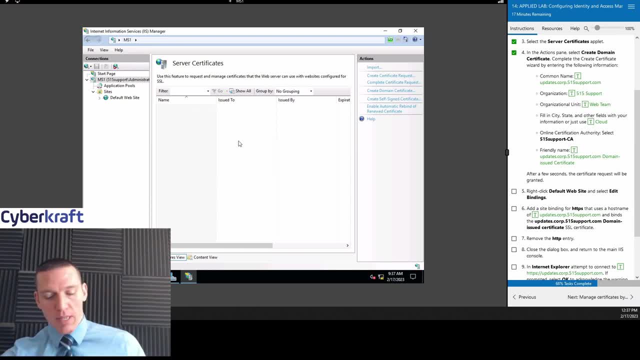 and right-click- create domain certificate. and right-click- create domain certificate, we go ahead create domain certificate. we go ahead create domain certificate. we go ahead create domain certificate. it's gonna take a moment, then it's gonna. it's gonna take a moment, then it's gonna. it's gonna take a moment, then it's gonna open up a wizard. 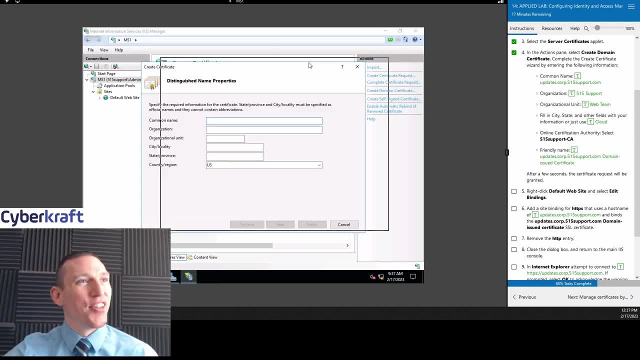 it is working. it's just taking a little. it is working. it's just taking a little. it is working, it's just taking a little longer. sometimes I wonder too if I did longer. sometimes I wonder too if I did longer. sometimes I wonder too if I did this. but it really just takes out that. 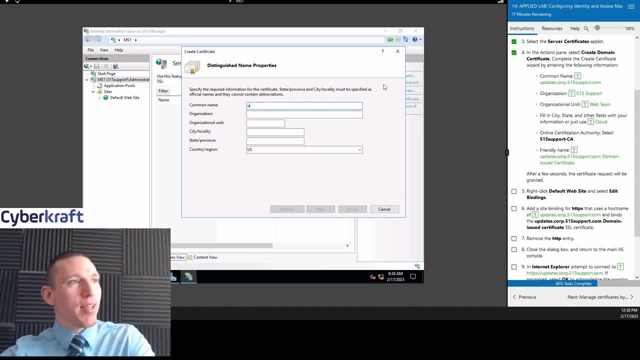 this, but it really just takes out that this, but it really just takes out that long all right, so we're gonna do long. all right, so we're gonna do long. all right, so we're gonna do updates. I'm just gonna go ahead and type updates. I'm just gonna go ahead and type. 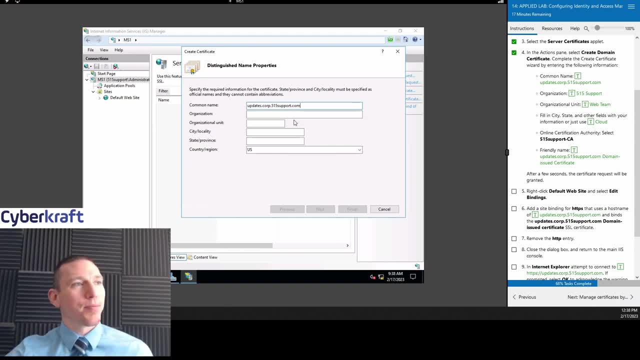 updates. I'm just gonna go ahead and type these in when you're not typing in these in, when you're not typing in these in, when you're not typing in command. so you're just typing in you command. so you're just typing in you command. so you're just typing in you know the organization name, the. 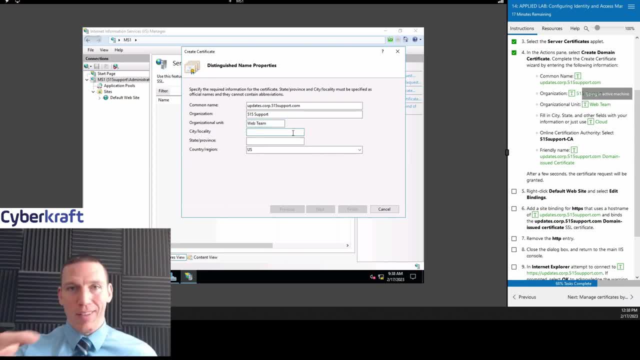 know the organization name. the know the organization name. the organizational unit. I don't think that organizational unit. I don't think that organizational unit. I don't think that really helps you learn any. the learn the really helps you learn any. the learn the really helps you learn any. the learn the lab any better. but when you have to, 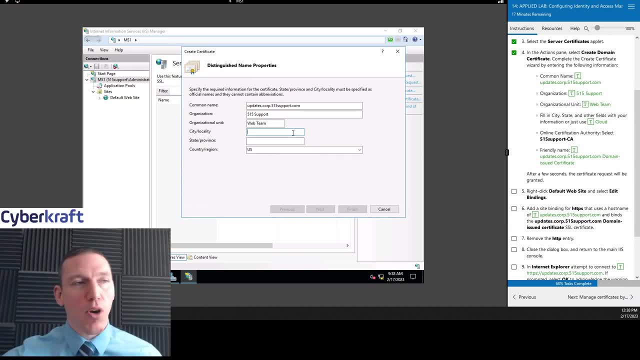 lab any better. but when you have to lab any better. but when you have to type in commands and PowerShell or terminal type in commands and PowerShell or terminal type in commands and PowerShell or terminal or command prompt, that's when I or command prompt, that's when I. 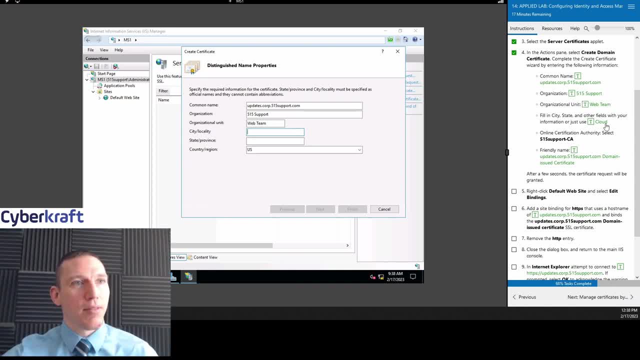 or command prompt. that's when I think it's important for you to type in type, think it's important for you to type in type, think it's important for you to type in type these in manually. but if you're these in manually, but if you're. 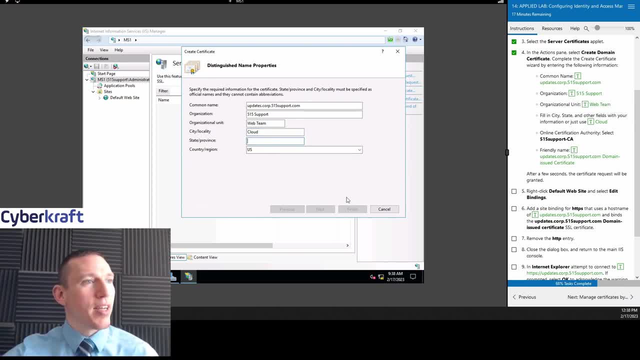 these in manually. but if you're doing this, just just use the helps, it's fine doing this, just just use the helps. it's fine doing this, just just use the helps, it's fine. okay, state province say it's in. okay, state province say it's in. 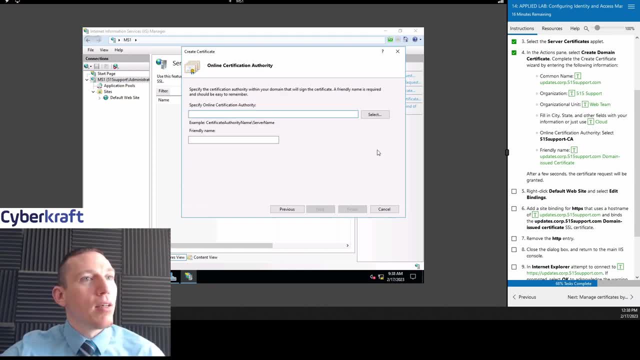 okay, state province say it's in Wyoming. okay, so we're gonna select our Wyoming. okay, so we're gonna select our Wyoming. okay. so we're gonna select our certificate authority. the car that's certificate authority, the car that's certificate authority, the car that's gonna be 515. support cost: the internal. gonna be 515 support cost. the internal gonna be 515 support cost the internal. car that we maintain. you know 515 car that we maintain. you know 515 car that we maintain. you know 515 support cop or type. this is a friendly support cop or type. this is a friendly. 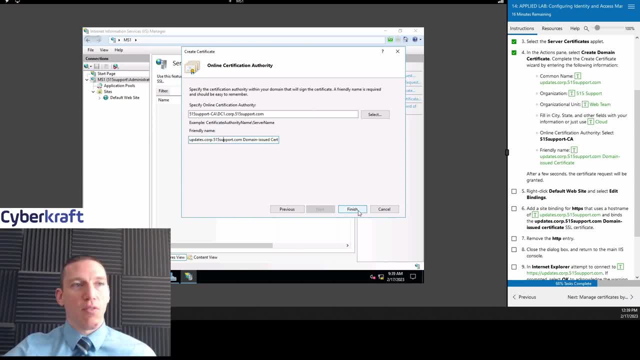 support, cop or type. this is a friendly name. the friendly name is gonna be a name. the friendly name is gonna be a name. the friendly name is gonna be a name that we can easily identify. okay, so, name that we can easily identify. okay, so, name that we can easily identify. okay, so what we've done here is we we're 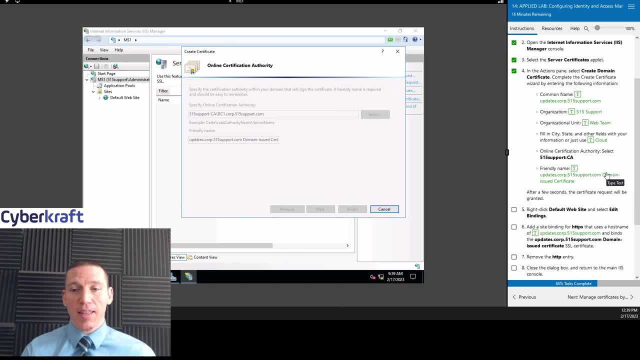 what we've done here is we. we're. what we've done here is we. we're creating a domain certificate. now we're creating a domain certificate. now we're creating a domain certificate. now we're paying the cop, we're asking them to you. paying the cop, we're asking them to you. 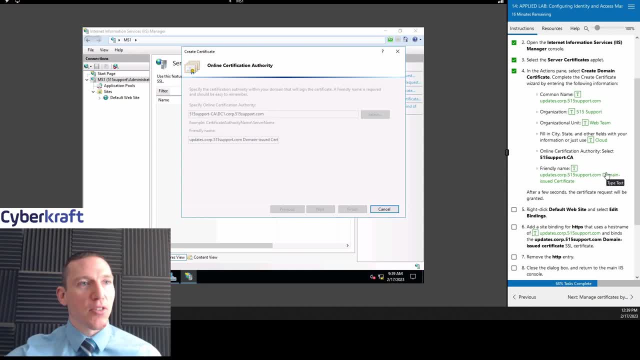 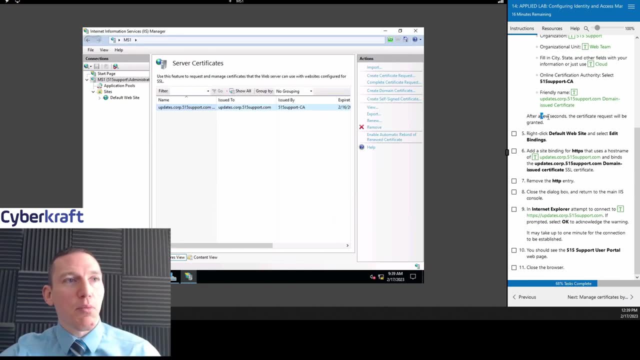 paying the cop. we're asking them to you. know we're asking the car to validate. know we're asking the car to validate. know we're asking the car to validate and create this domain certificate. says and create this domain certificate. says and create this domain certificate. says after a few seconds. might want to say a. 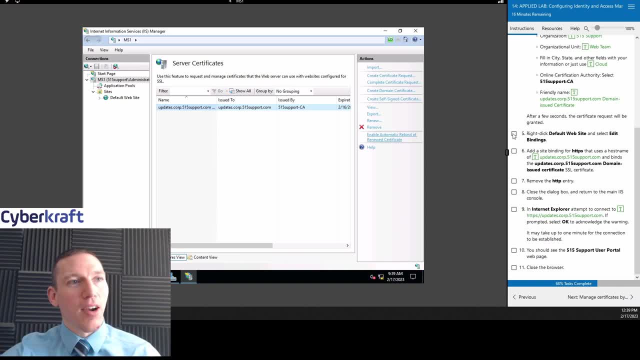 after a few seconds might want to say a after a few seconds, might want to say a few minutes: okay, it didn't take that few minutes. okay, it didn't take that few minutes. okay, it didn't take that long this time, all right, so go ahead. long this time, all right, so go ahead. 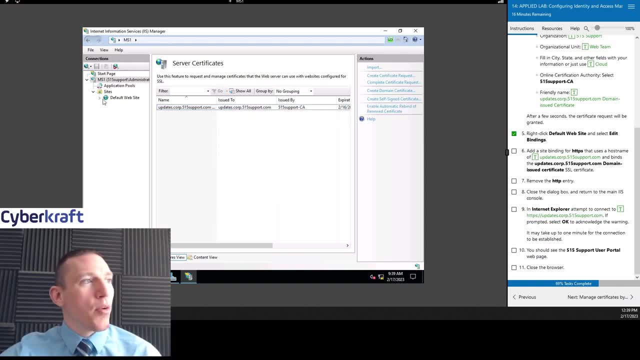 long this time. all right, so go ahead and right-click on this. I know we're and right-click on this. I know we're and right-click on this. I know we're right-click on default website. okay, so, right-click on default website. okay, so, right-click on default website. okay. so what we've done? we've created a. 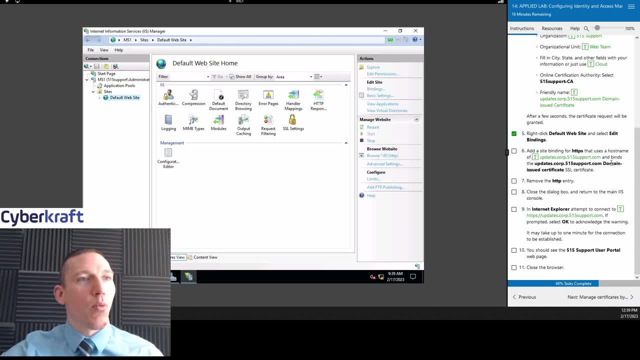 what we've done. we've created a. what we've done, we've created a certificate. now we'll be adding that certificate now. we'll be adding that certificate. now we'll be adding that certificate to our website here. all certificate to our website here. all certificate to our website here. all right, we're gonna go ahead and 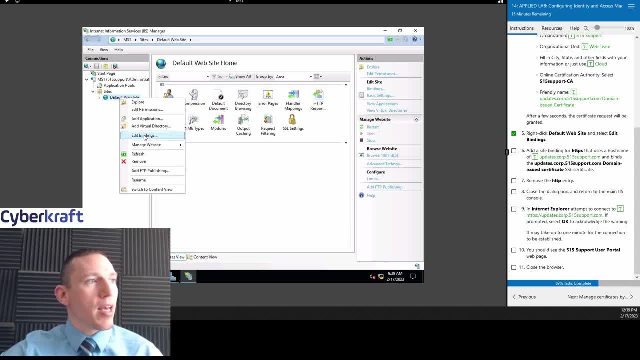 right, we're gonna go ahead and right, we're gonna go ahead and right-click this edit bindings- okay. or you right-click this edit bindings, okay. or you right-click this edit bindings- okay, or you can go. you click on it, go to the can go. you click on it, go to the. 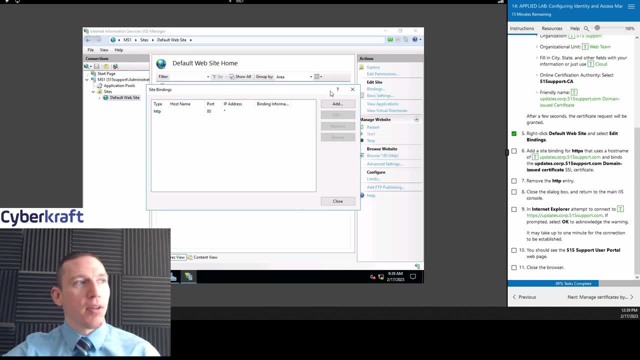 can go. you click on it. go to the right actions- edit bindings. okay, now we have right actions- edit bindings. okay, now we have right actions- edit bindings. okay, now we have HTTP port 80. I believe we're gonna HTTP port 80. I believe we're gonna. 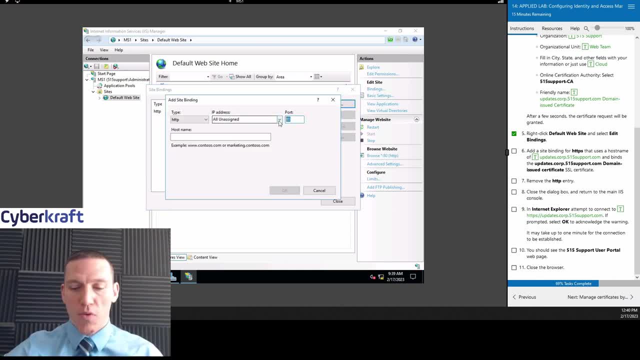 HTTP port 80. I believe we're gonna be removing that. we're gonna go ahead and be removing that. we're gonna go ahead and be removing that. we're gonna go ahead and add one for 443. try not to look on. add one for 443. try not to look on. 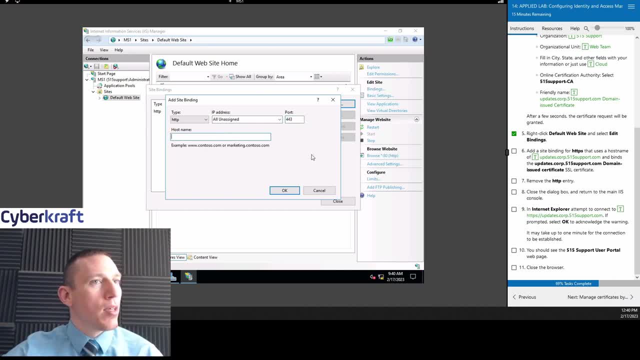 add one for 443. try not to look on the right side. we're gonna have to have the the right side. we're gonna have to have the the right side. we're gonna have to have the host name. here we type this in: host name. here we type this in. 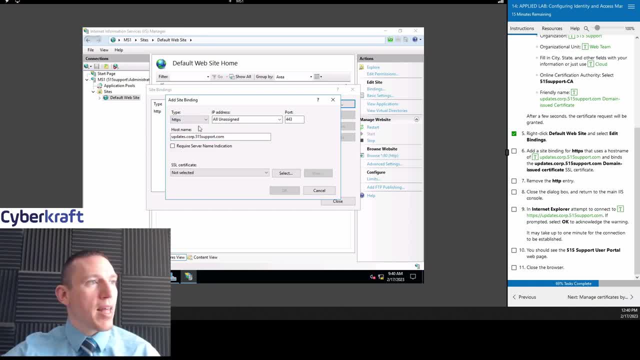 host name. here we type this in updates: a quarter 515 support- comm. make updates a quarter 515 support comm. make updates a quarter 515 support comm. make that HTTPS. we're gonna select their that HTTPS. we're gonna select their that HTTPS. we're gonna select their certificate. so we're forcing a secure. 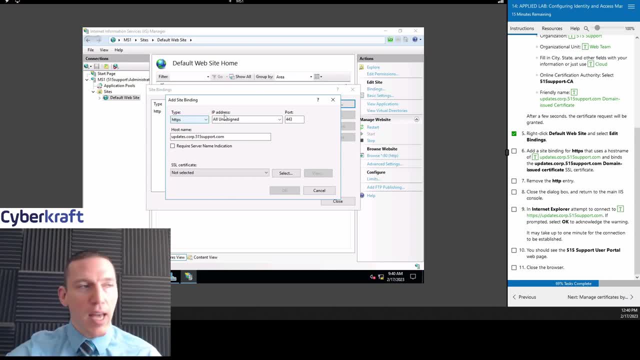 certificate. so we're forcing a secure certificate. so we're forcing a secure connection using HTTPS now to do that connection using HTTPS now to do that connection using HTTPS now to do that. it's gonna operate a report 443, remember. it's gonna operate a report 443, remember. 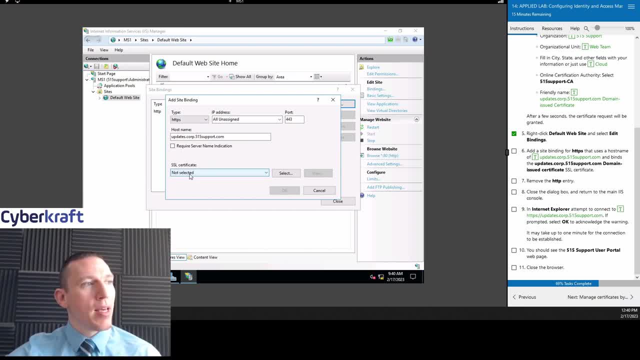 it's gonna operate a report 443. remember, HTTPS operates over 4443 and we have to. HTTPS operates over 4443 and we have to. HTTPS operates over 4443 and we have to select a certificate. you need a SSL or select a certificate. you need a SSL, or. 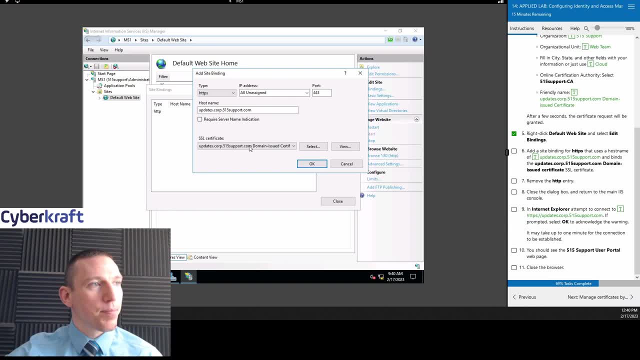 select a certificate. you need a SSL or TLS certificate. remember we're really TLS certificate. remember we're really TLS certificate. remember we're really using TLS here to do this. okay, now it using TLS here to do this. okay, now it using TLS here to do this. okay, now it says SSL, but it's just because this is. 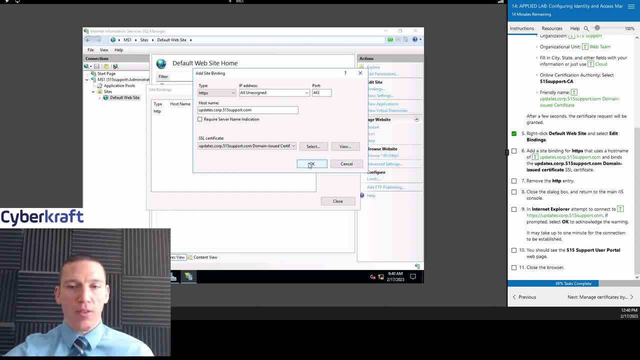 says SSL, but it's just because this is says SSL, but it's just because this is an older version of server manager, right? an older version of server manager, right, an older version of server manager. right now, SSL is deprecated. we're using TLS. now, SSL is deprecated, we're using TLS. 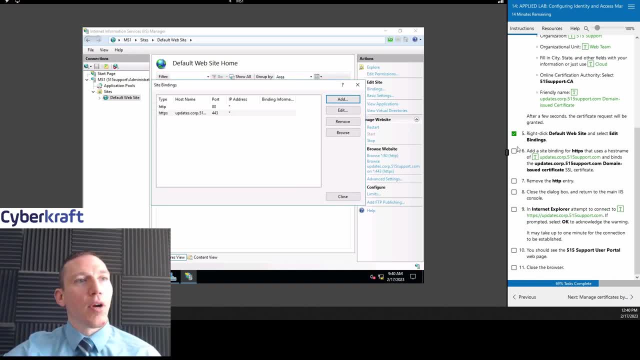 now SSL is deprecated. we're using TLS, so we're create that and that should. so we're create that and that should. so we're create that and that should. work site binding. let's see if we did work site binding. let's see if we did work site binding. let's see if we did that correct. yep, and we'll remove the. 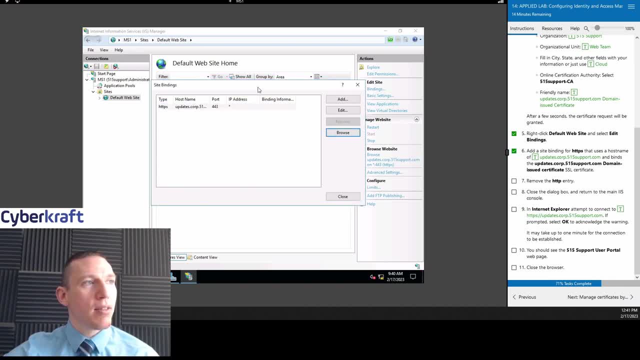 that correct, yep, and we'll remove the. that correct, yep, and we'll remove the HTTP binding- okay, and then we're going HTTP binding- okay, and then we're going HTTP binding- okay, and then we're going to close this and we should be in set. 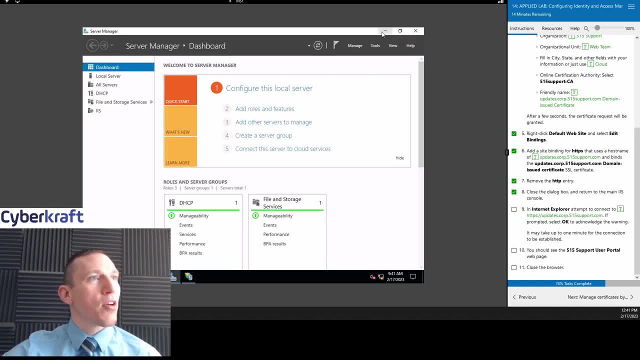 to close this and we should be in set to close this and we should be in set now. let's go ahead and open up Internet now. let's go ahead and open up Internet now. let's go ahead and open up Internet Explorer- still using Internet Explorer. Explorer- still using Internet Explorer. 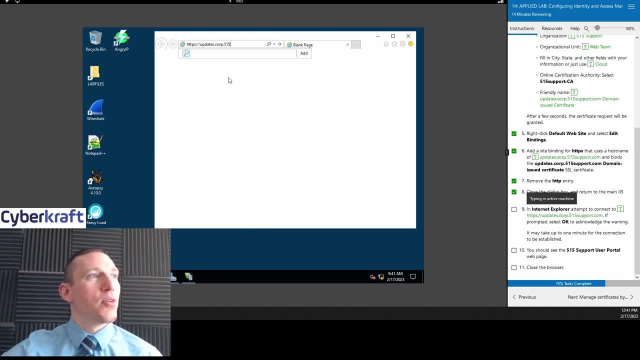 Explorer still using Internet Explorer in this lab and we're gonna navigate to in this lab and we're gonna navigate to in this lab and we're gonna navigate to the updates website. it's gonna give us a the updates website. it's gonna give us a the updates website. it's gonna give us a warning about secure connection. that's. 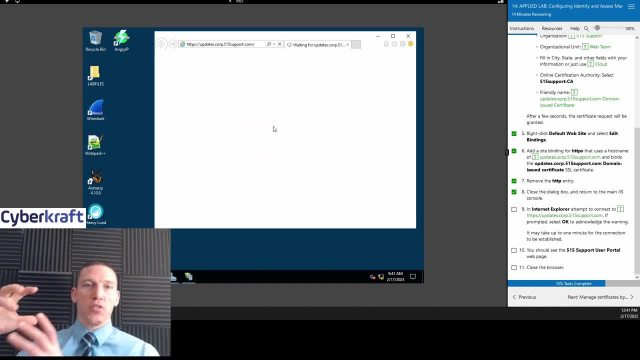 warning about secure connection. that's warning about secure connection. that's because this is a self-signed, because this is a self-signed, because this is a self-signed certificate and we're signing this use certificate and we're signing this use certificate and we're signing this use, our internal certificate Authority. so 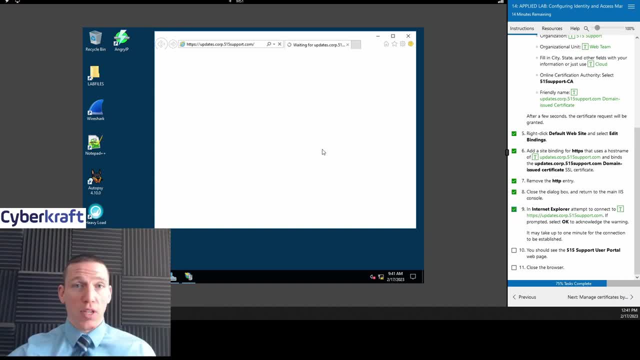 our internal certificate Authority. so our internal certificate Authority. so it's not the certificates not located in. it's not the certificates not located in. it's not the certificates not located in this browsers root certificate store. this browsers root certificate store. this browsers root certificate store, which is what the browser uses to. 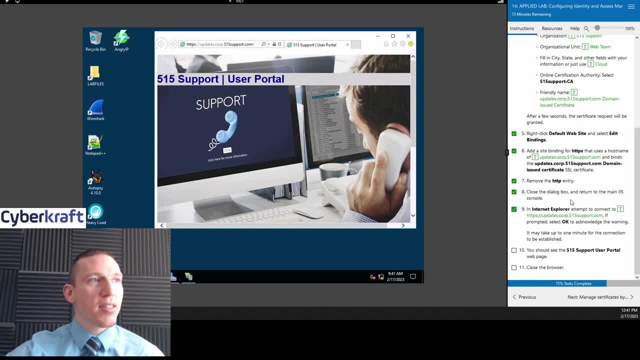 which is what the browser uses to. which is what the browser uses to recognize a secure certificate, and it recognize a secure certificate and it recognize a secure certificate and it does successfully navigate to the does successfully navigate to the does successfully navigate to the website and we can see with this lock. 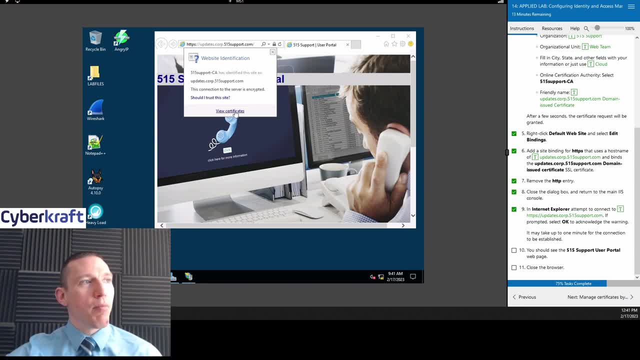 website and we can see with this lock website and we can see with this lock icon that we are connecting through an icon, that we are connecting through an icon, that we are connecting through an HTTPS connection. now we can view that HTTPS connection. now we can view that. 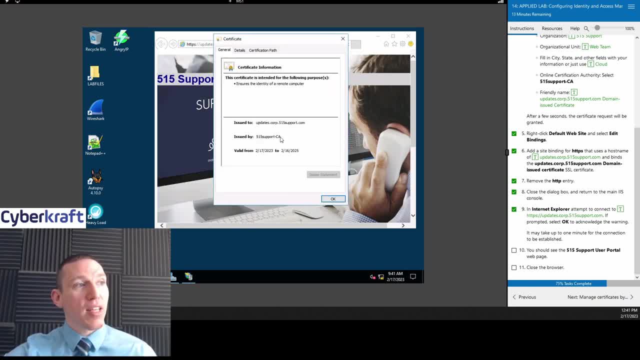 HTTPS connection. now we can view that certificate here and we can see that certificate here and we can see that certificate here and we can see that the certificate is issued by 515 support. the certificate is issued by 515 support. the certificate is issued by 515 support. car, okay, and it's valid from today. 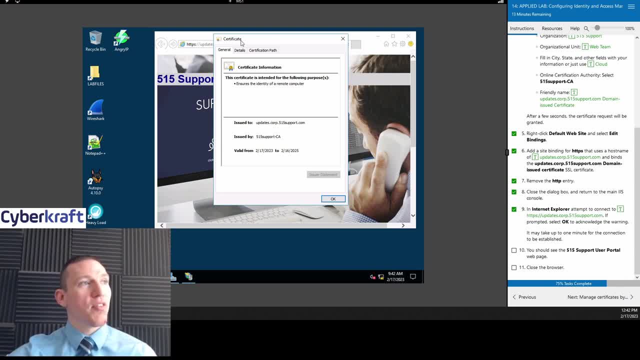 car okay, and it's valid from today. car okay, and it's valid from today because we created it today until 2025, because we created it today until 2025, because we created it today until 2025. so this is a certificate we just made. 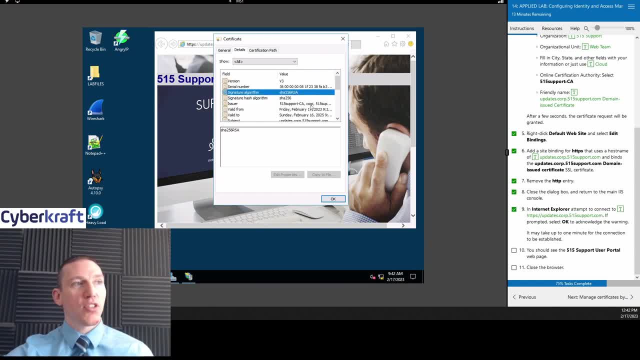 so this is a certificate we just made. so this is a certificate we just made. it's a shot 256 certificate uses shot 256. it's a shot 256 certificate uses shot 256. it's a shot 256 certificate uses shot 256. RSA or Revis Shamir Ottoman encryption. 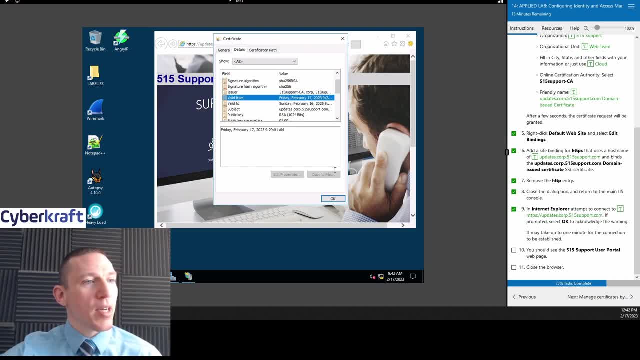 RSA or Revis Shamir Ottoman encryption. RSA or Revis Shamir Ottoman encryption, and it was created at 929 am or it was. and it was created at 929 am or it was and it was created at 929 am or it was valid. I say it's interesting, is valid. 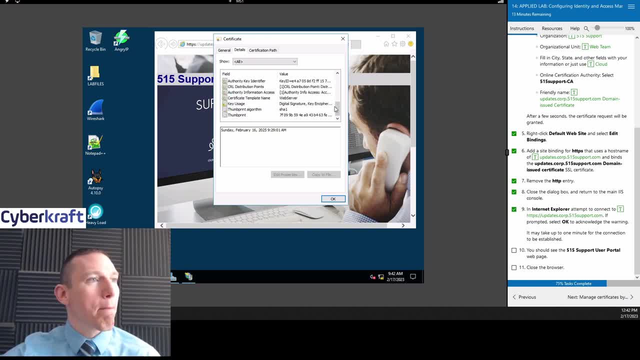 valid, I say it's interesting is valid. valid, I say it's interesting, is valid ten minutes before when we created it, ten minutes before when we created it, ten minutes before when we created it, which is pretty interesting, so all sorts. which is pretty interesting, so all sorts. 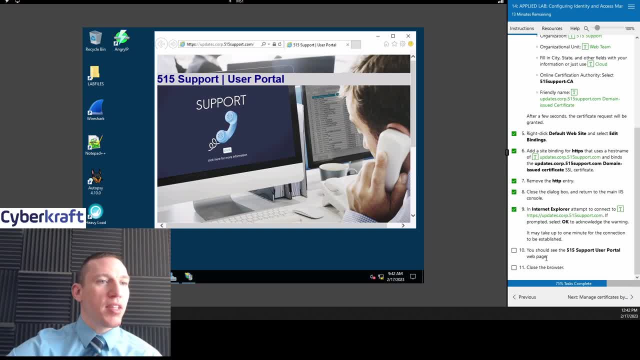 which is pretty interesting. so all sorts of information you can see about the of information you can see about the of information you can see about the certificate. none of this is really I'll certificate. none of this is really I'll certificate. none of this is really. I'll tell you to do this here. it just says: 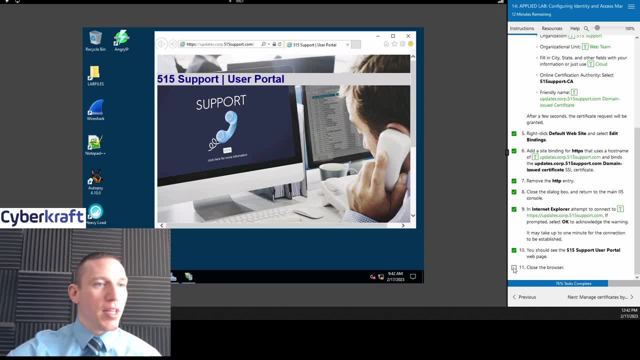 tell you to do this here. it just says: tell you to do this here. it just says: you know if you've loaded the website. you know if you've loaded the website. you know if you've loaded the website. you've done it correctly, which we did. you've done it correctly, which we did. 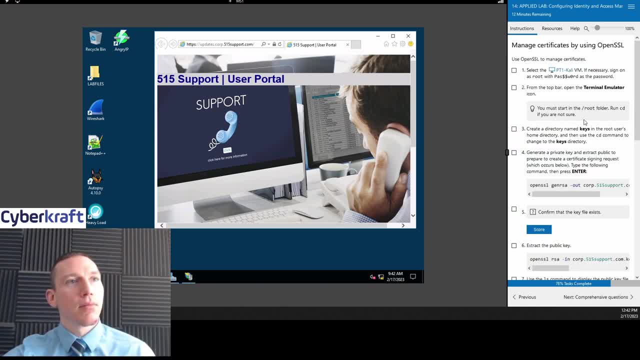 you've done it correctly, which we did, okay, okay, so now we're going back to okay. okay, so now we're going back to okay. okay, so now we're going back to Cali. I'm surprised this is still going Cali. I'm surprised this is still going. 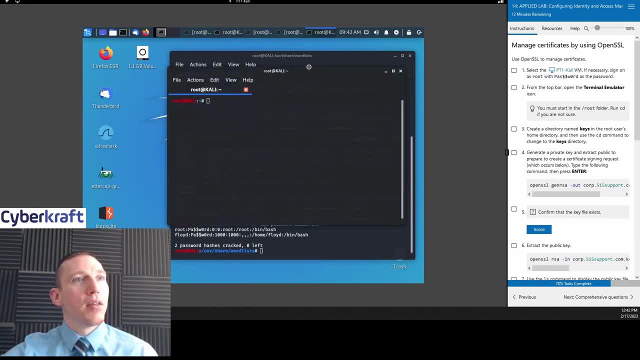 Cali. I'm surprised this is still going. this is a one of the longest labs in the. this is a one of the longest labs in the. this is a one of the longest labs in the whole thing. okay, so now we're gonna go. whole thing. okay, so now we're gonna go. 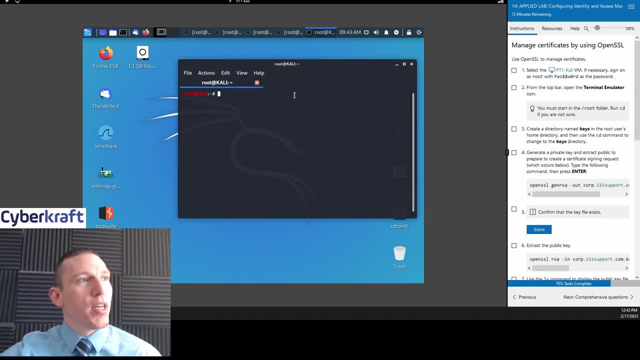 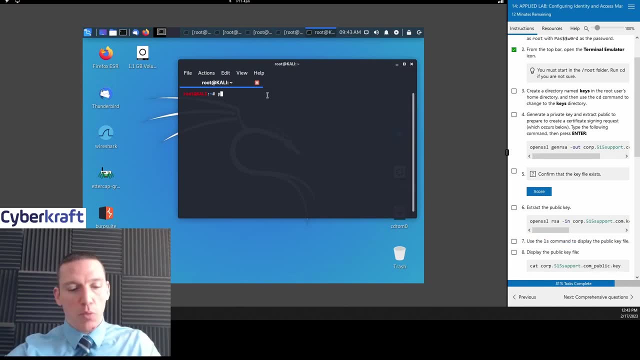 whole thing. okay. so now we're gonna go back to Cali. let me minimize our old back to Cali. let me minimize our old back to Cali. let me minimize our old terminal window opening a new terminal terminal window opening a new terminal terminal window opening a new terminal. make sure we're in the root folder, yep. make sure we're in the root folder: yep, make sure we're in the root folder. yep, we're in the root. if you open up a new, we're in the root. if you open up a new, we're in the root. if you open up a new terminal, you're gonna be in the root. 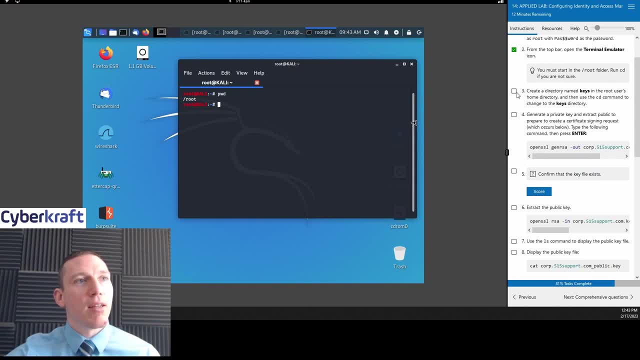 terminal. you're gonna be in the root terminal. you're gonna be in the root folder, so don't have to keep checking it folder. so don't have to keep checking it folder. so don't have to keep checking it. but it's good practice to practice these. 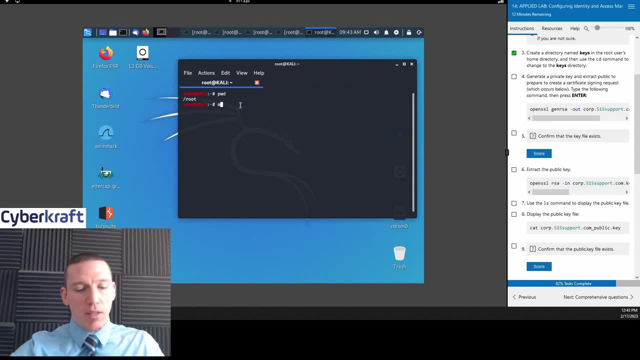 but it's good practice to practice these. but it's good practice to practice these commands. now we're to create a directory commands. now we're to create a directory commands. now we're to create a directory- make directory- and then we're gonna call make directory, and then we're gonna call. 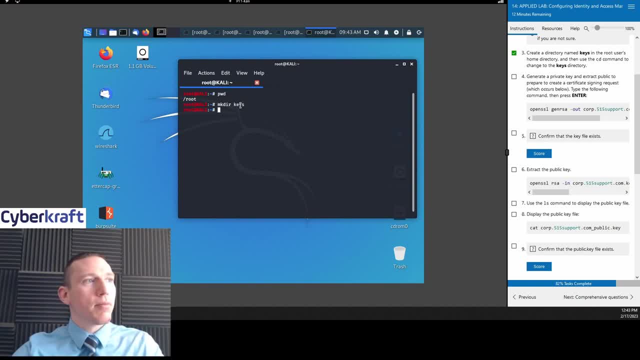 make directory and then we're gonna call that keys okay. and then you know, see that keys okay. and then you know, see that keys okay. and then you know, see, we've made that directory keys we can. we've made that directory keys we can. we've made that directory keys we can see it here in the root directory we have. 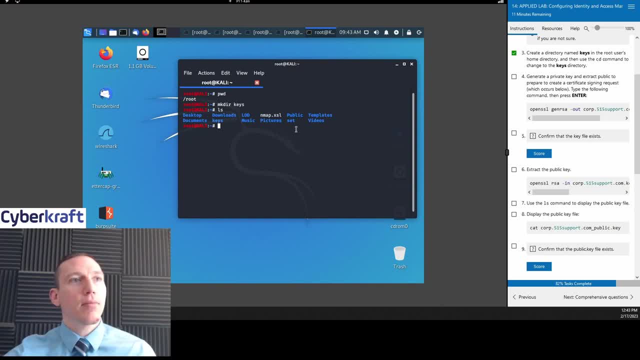 see it here in the root directory. we have. see it here in the root directory. we have a directory called keys. then we can do a directory called keys. then we can do a directory called keys. then we can do change directory to keys. you don't need change directory to keys, you don't need. 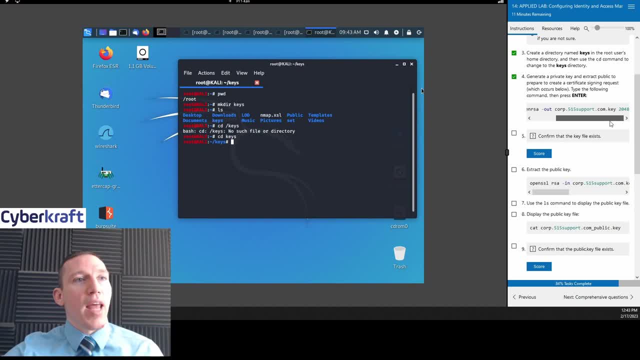 change directory to keys. you don't need the slash CD keys. okay, now we're gonna the slash CD keys. okay, now we're gonna the slash CD keys. okay, now we're gonna be using terminal commands. oh so we're be using terminal commands. oh so we're. 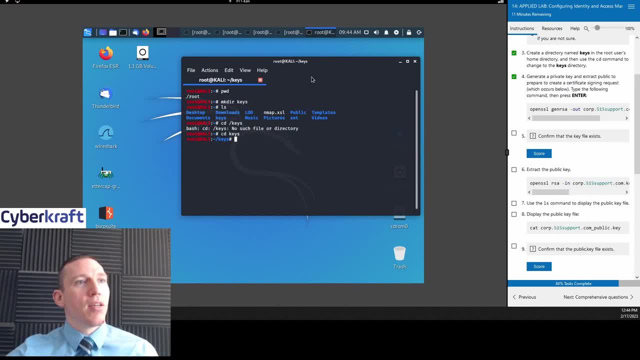 be using terminal commands. oh so we're doing the same thing, but we're doing in doing the same thing, but we're doing in doing the same thing, but we're doing in Linux. okay, great, so this makes sense. doing the same thing, but we're doing in Linux. okay, great, so this makes sense. 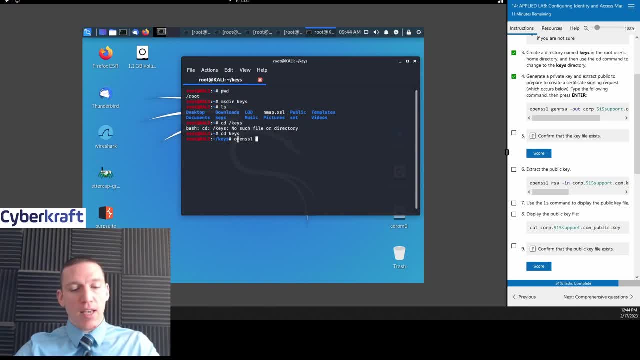 doing the same thing, but we're doing in Linux. okay, great, so this makes sense. cell command: open SSL command: open SSL gen RSA output. cell command: open SSL command. open SSL gen RSA output. cell command: open SSL command: open SSL gen RSA output. member RSA rivets: Samir Adelman. 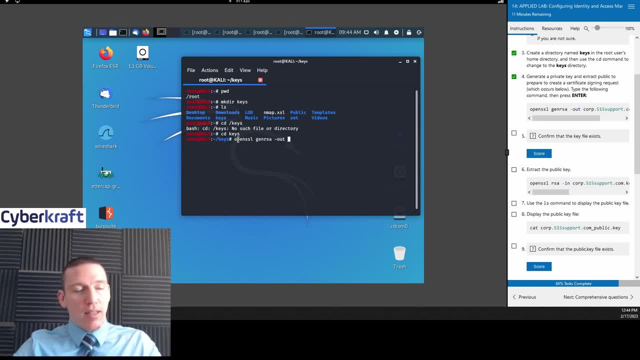 member. RSA rivets Samir Adelman. member- RSA rivets Samir Adelman. should be generating SSL certificate using. should be generating SSL certificate using. should be generating SSL certificate using that, that certificate for that, that, that certificate for that, that that certificate for that encryption algorithm. okay, we're gonna. 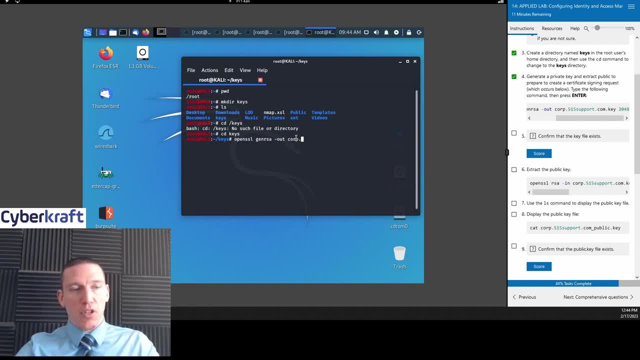 encryption algorithm. okay, we're gonna encryption algorithm. okay, we're gonna specify the output. what are we naming? specify the output. what are we naming? specify the output. what are we naming these certificates? we corped a 515. these certificates. we corped a 515. these certificates. we corped a 515 calm key and then we're gonna be key and. 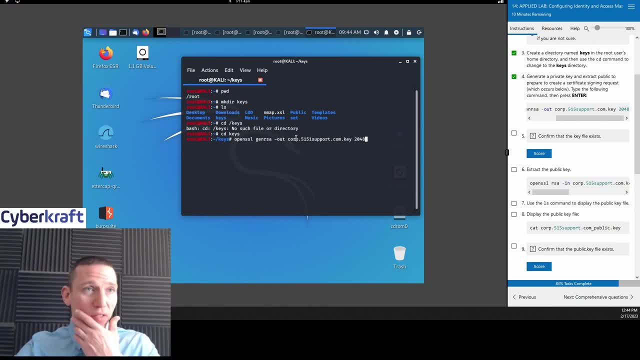 calm key, and then we're gonna be key and calm key, and then we're gonna be key, and then we're gonna be specifying the. then we're gonna be specifying the. then we're gonna be specifying the length of certificate as 2048 generates. length of certificate as 2048 generates. 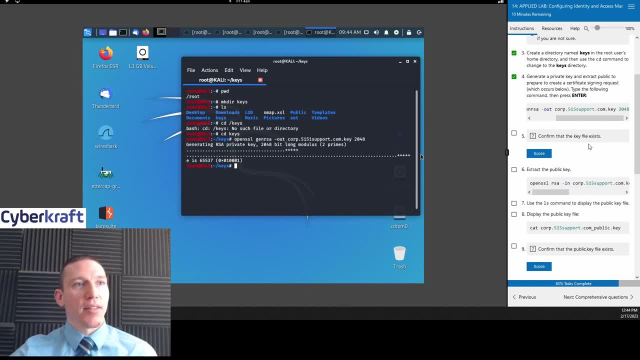 length of certificate, as 2048 generates an RSA private key. and it did that- an RSA private key. and it did that- an RSA private key. and it did that successfully. we can confirm that with the successfully. we can confirm that with the successfully. we can confirm that with the script, now we can subtract that extract. 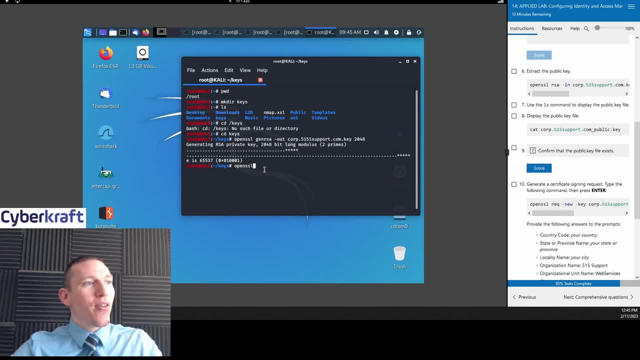 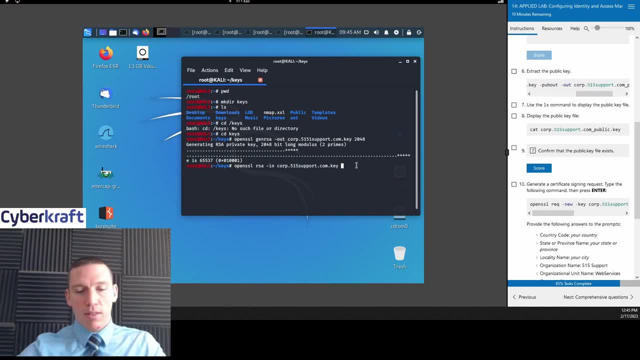 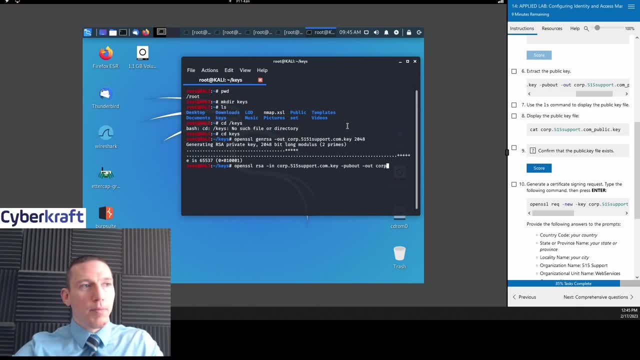 now we're gonna go ahead and select the output, and then we're now we're gonna go ahead and select the output, and then we're gonna go ahead and do that, gonna go ahead, and do that, gonna go ahead and do that. dash out corp 515: support calm. 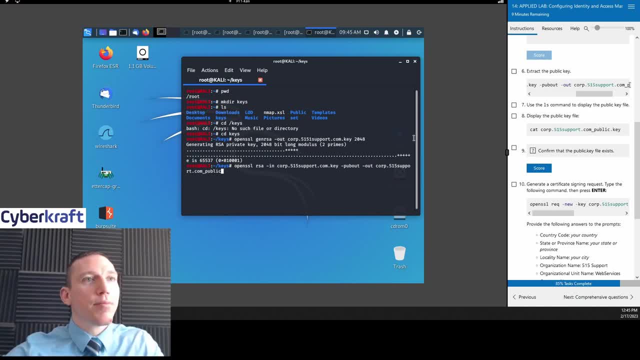 dash out corp 515- support- calm. dash out corp 515- support calm. underscore public key. so we've created a underscore public key. so we've created a underscore public key. so we've created a private key and now we're creating a private key, and now we're creating a. 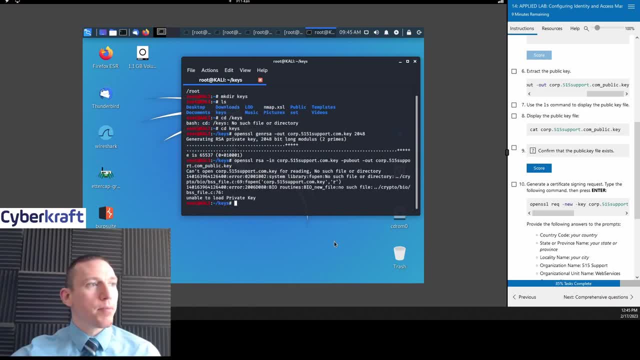 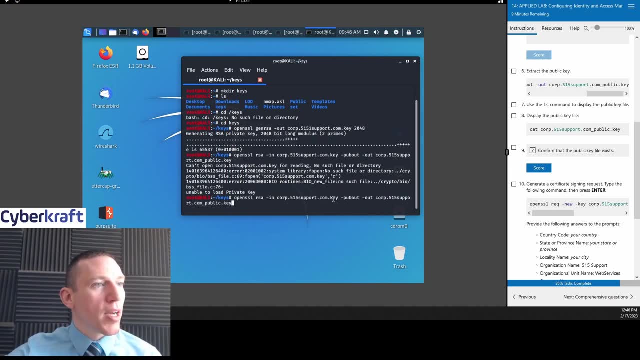 private key and now we're creating a public key. so we have a private and public key. so we have a private and public key. so we have a private and public key pair. I mistyped something. public key pair. I mistyped something- public key pair. I mistyped something. let's see: corp to 515: support calm key. 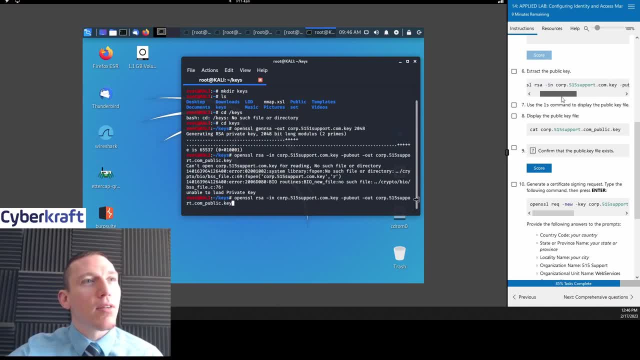 let's see: corp to 515- support calm key. let's see: corp to 515- support calm key. corp to 515- support calm public key. I never load private key, so it should be. I never load private key, so it should be. I never load private key, so it should be something here that I messed up open SSL. 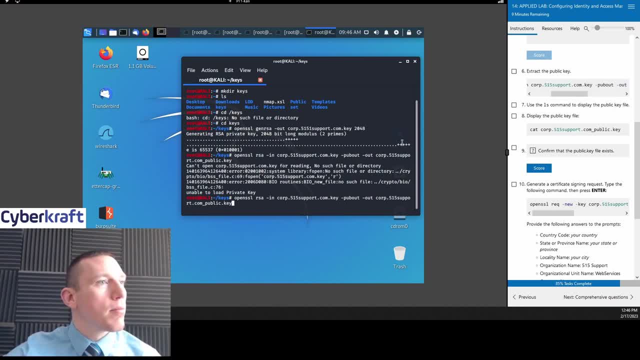 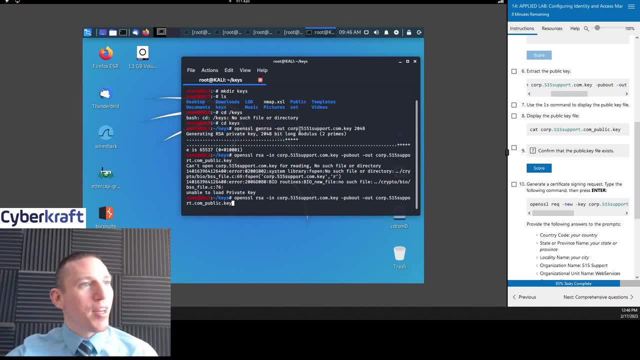 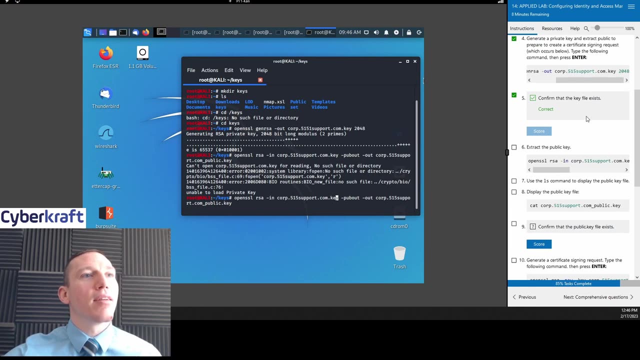 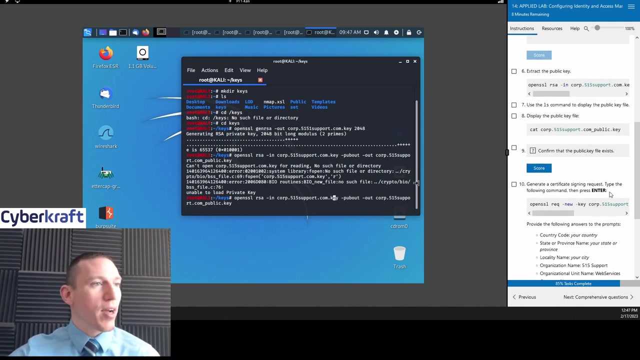 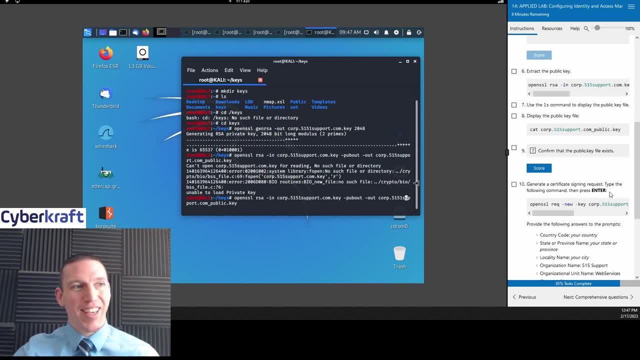 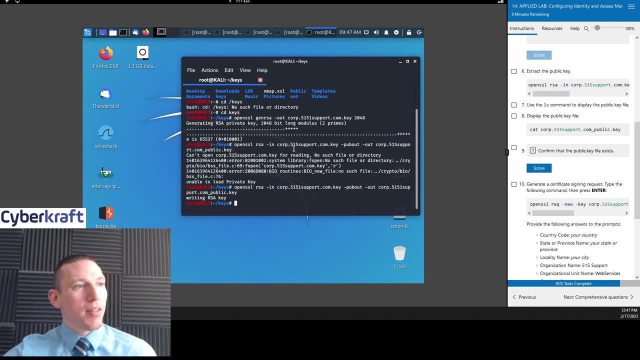 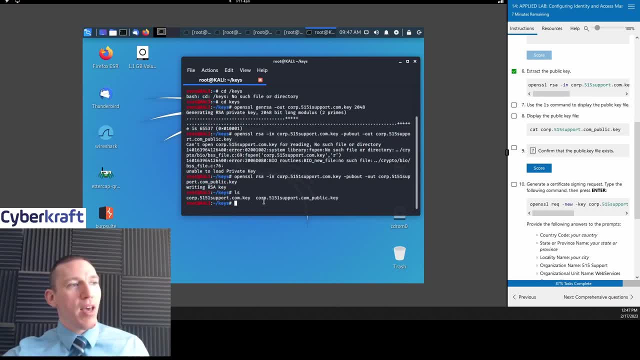 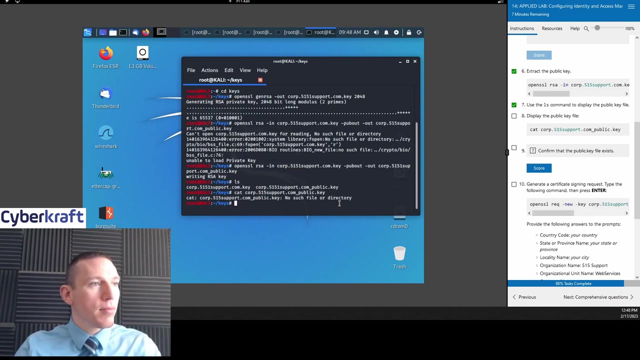 the keys folder and we can see that we have a private key and a public key. looks great and we can. then we can display the public key core up to five. one: five support calm underscore. public key: no again, this is 51 51 support. this is the next evolution of 515 support. if you thought 515 support was. 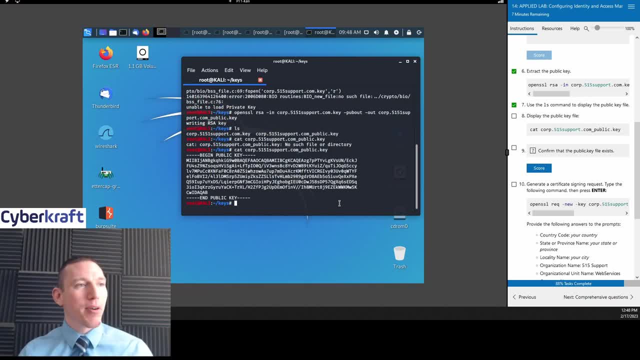 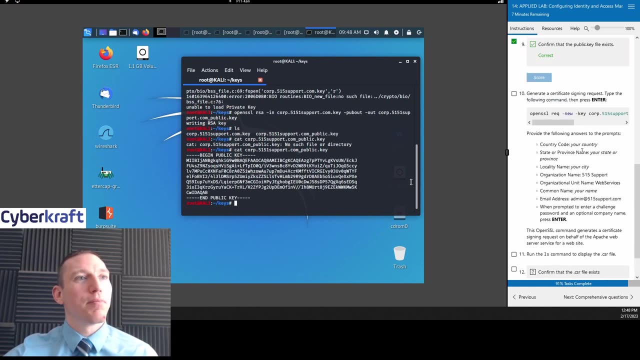 good. 51, 51 support is even better. it's nearly 10 times better. okay, so there's the public key that we see there. good, and it's gonna work. confirm that, because it's just looking for a key file and now we're gonna be generating a CSR. 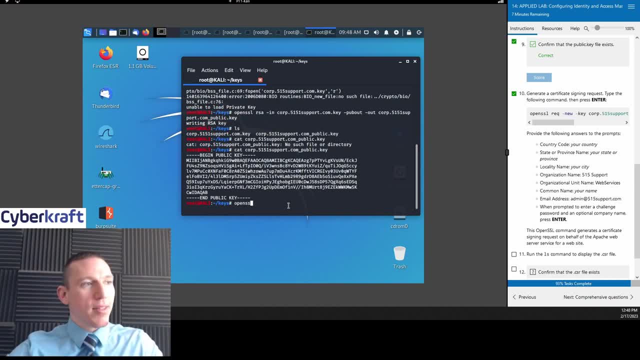 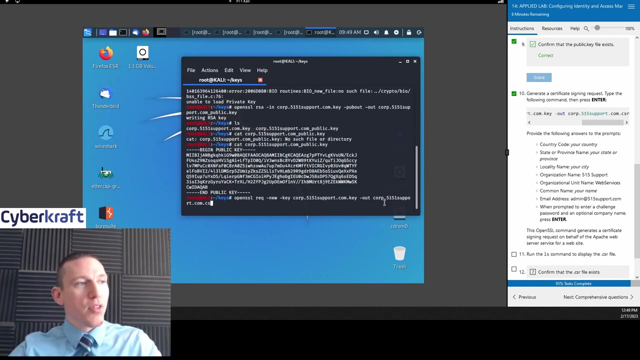 certificate signing request. okay, open SSL req request. dash new dash key corp 51 51 support calm dot key dash output corp not 51 51 support calm dot CSR. CSR stands for certificate signing request. this is request sent to a certificate authority to validate a certificate. okay, you'll be. 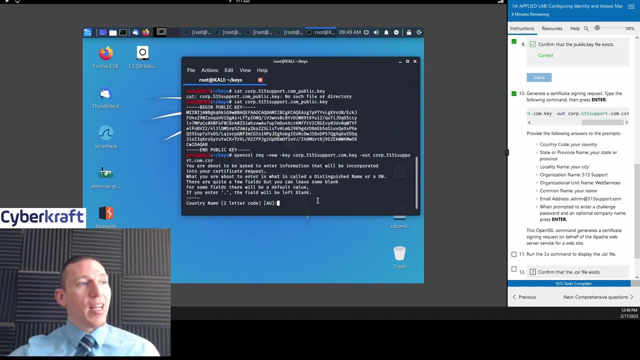 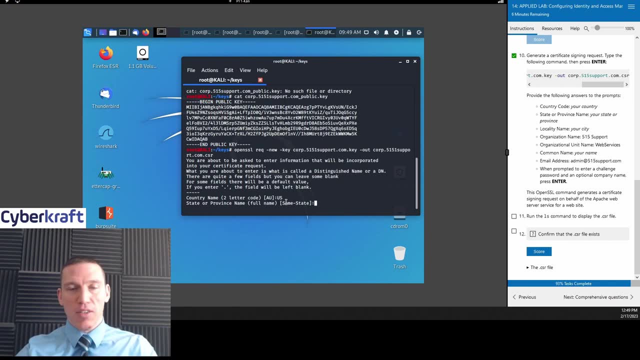 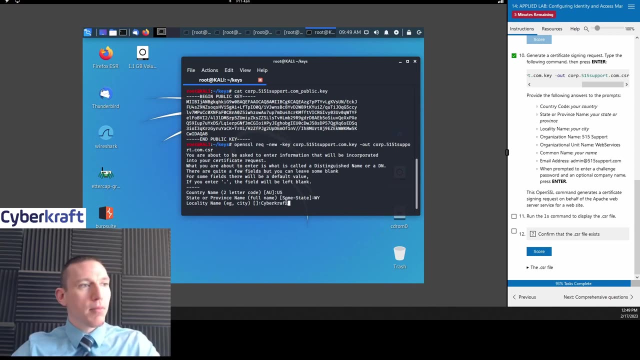 asked. you're about to be asked to enter information will be incorporated into your certificate request, okay, so now we're gonna be creating, we're gonna be inputting this information that's set up in our request here, okay, and then for it's gonna ask us to do admin at, we're gonna do admin 51, 51, support, calm the. 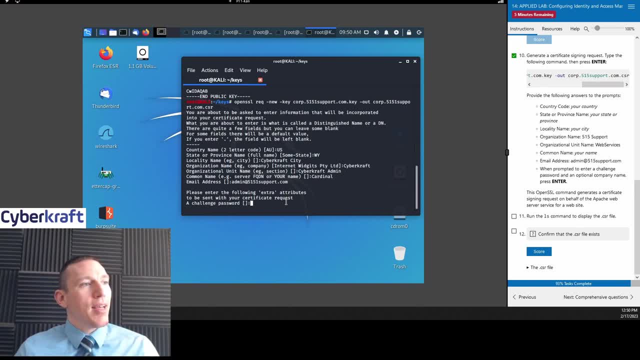 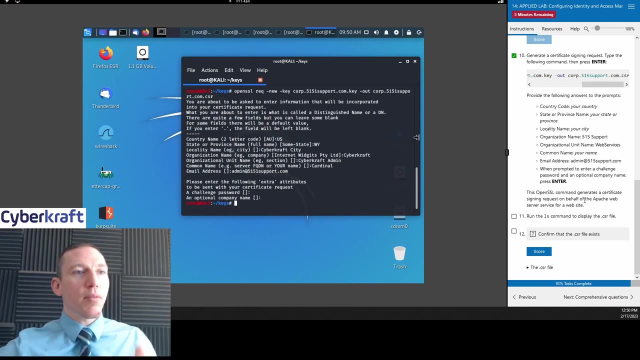 next evolution of tech support. and then please enter the following extra attributes: challenge password. now we just hit enter optional company name. we can hit enter. okay, now we have a CSR and we should be able to LS see that CSR. so we have that CSR. now we can send that CSR if we want off to a certificate. 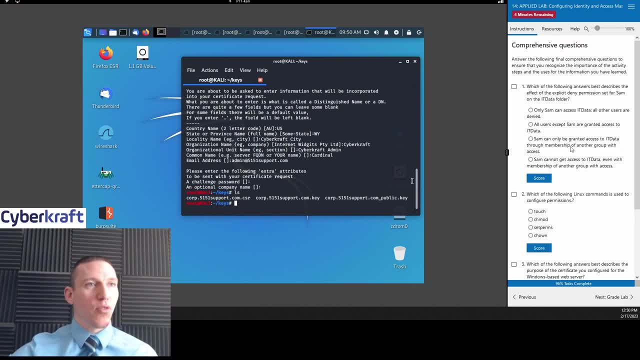 authority to validate our certificates here if we, if we really wanted to, but we don't need to do that. that's the end of the lab, alright, so let's go ahead and do our questions. you guys have any other questions before we get into these great questions today? so far, I appreciate it. 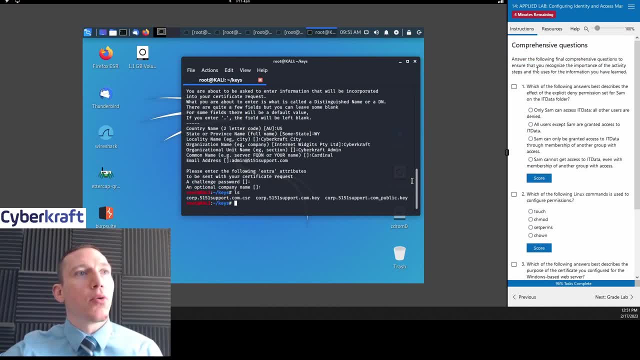 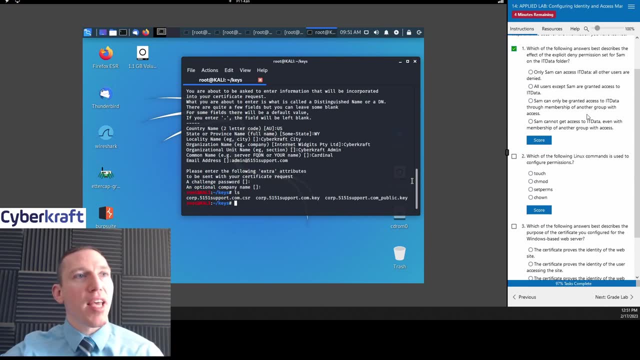 thank you so much for watching this video and I'll see you guys in the next video on the YouTube and in the in the discord. okay, which of the following answers best describes the effect of the explicit deny permission set for Sam's in the IT data folder? wow, it's going this. this lab is so involved. I could see you easily. 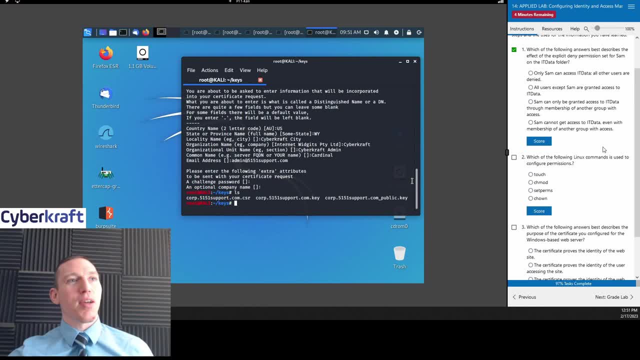 just not remembering these, okay. so which of following answers best describes the effect? remember: we create an explicit deny rule just for Sam. we're hating on Sam and the IT data folder. you- all users except Sam- are granted access to IT data. Sam cannot get access to IT. 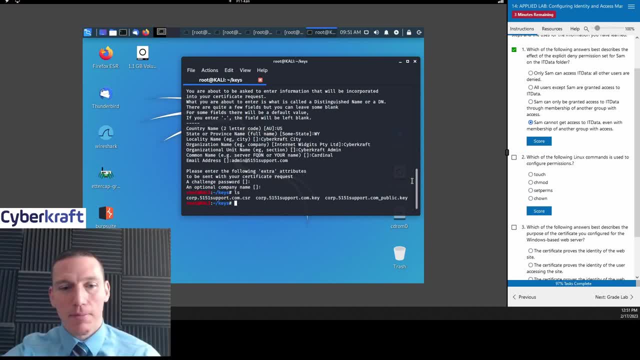 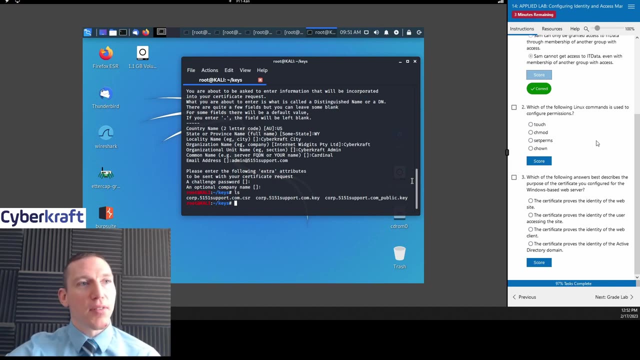 data. any ideas? yeah, Sam can. I can access to IT data even with membership of another group or access. remember, the deny rules always override the allow rules, so that's why that's correct. which of the following latest commands is used to configure permissions? well, 私gaard says I can't access it via any condition. I didn't常登. 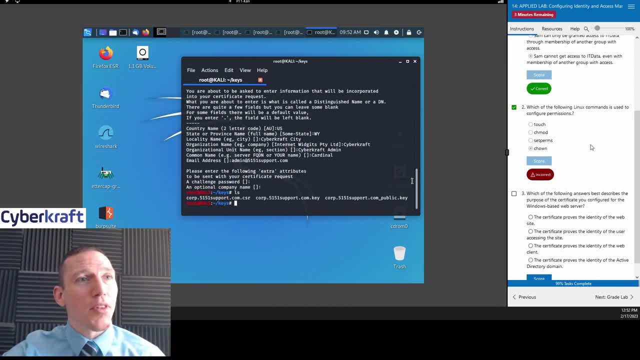 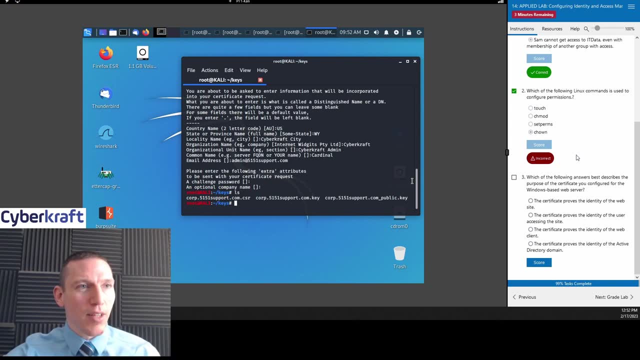 I'm sure, Sam forMontageHealthroomHealth through the app. I don't give a fuck. you can do it a couple of different ways, but cmod chmod is probably what they're looking for. you can do it through. I don't like that, kate. I don't like that. 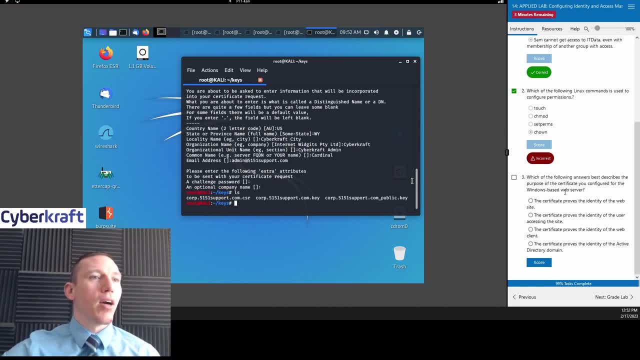 question, not just because I it's not correct, but II don't think that's an accurate way of describing that. alright, which of the following answers best describes the purpose of the certificate you configure for the windows-based web server? certificate proves the identity of the website. the certificate proves the identity of the user. 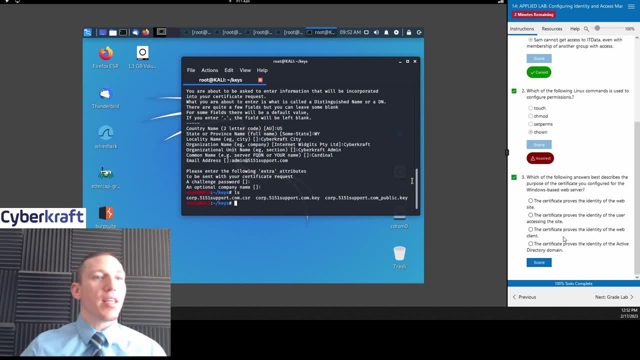 accessing the site. certificate proves the identity of the web's client or the web, and the certificate proves the identity of the active directory domain, or what do you guys think the answer is here: a, b, c or d. i'll just this: will be a, b, c or d.